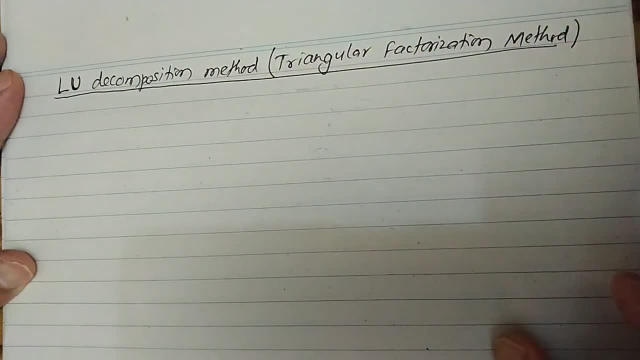 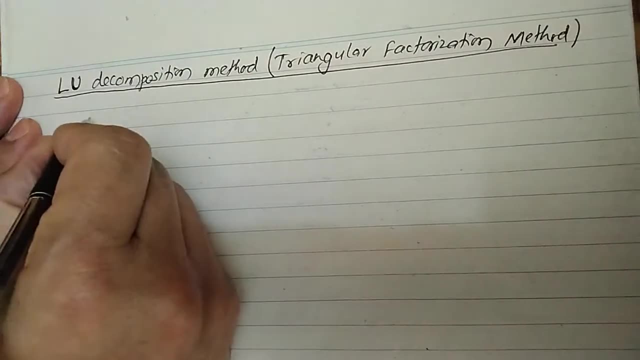 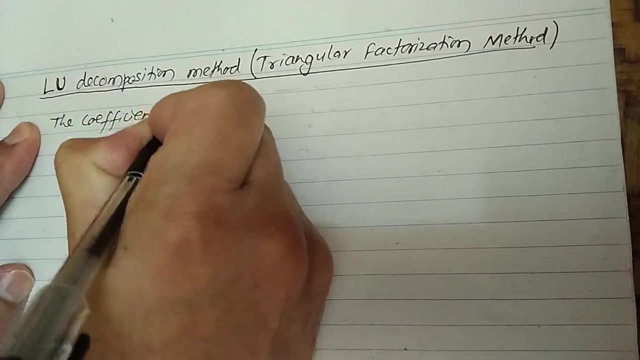 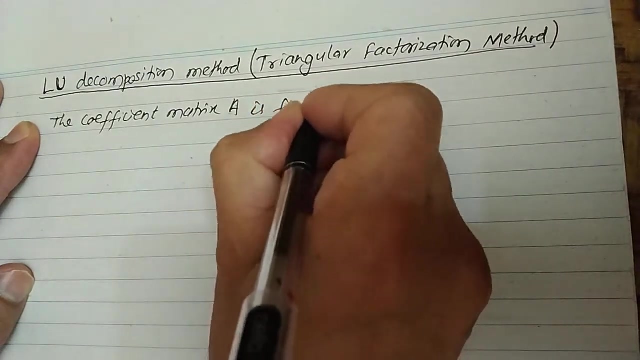 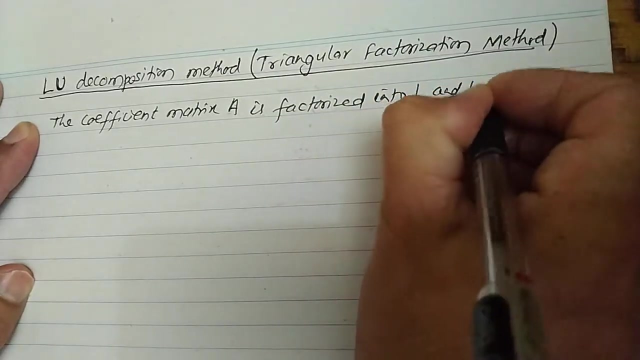 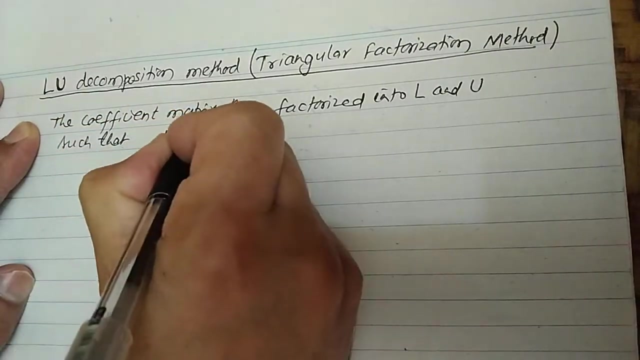 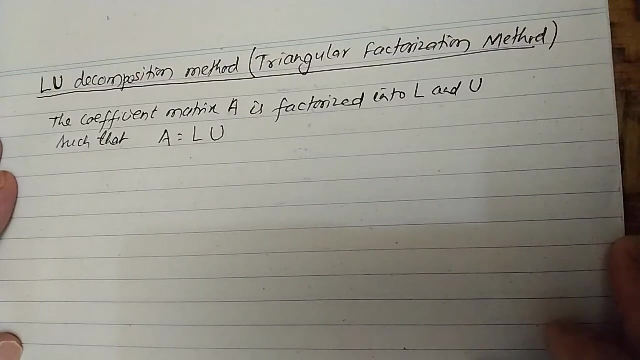 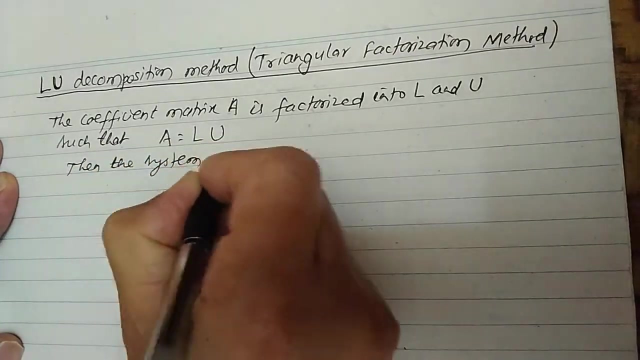 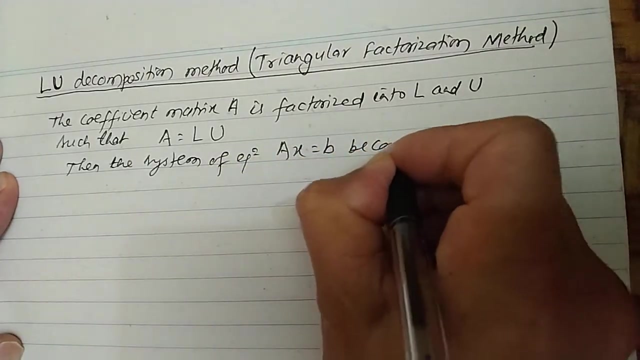 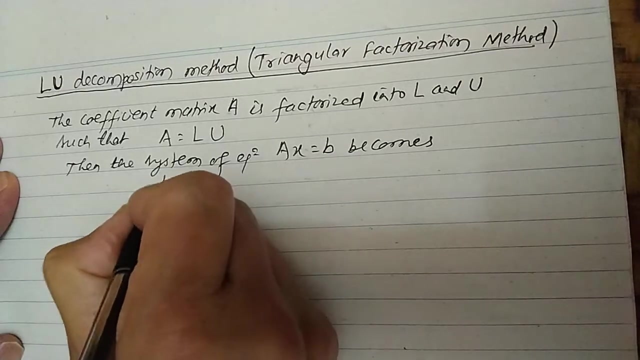 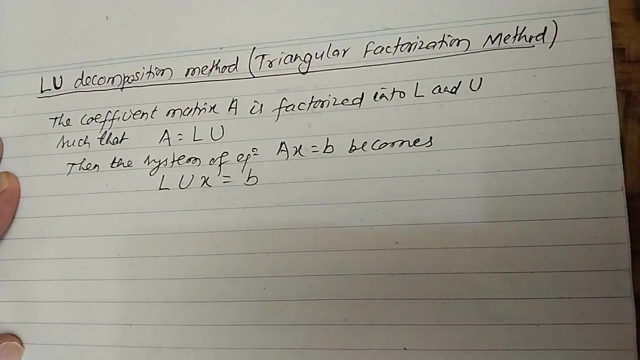 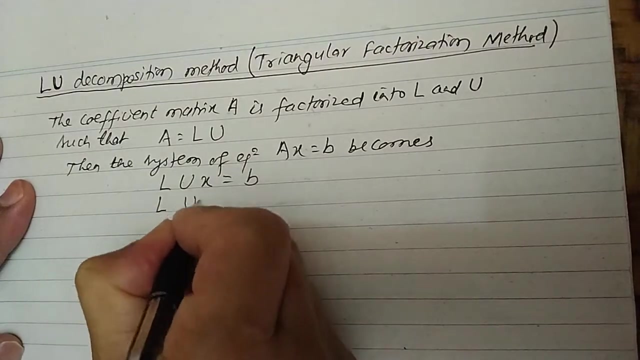 In this method the coefficient matrix A is factorized into L and U, such that A will be equal to the product of L and U. Then the given system of equation, AX equals to B, becomes SUBSTITUTION B, where Man and Vx L into UX equal to 7. 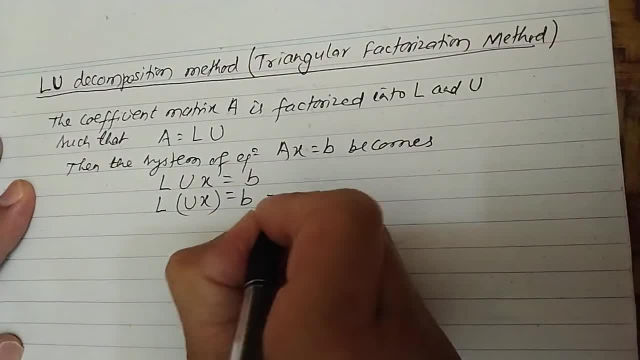 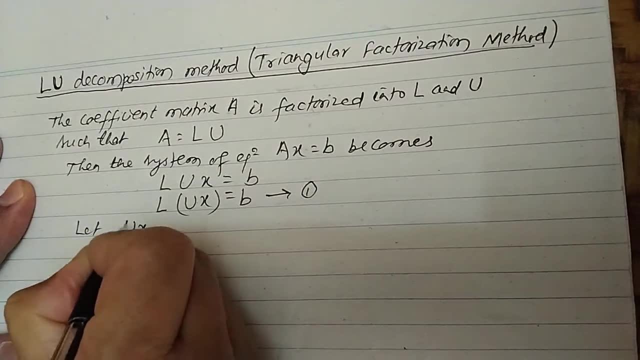 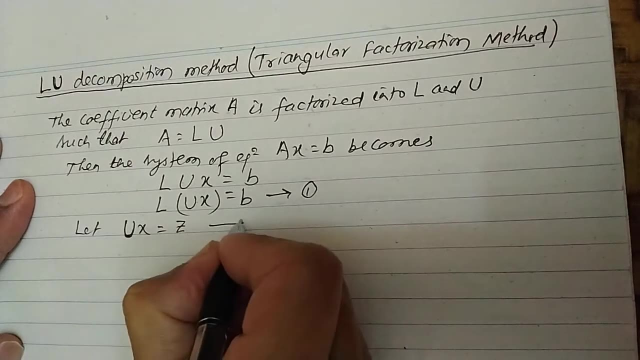 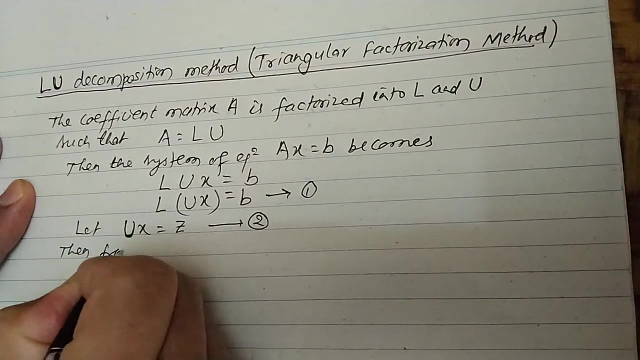 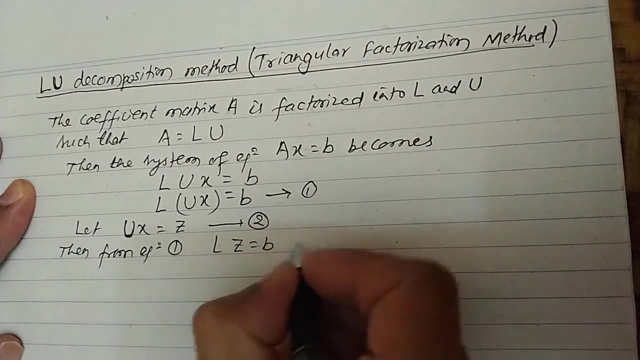 So what shall we substitute in the equation A? So let ux u into x equals to z, where z is an unknown vector. If you suppose this, then equation 1 becomes l into z equals to b. This is equation number 3.. 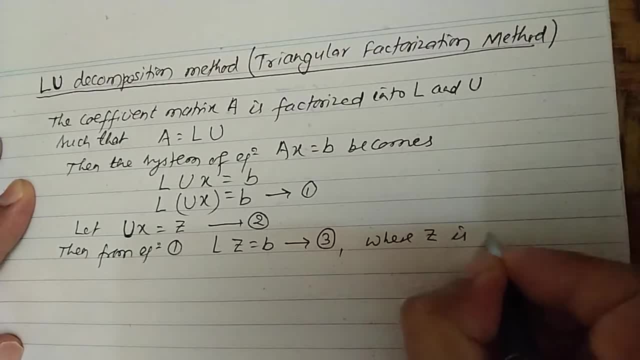 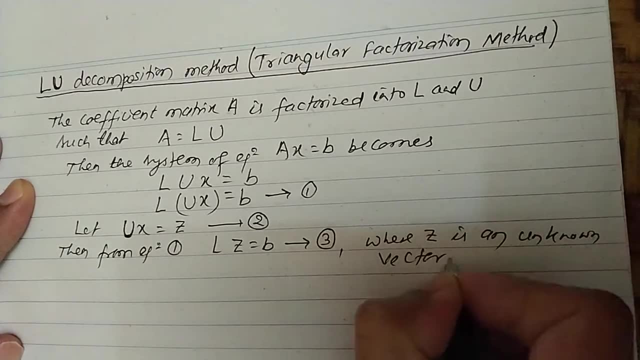 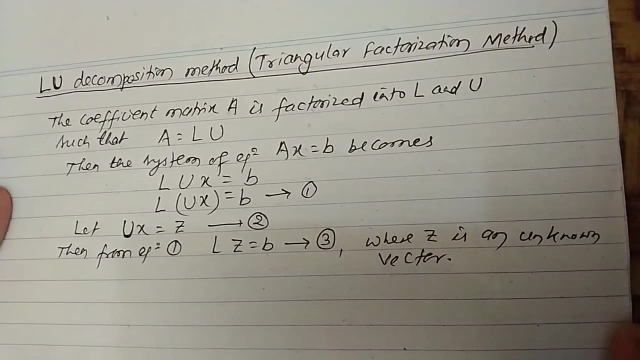 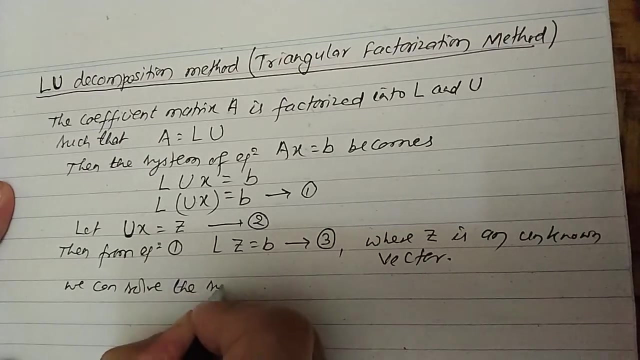 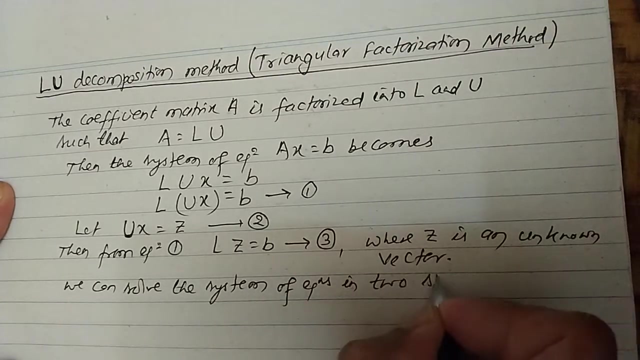 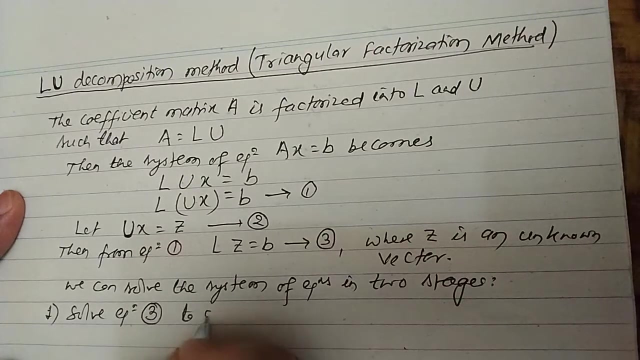 Where z is an unknown vector. Where z is an unknown vector, We can solve the system of equations in two stages. So we can solve The system of equations in two stages. So first stage, Solve equation 3 to get the value of z. 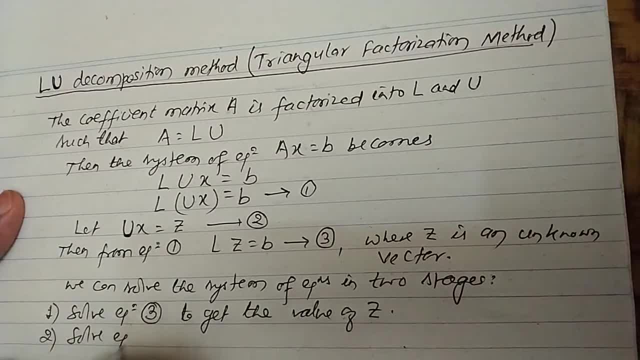 If we can solve this, then the problem will be solved in the next stage. Now we can use it in the resultant solution. Can't solve equation 1.. Followed by this one, Solve the equation 2, to get x into g. 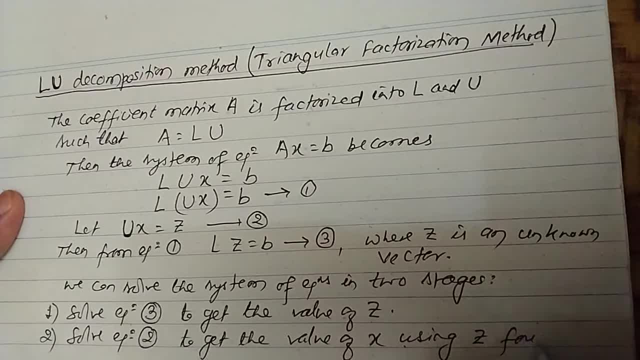 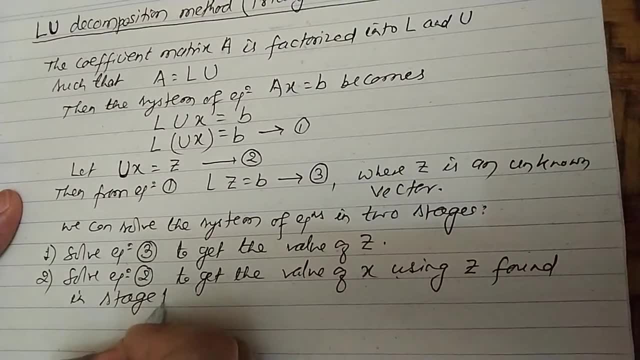 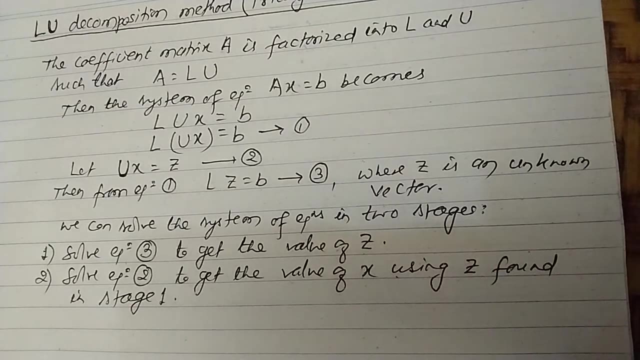 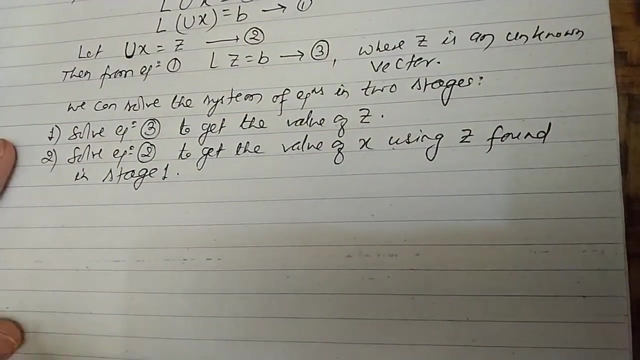 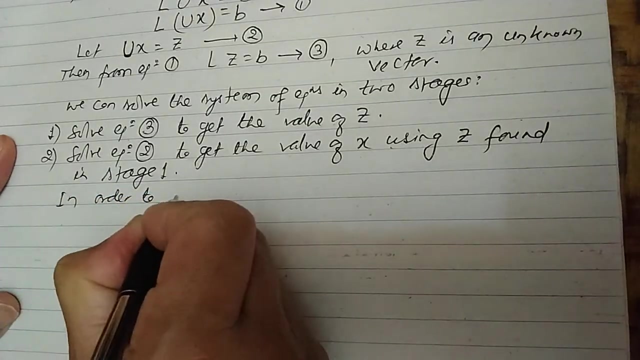 Solve equation 2 to get x into g. Solve equation 1 into x. Ask for solution 1. Here, ask for solution the two Easy problem. oh so we can do this in two stages. so, in order to produce, in order to produce. 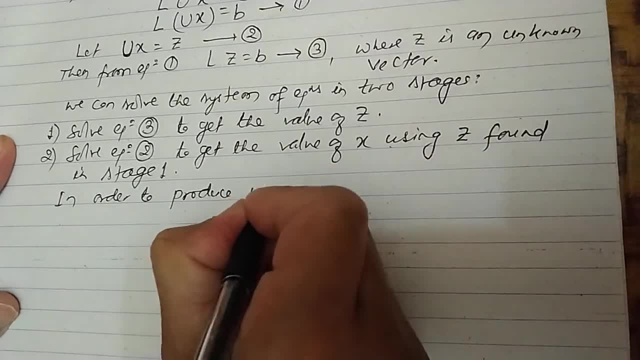 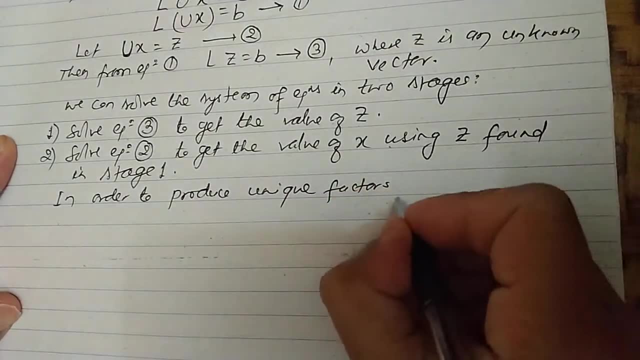 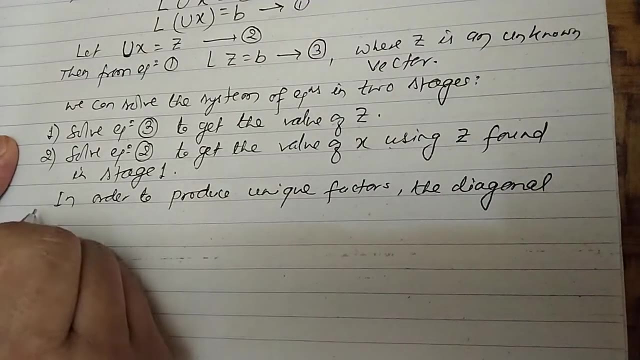 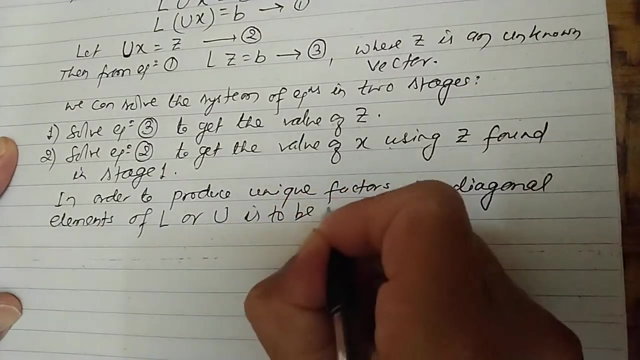 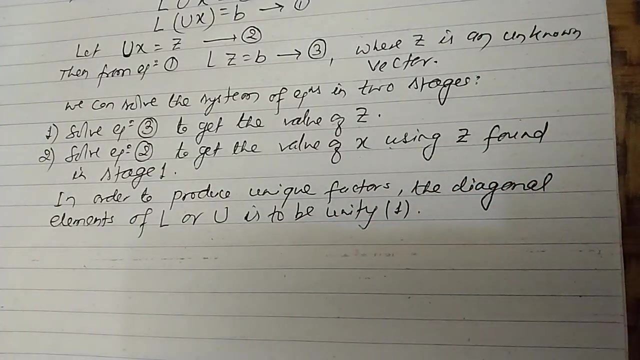 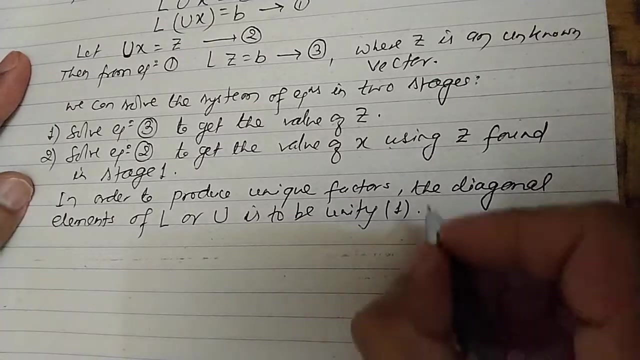 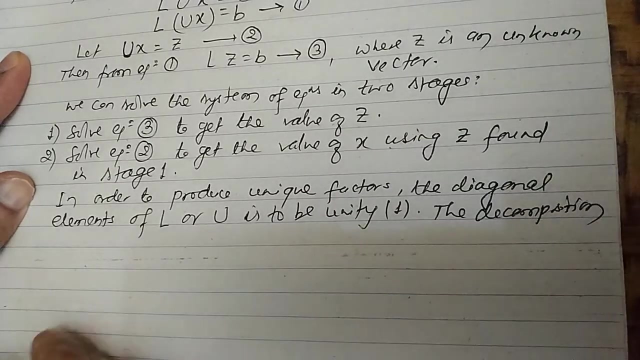 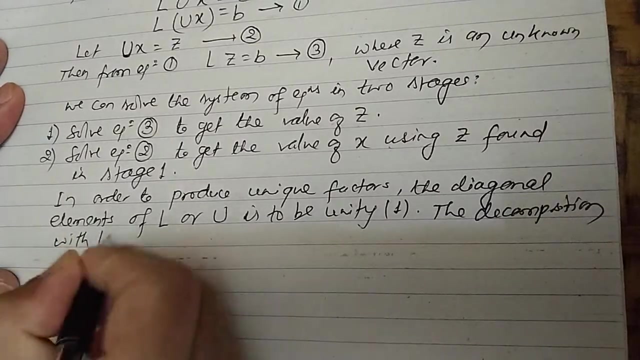 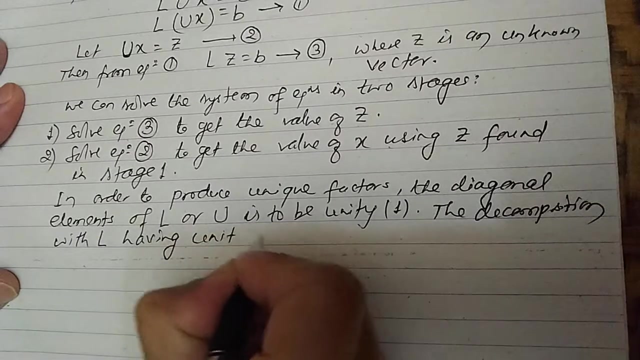 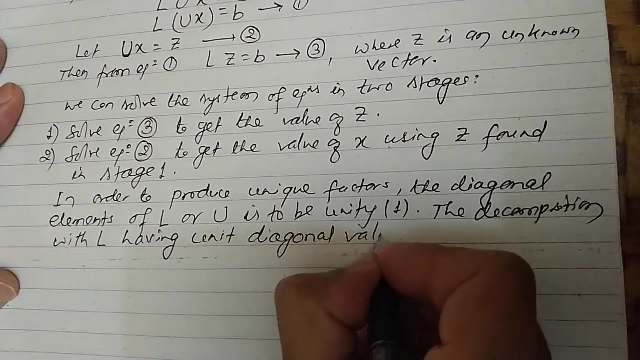 unique factors: unique factors in order to produce unique factors. the diagonal element, the diagonal elements of y'all or you, you is to be unity. when I go one person, the diagonal elements of either L or you should be unity. the decomposition with L having unit diagonal values is called. 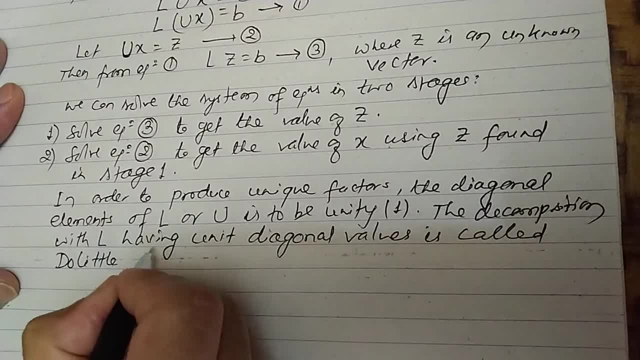 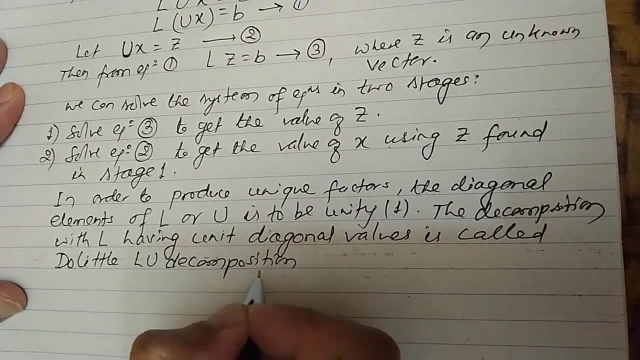 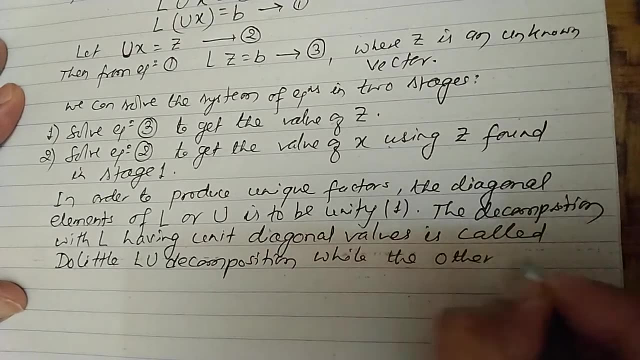 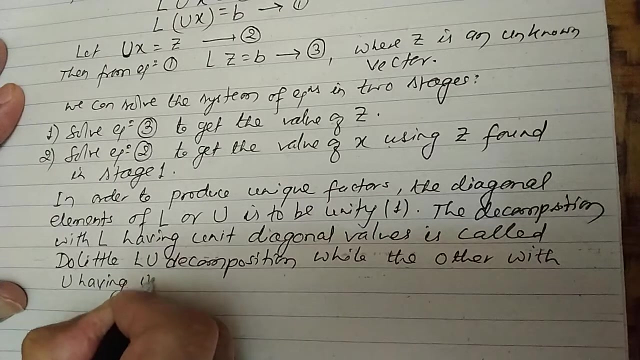 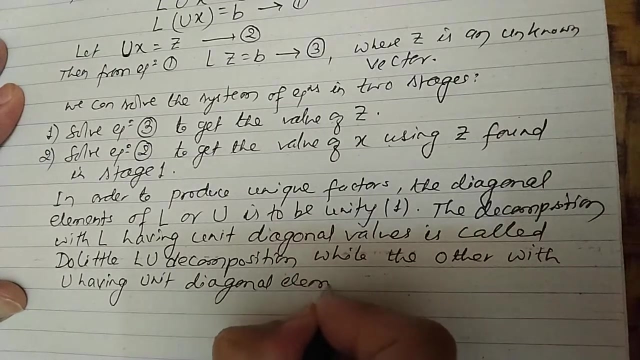 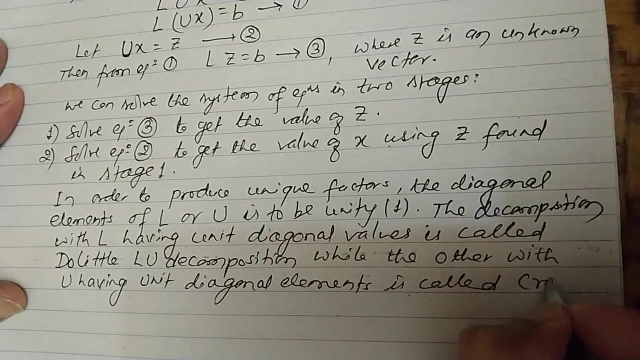 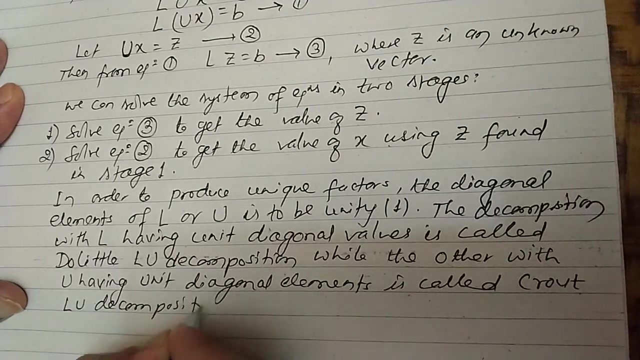 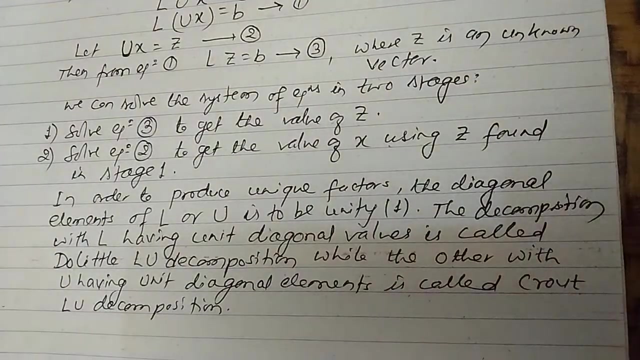 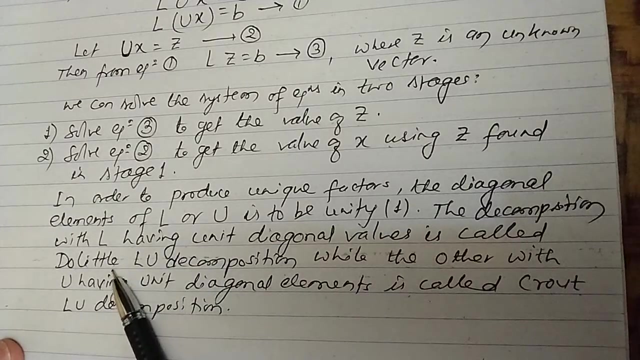 do��이야 alú decomposition is called � . While the other with U having unit diagonal elements is called cropped. So, if you take the diagonal elements of L to be unity 1, so that is called Doolittle LU decomposition or Doolittle algorithm. If you take the diagonal element of U to be 1, 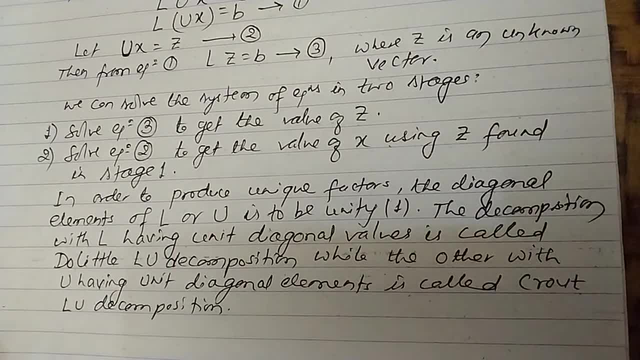 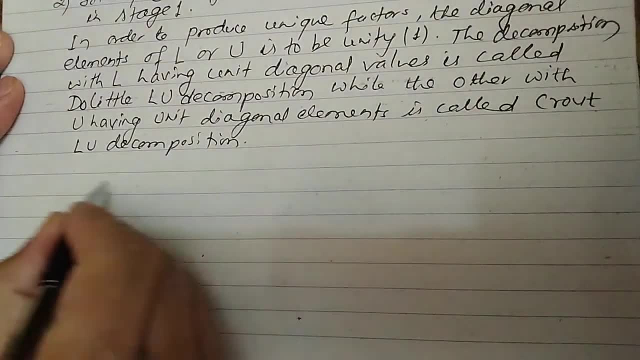 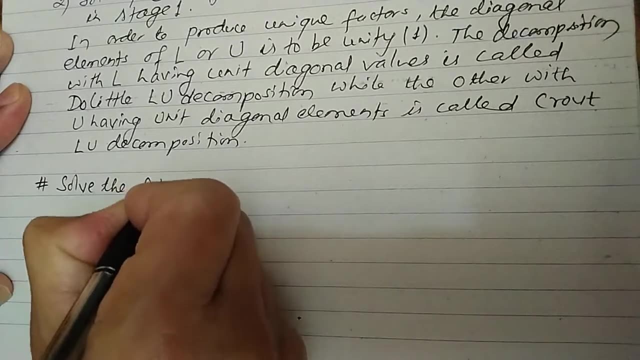 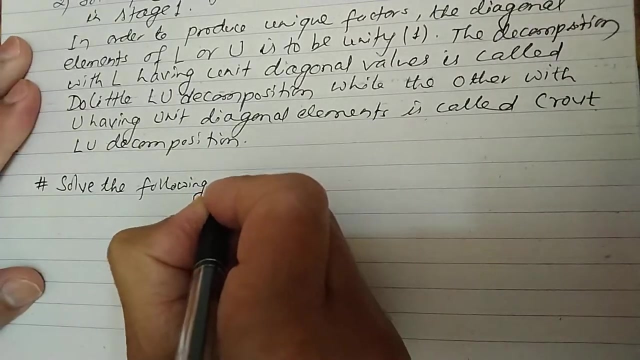 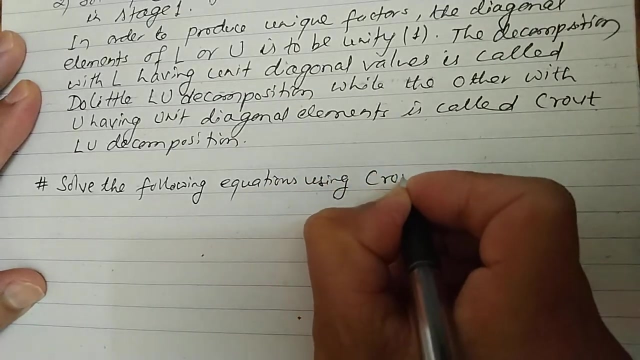 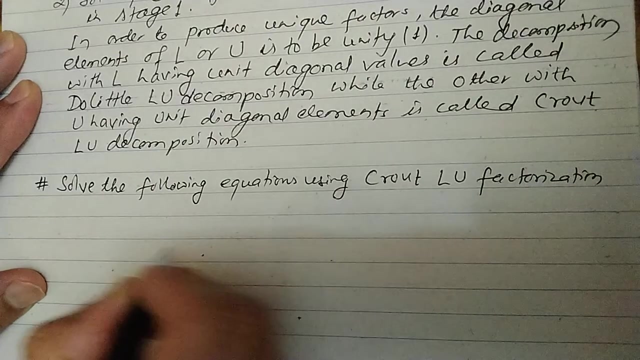 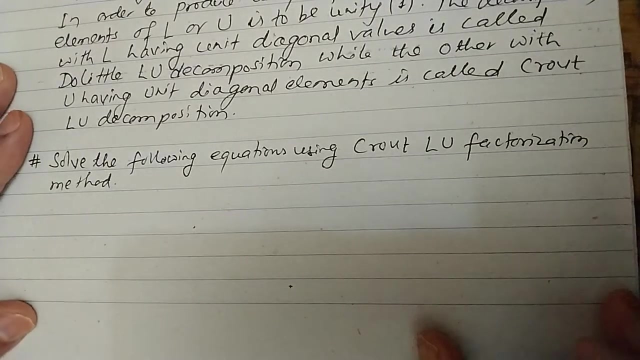 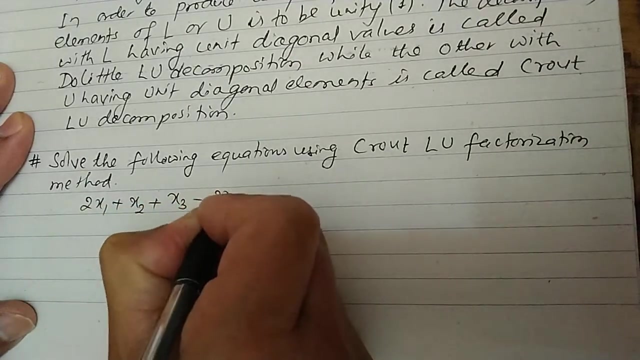 that is called Crout LU decomposition. So write down a problem. Solve the following equations: Crout LU factorization method. So you solve these equations by using LU factorization methods. The equations are: 2x1 plus x2 plus x3 minus 2x4. hoor, equals to 0.. 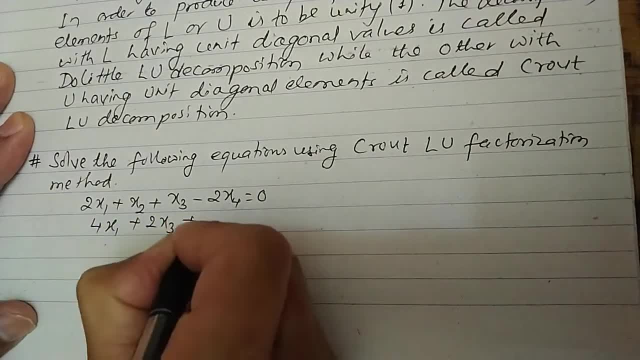 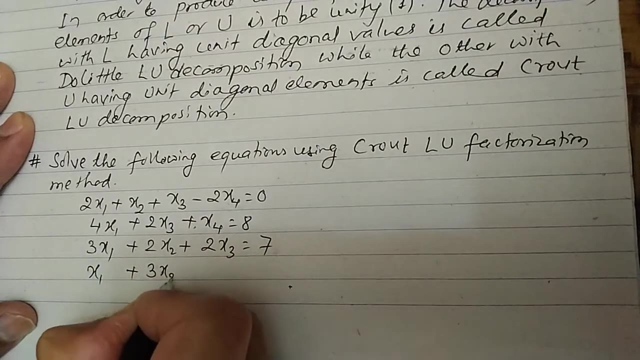 4x1 plus 2x3 plus x2. x4 equals to 8, 3x1 plus 2x2 plus 2x3 equals to 7, x1 plus 3x2 plus 2x3 equals to 3.. 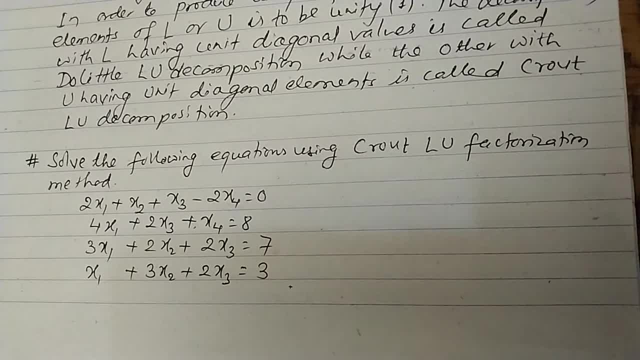 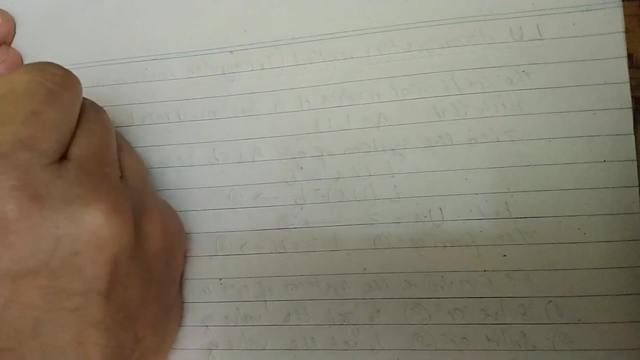 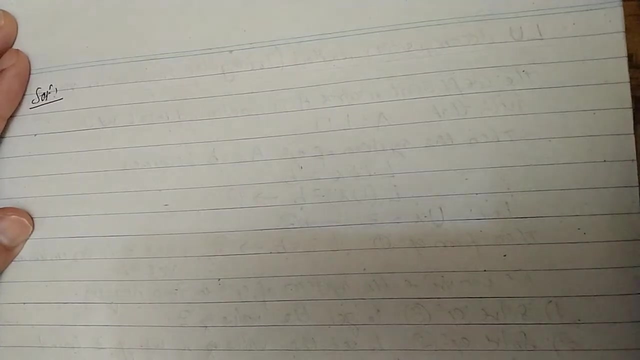 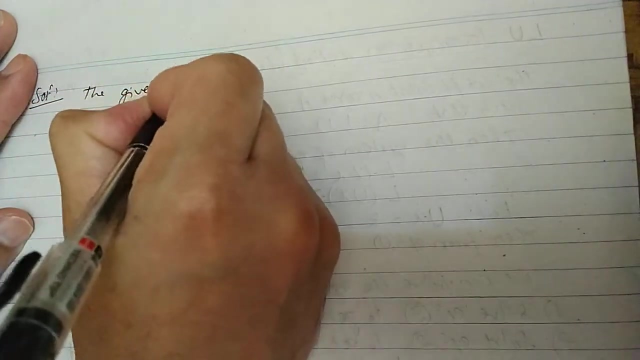 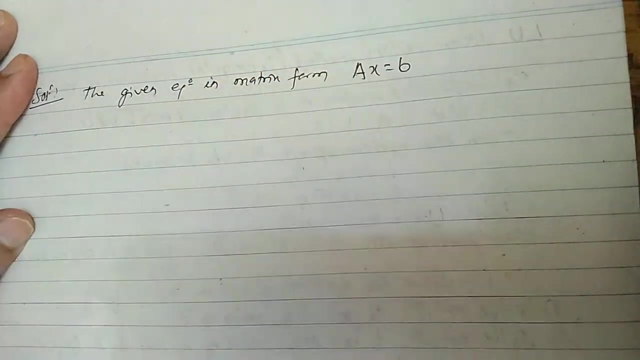 So let us do the solution. So write down: Ax equals to b. So let us write down the form of the given equation in matrix form: Ax equals to b. Alright, So write down the value of a. Okay, Keshav. 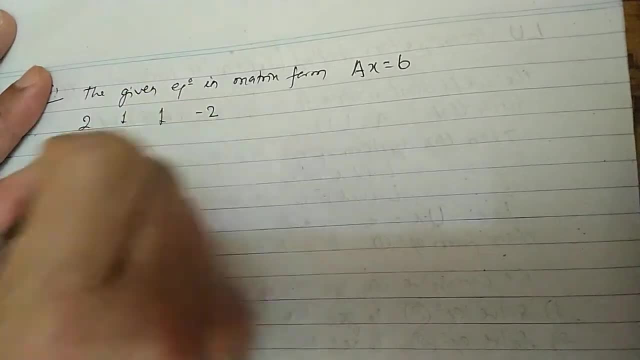 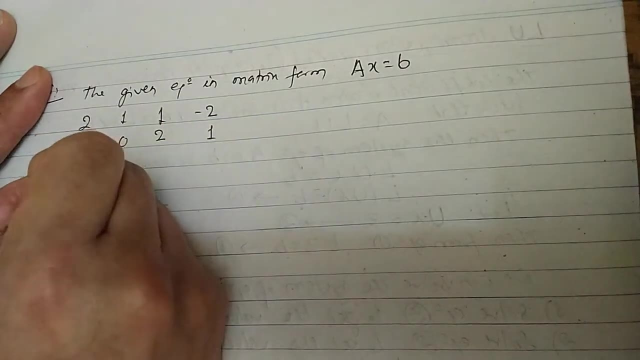 2, 1, 1, minus 2, 4, 0, 2, 1.. 3, 2, 2, 0, 1, 3, 2, 0.. This is a 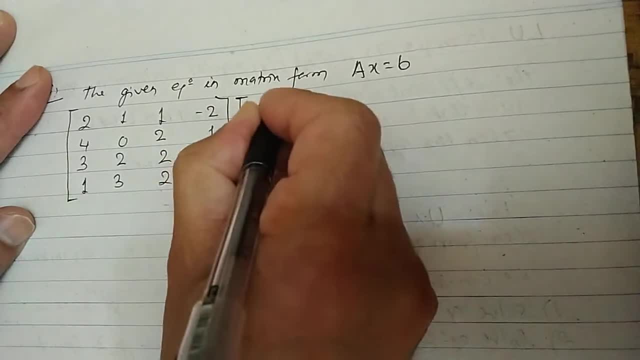 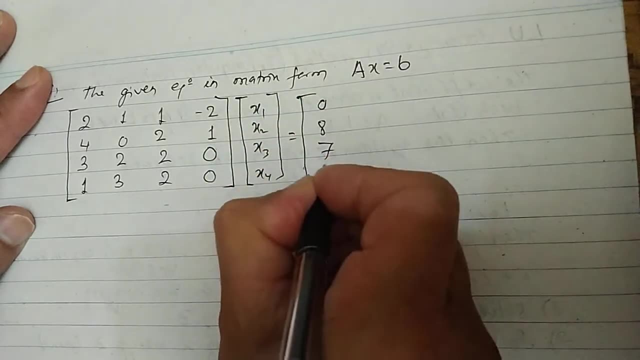 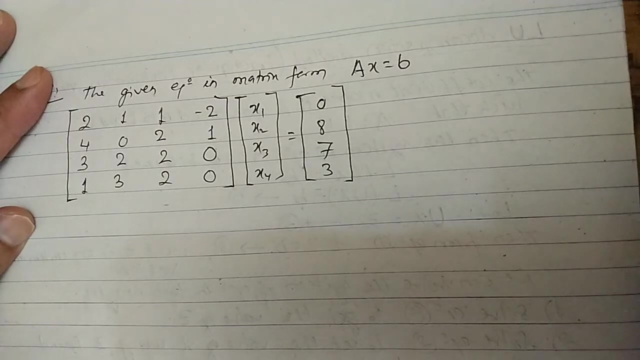 x1, x2,, x3, x4.. This is x, And what is right hand side vector 0, 8.. So 0, 8, 7. 3. Got it? So let us factorize. 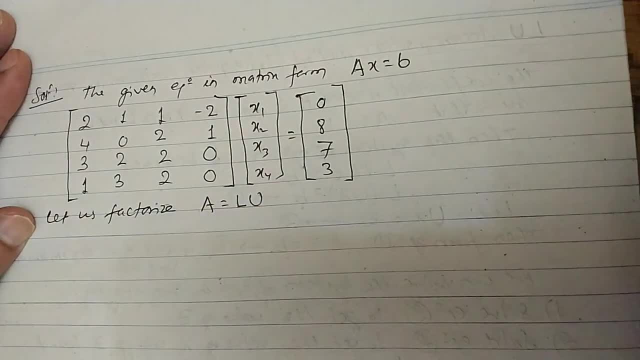 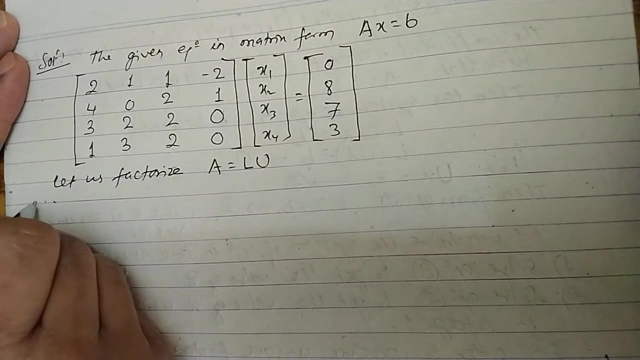 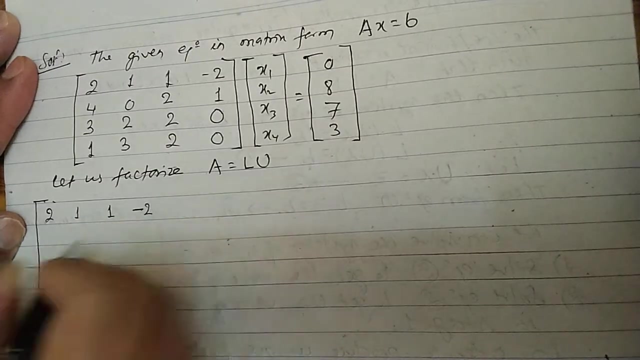 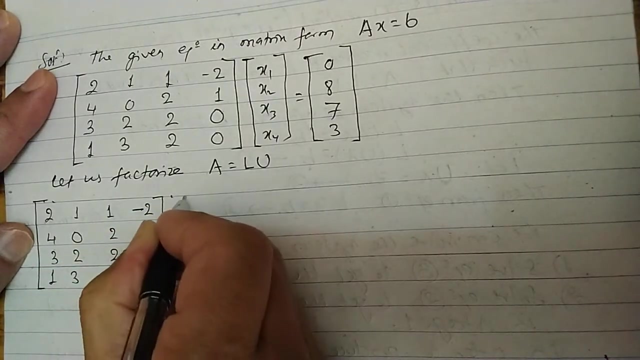 a equals to l? u. Alright, Let us factorize the coefficient matrix a into l and u, such that a? equals to l? u. Okay, So write down the value of a here: 2, 1, 1, minus 2, 4, 0, 2, 1, 3, 2, 2, 0, 1, 3, 2, 0, this is A equals to. now let us write: 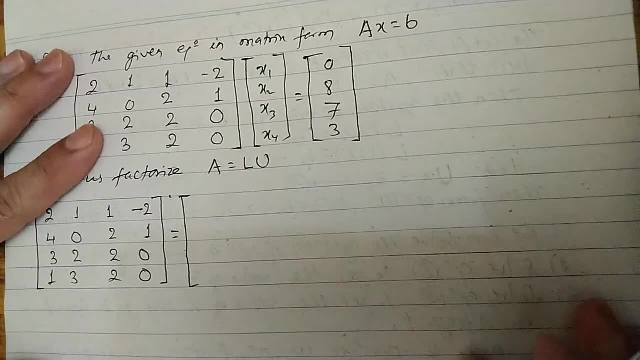 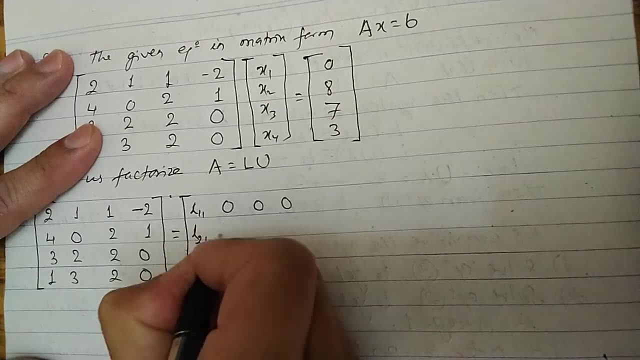 down the value of L and U: L1, 1, 0, 0, 0, L2, 1, L2, 2, 0, 0, L3, 1, L3, 2, L3, 3, 0,. 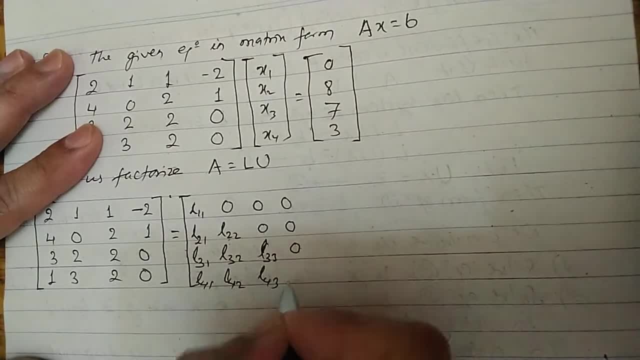 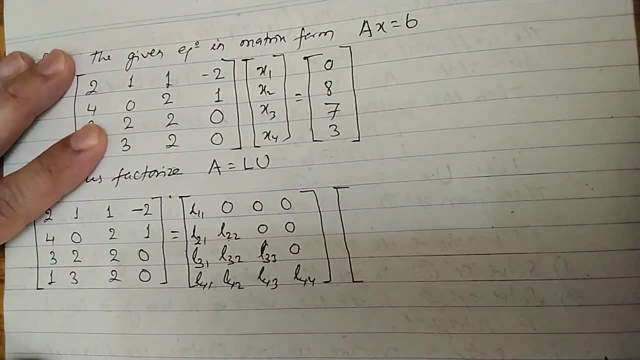 L4, 1, L4, 2, L4, 3, L4, 4,. alright, this is L Wow. Now let us write U. When we write U, the diagonal elements of U must be 1, because we have to use. 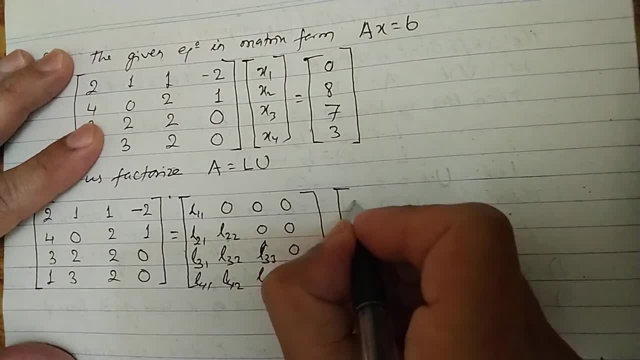 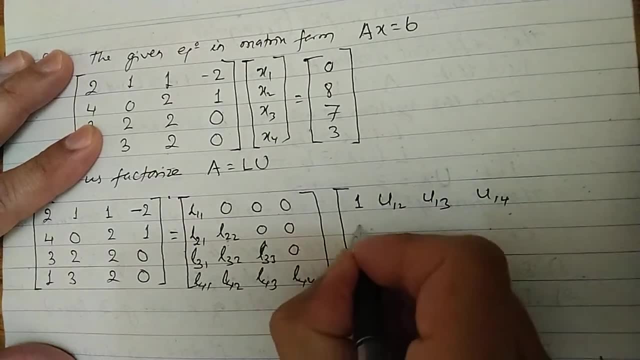 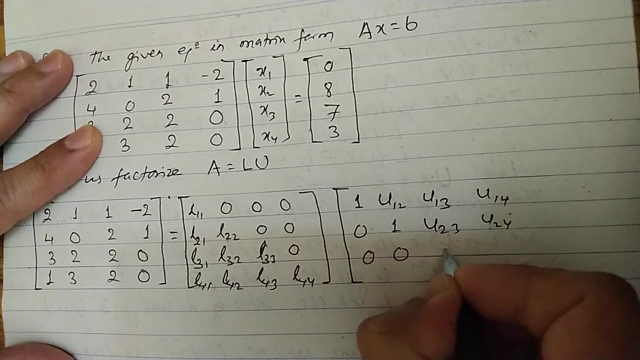 the Kraut algorithm. So to have the diagonal element of U1, the initial element of U is U12, U13, U14, 0, 1, U23, U24, 0, 0, 1, U34, 0, 0, 0, 1, alright. 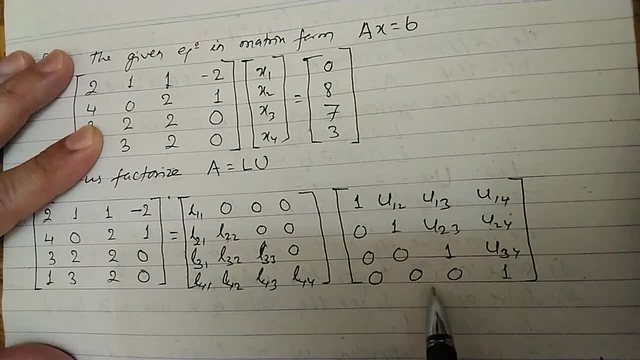 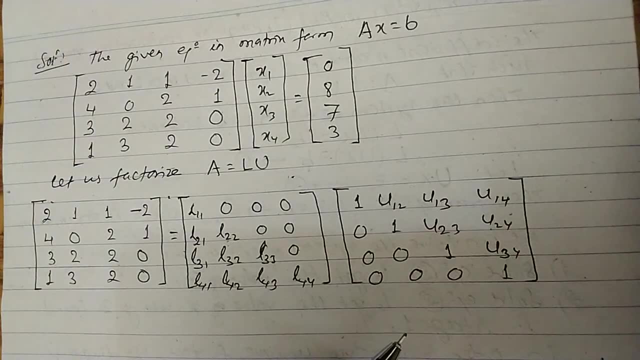 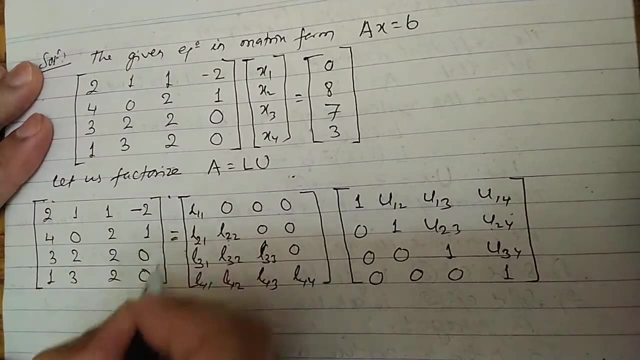 So this is a lower triangular matrix, this is an upper triangular matrix. We take the diagonal element of upper triangular matrix to be 1 because it is an Kraut algorithm or a Kraut-LU decomposition. Alright, so I will be using is equal to sign here, So multiply these two now. 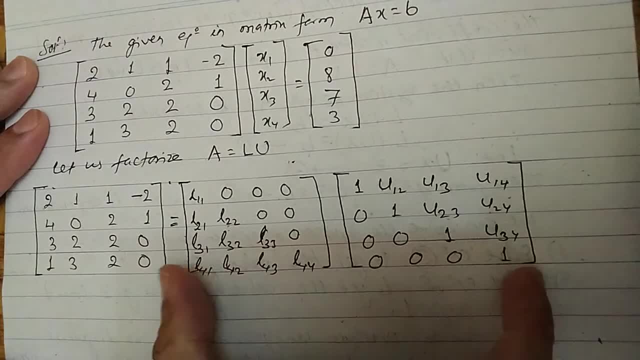 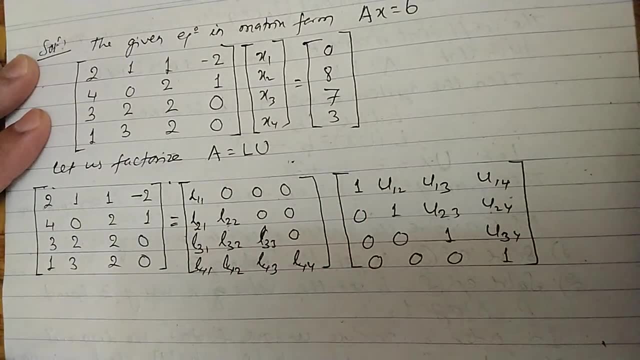 You have got a 4 into 4 matrix or 4 into 4 matrix. So multiply these two, you will get one 4 into 4 matrix. Compare the coefficient, Then you can get the value of L and U. Okay, so I will take an is equal to here. 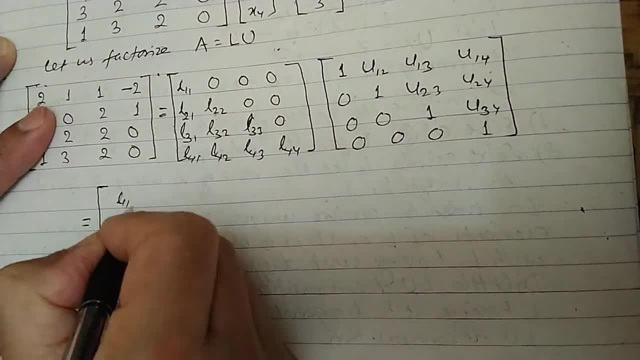 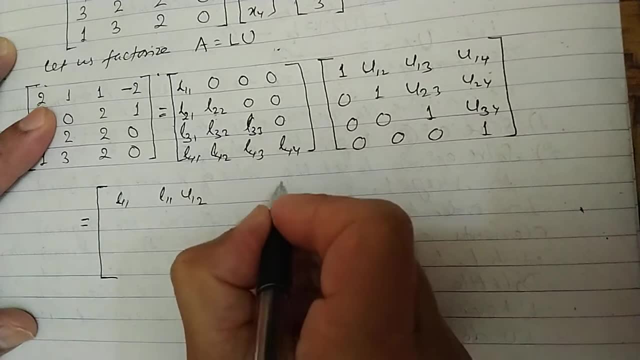 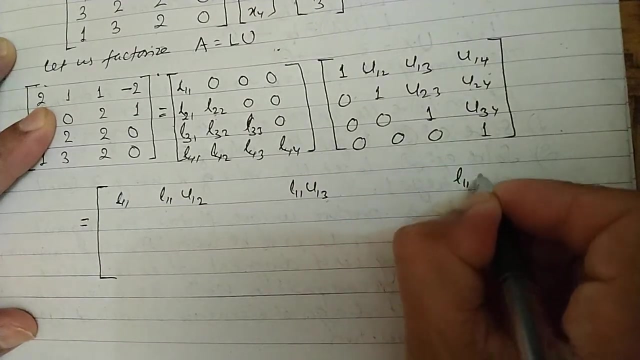 So let us multiply. Now, what is the lower element? It is L11.. L11, U12.. L11, U13.. L11, U14.. Keep these spaces, Let us multiply. It is not required in the beginning, but we can do it later. 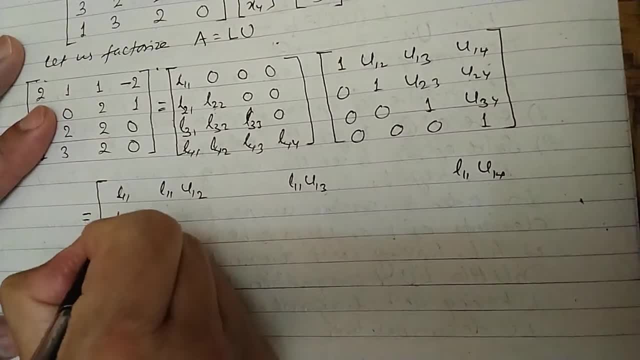 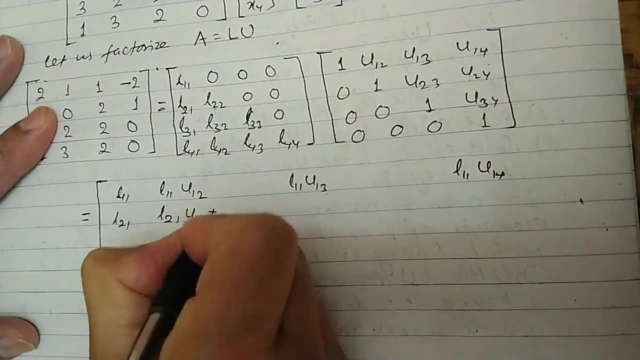 Keep these spaces, So L21.. What else is there? L21.. Multiply it L21 into U12 plus L22. And L21, U13 plus L22.. What else? L21, U14.. L21, U14. 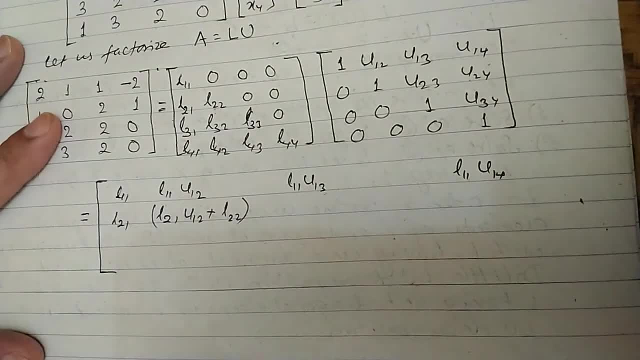 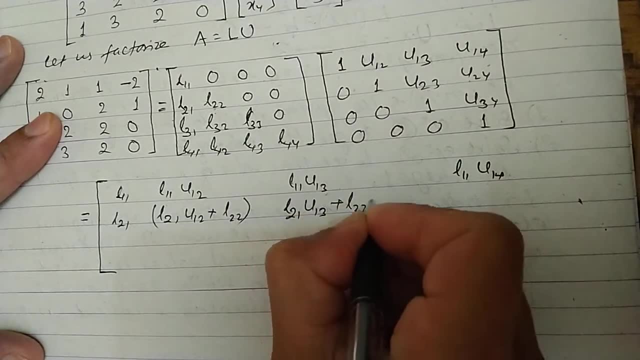 L21 U14.. What else? L21 U14.. 1. L21 U14.. 1. L21 U14 plus L22 U3.. 1. What else? 1. L21 U14 plus L22 U3.. 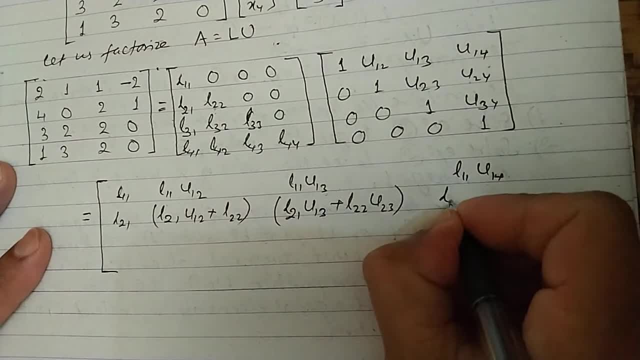 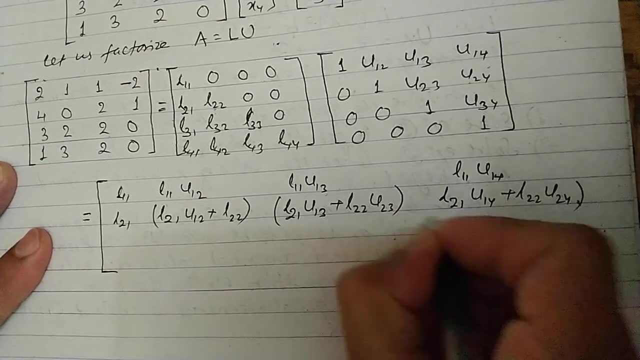 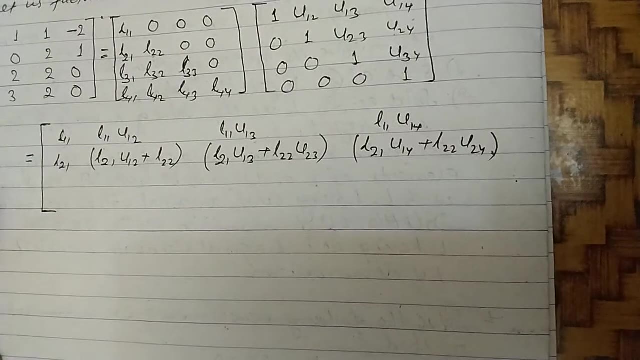 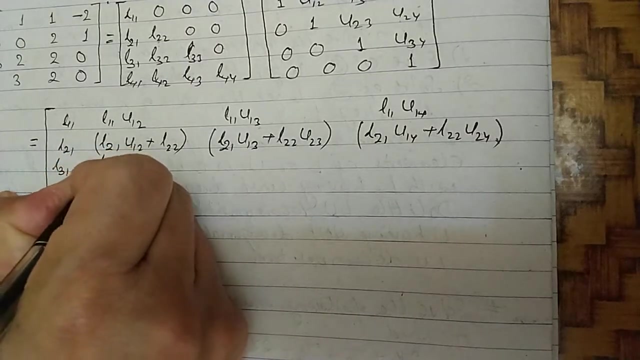 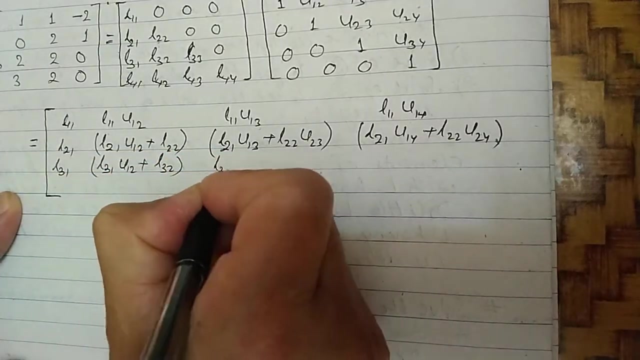 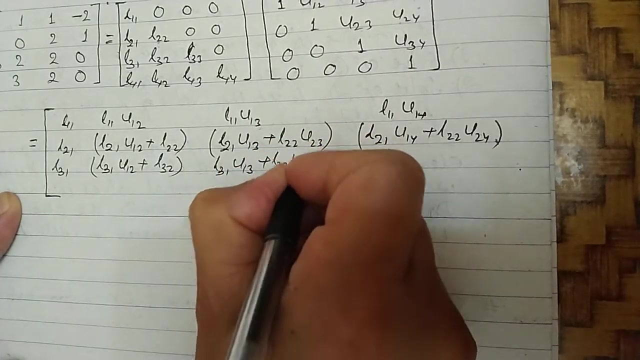 1. To do the same. we should also do it by do a row into column. Okay, so do the same. 2. L21- U14 plus L22- U24.. 1. or go down: l31- l31- u12 plus l32, l31- u13 plus l32, u23 plus l33. 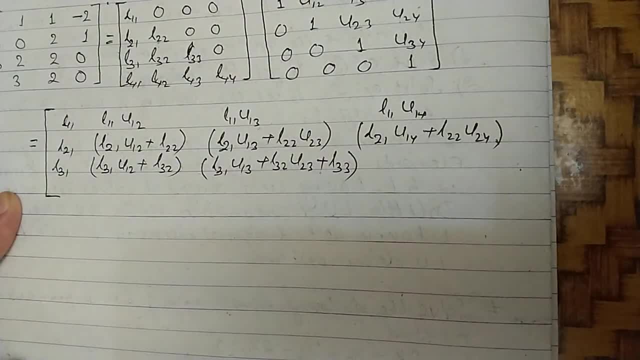 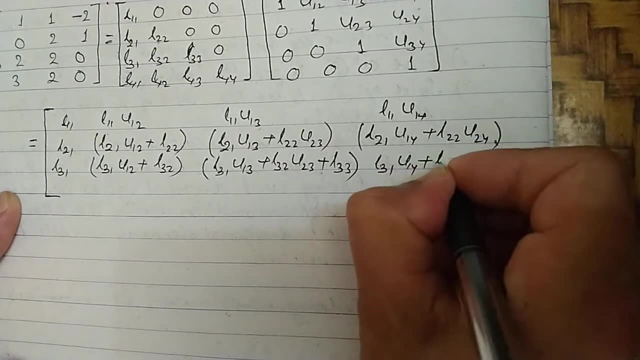 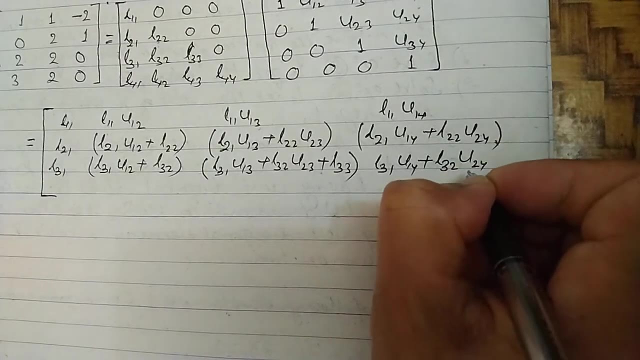 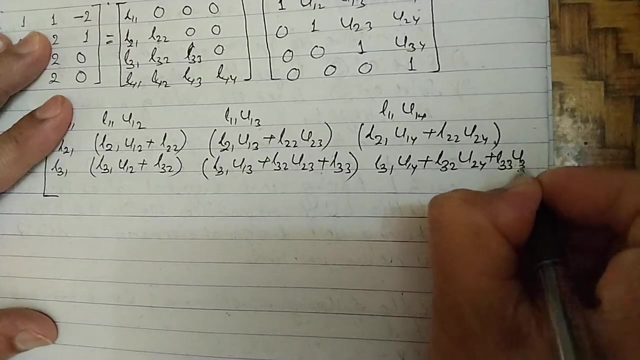 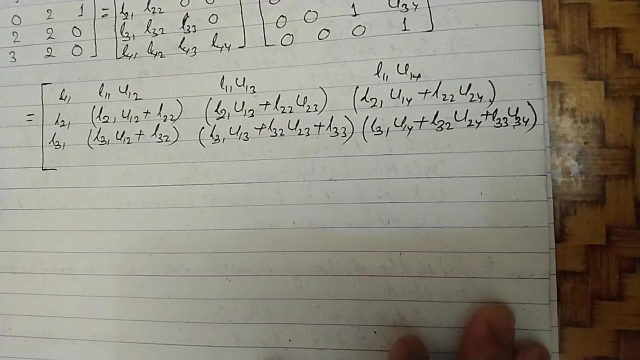 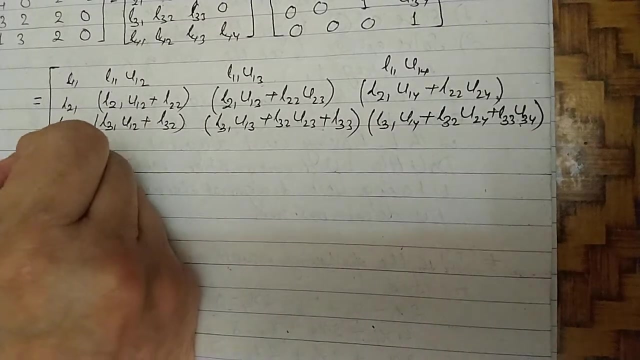 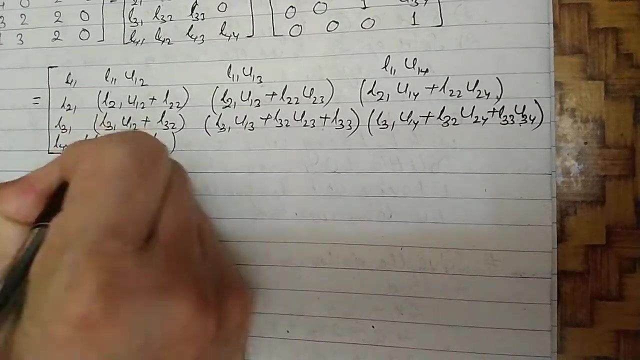 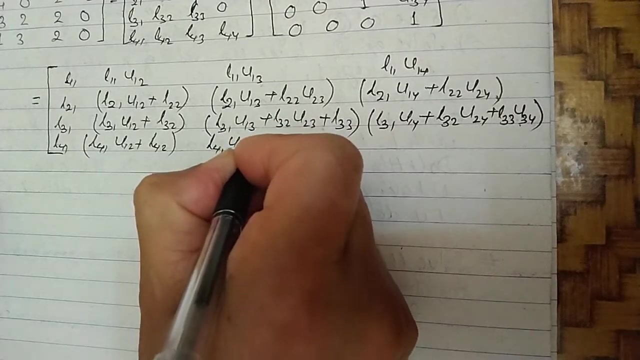 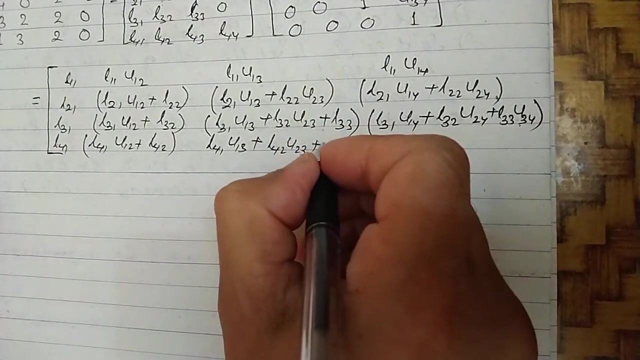 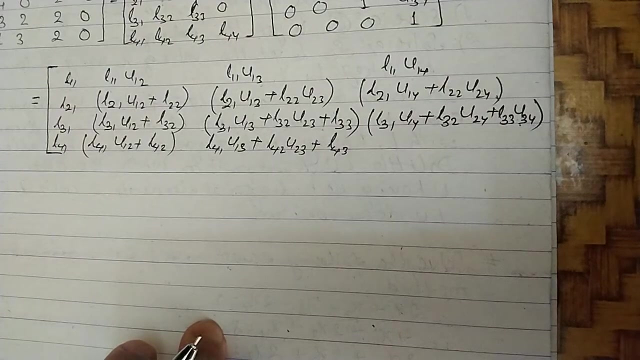 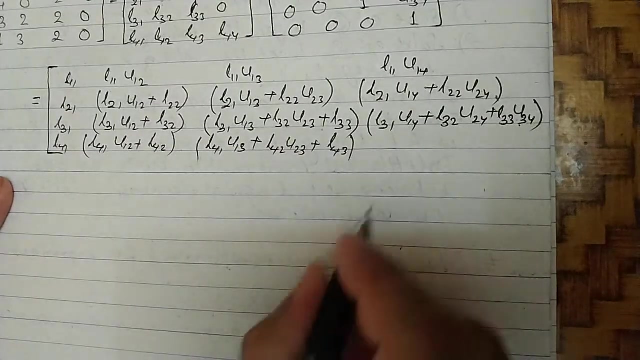 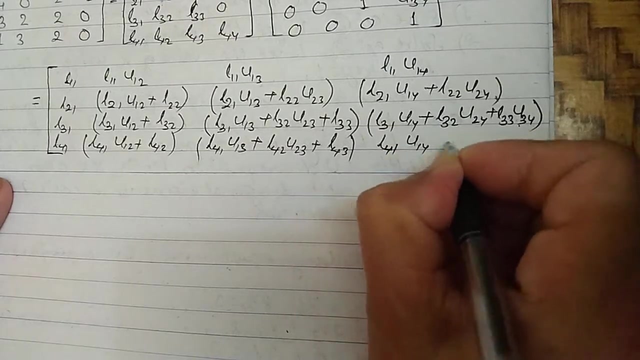 the next one: l31. u14 plus l32. u24 plus l33, u34 by l41. l41 into u12 plus l42. l41 into u13 plus l42 into u23 plus l43. the next one: l41 into u14 plus l42 into u24. 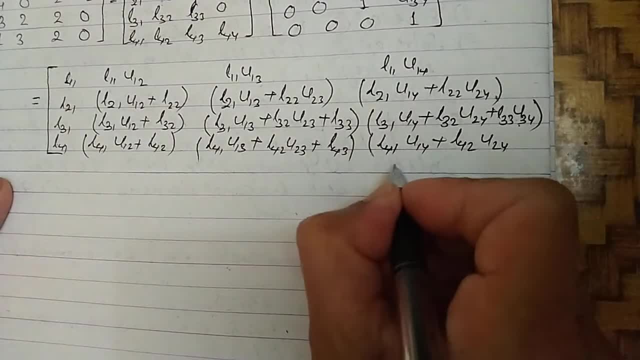 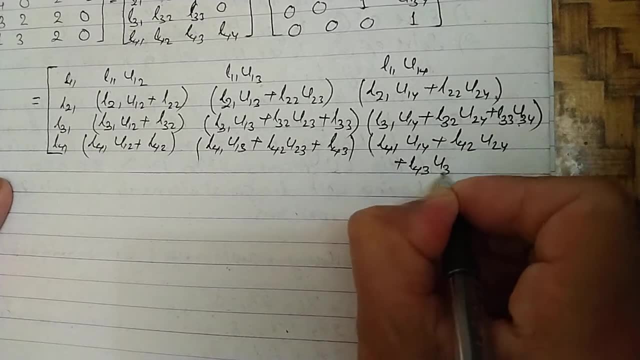 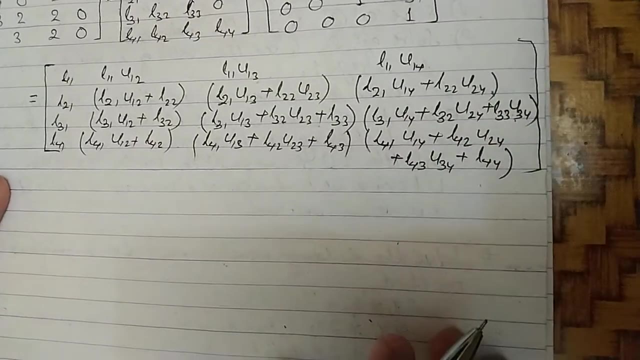 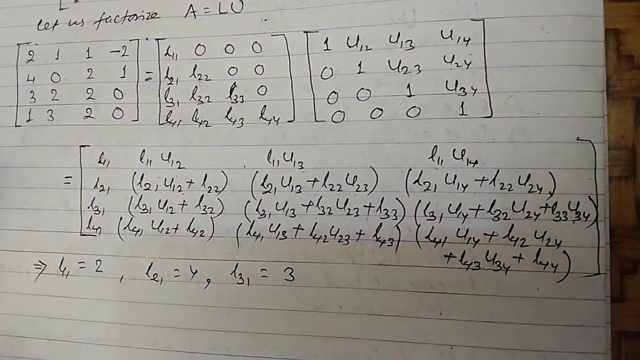 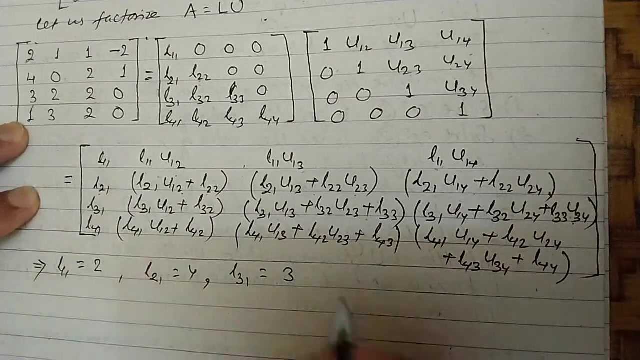 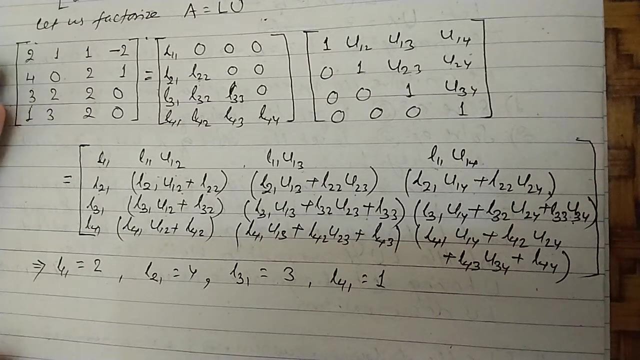 plus l43 into u14, l43 into u34 plus l44. so write down the coefficients by comparing with the equality. so l31 will be equals to 3, l41 will be equals to 1, l31 into u13. again let's compare some to make two ceres. 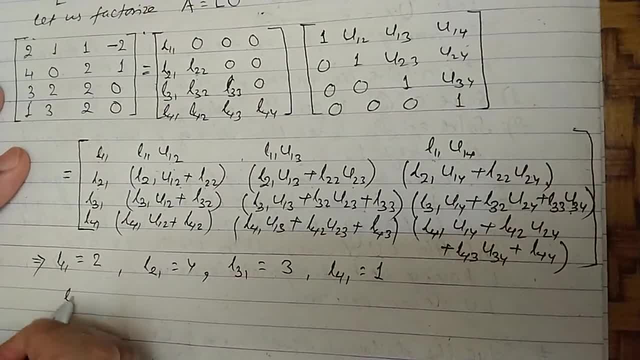 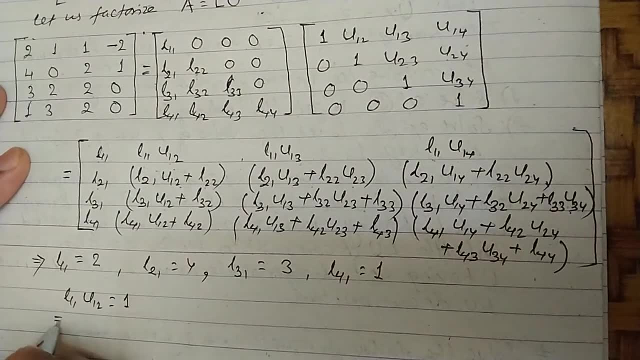 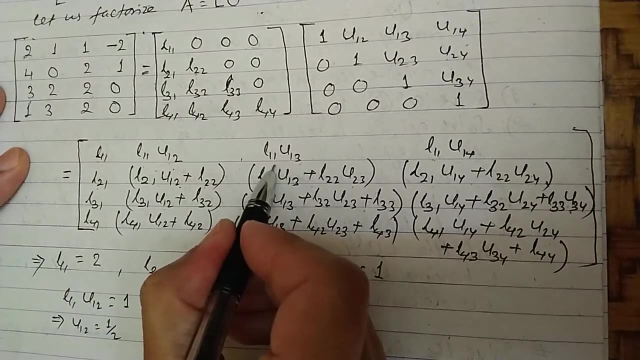 and see what happens: plus 2 plus 2, plus 2 times 2 is equal to all right. so few calculations, not all. so 2 is equal to 1. also, we get what L11 into: U13 is equal to 1.. 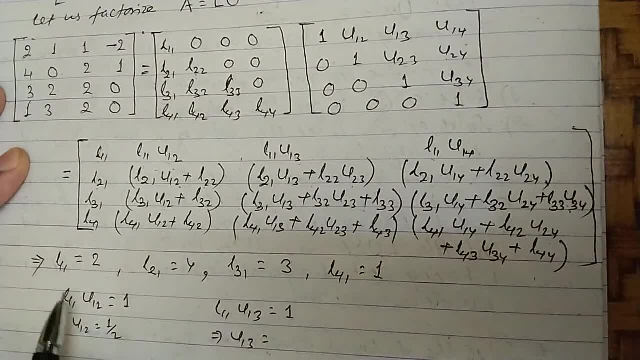 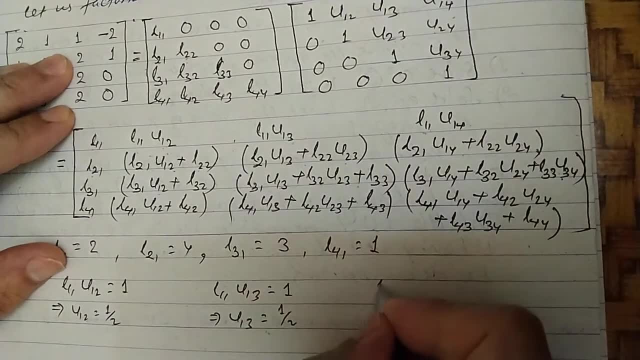 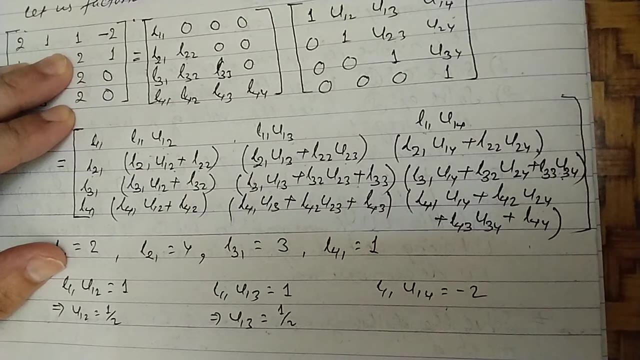 From this we can get U13.. L11 is equal to 1.. This is also half. Let's compare another coefficient, L11 into U14 is equal to minus 2.. From this, U14 is equal to minus 1.. 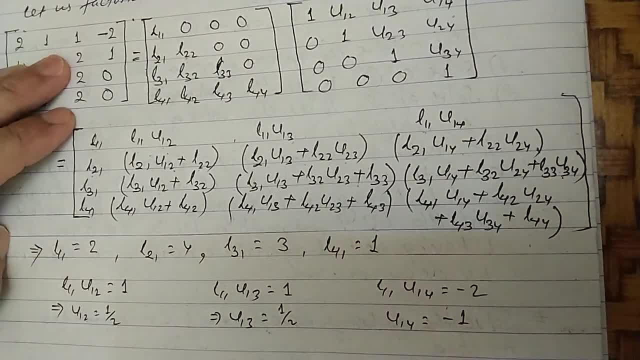 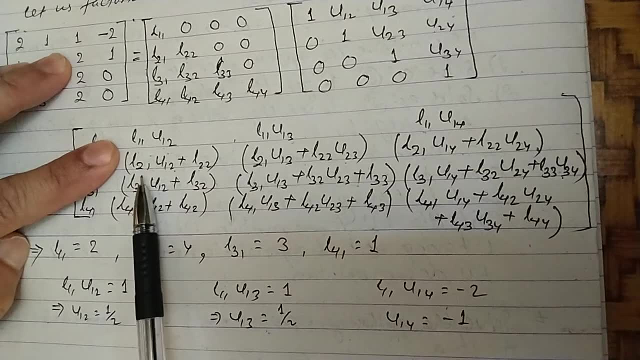 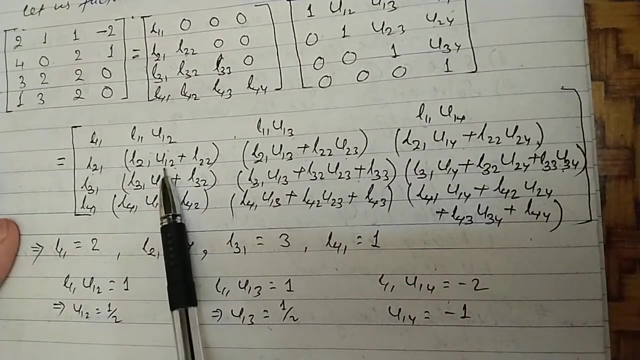 Because L11 is equal to 2.. Now let's go to S. What do we have to get from S? L21 into U12 is equal to L22.. L22 is not there, So let's get L21 into U12. 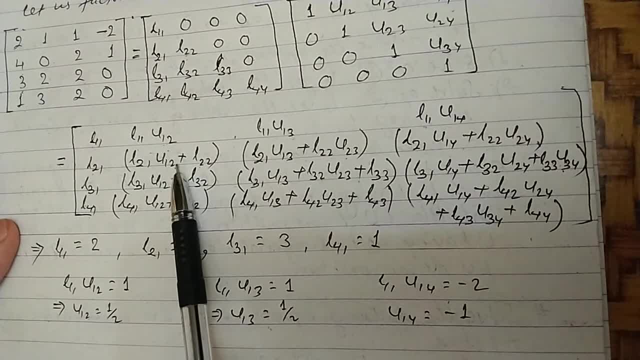 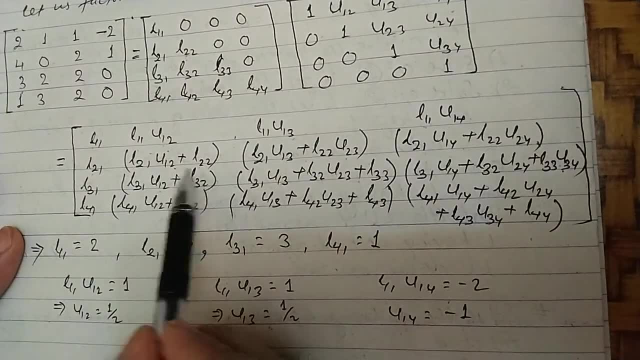 L21 into U12 is equal to L22.. When we get the value of L22, we get the value of L22.. Because U12 we have just calculated L21, we have already written over here, So we get L22.. 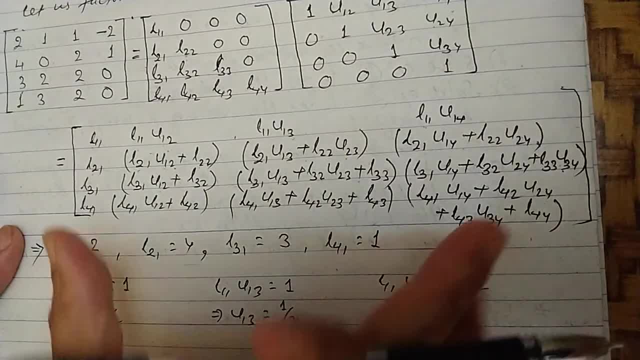 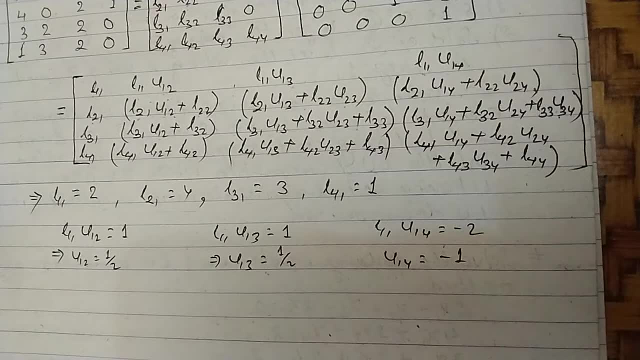 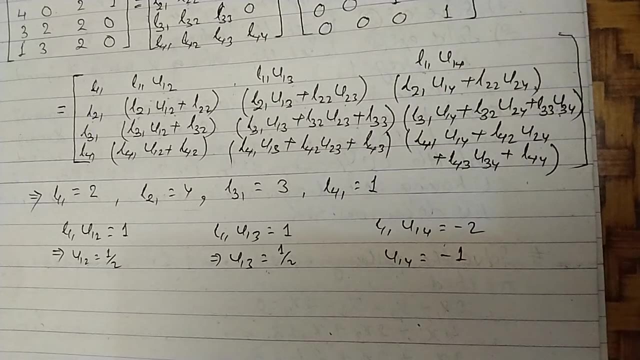 So we have to get all the values. It is lengthy, It will take time, But we get all the values In this work. let me list out the values. So I will try to list out the values. Write down all the values of U and L. 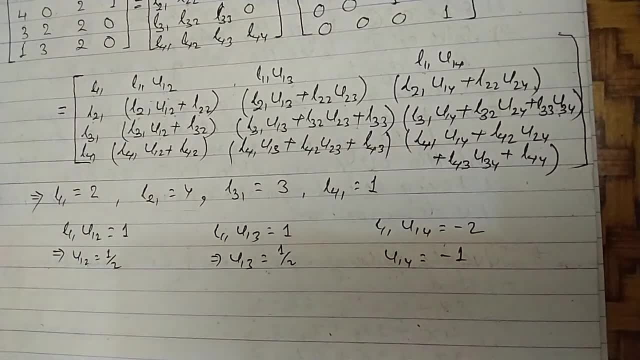 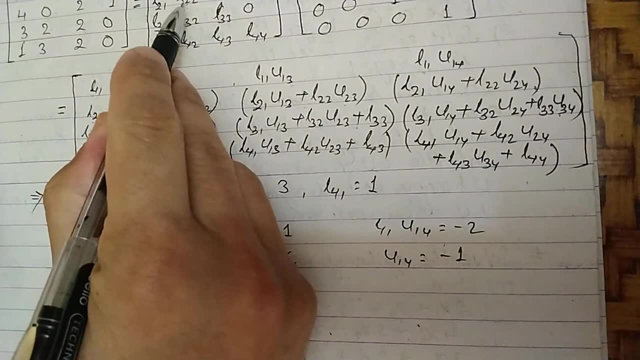 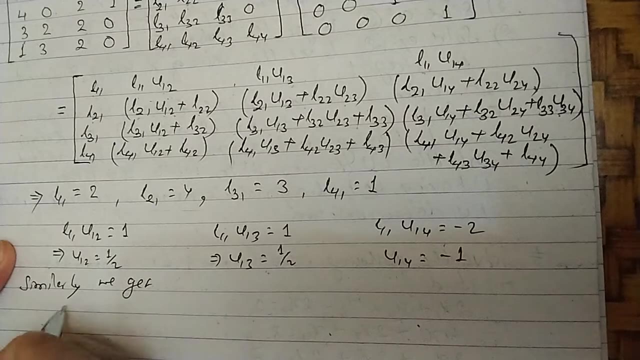 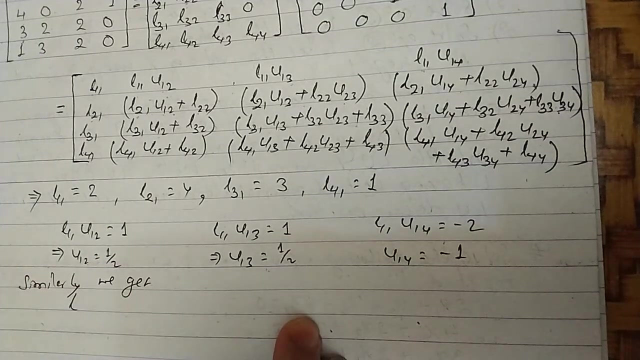 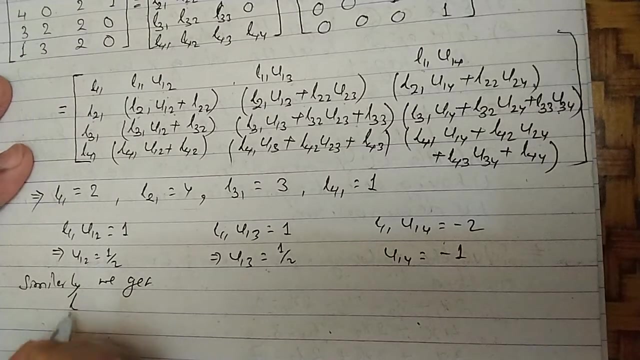 So we can find out. So we have written this- How many L22 will come. Similarly, we get Alright. So we have written all the values. We have written L22.. So L22.. Select L232.. 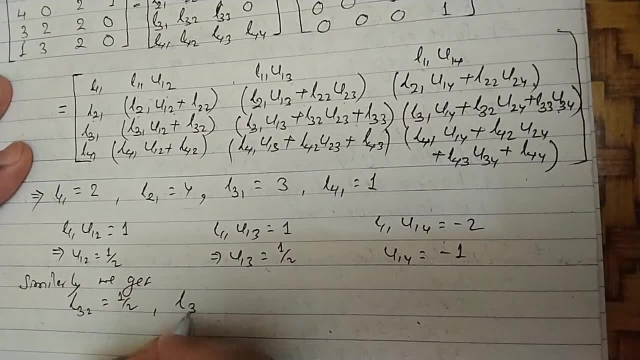 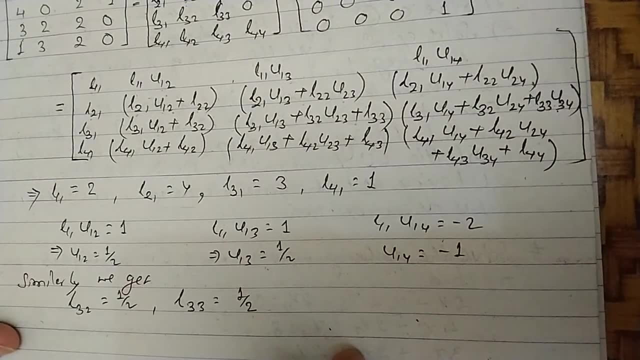 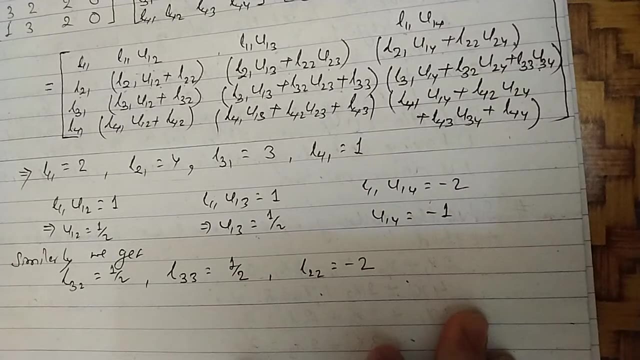 It will come in the half. Similarly, we have DL33: It will come in the half. We have tick L22 in it, So we can also get L22.. L22 will come here This way. let's get U23.. 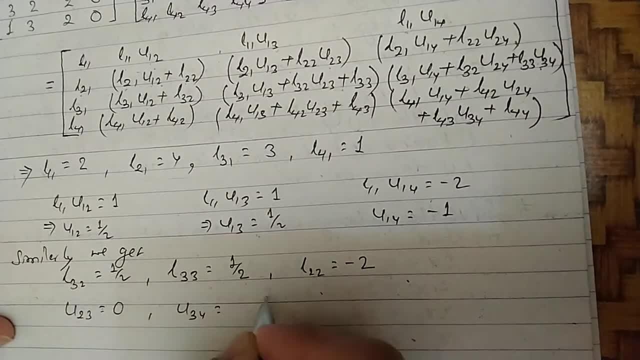 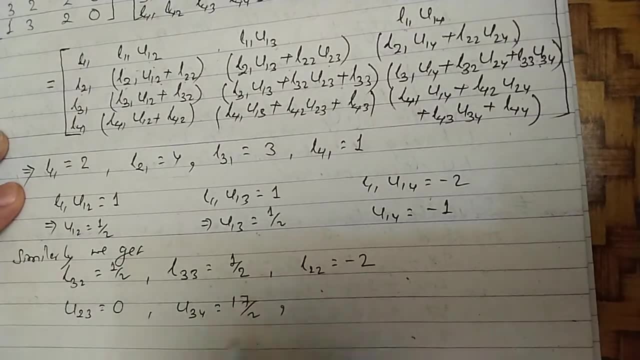 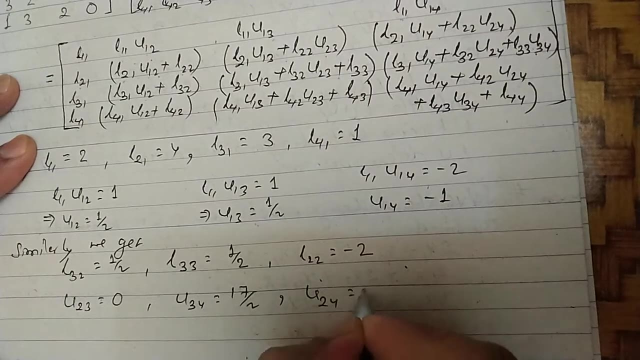 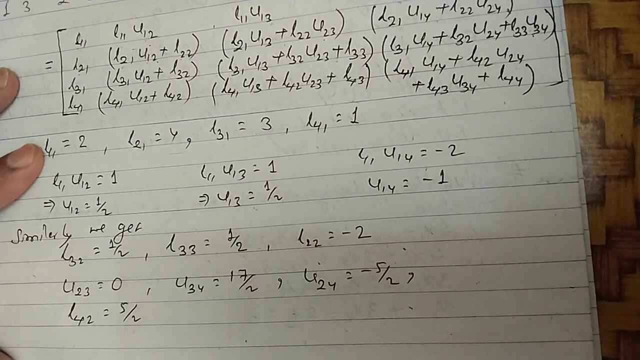 This will come as zero: U34. So this 17 by 2 is coming In this way: U24 is coming. this minus 5 by 2 will come. L42 is coming. this 5 by 2 will come. L43 is coming. this 3 by 2 will come. 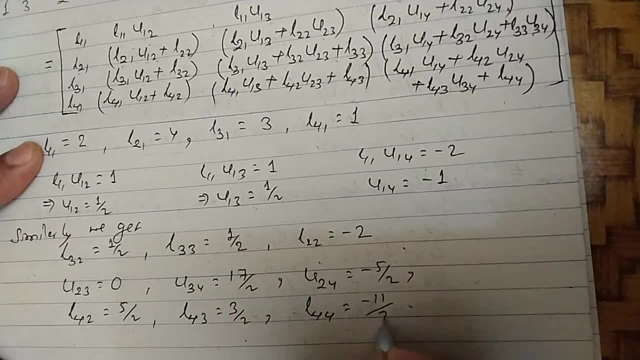 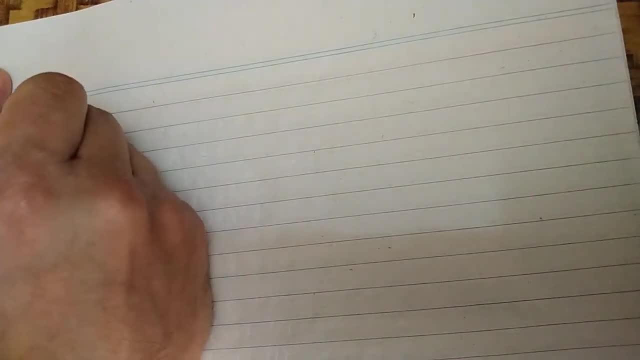 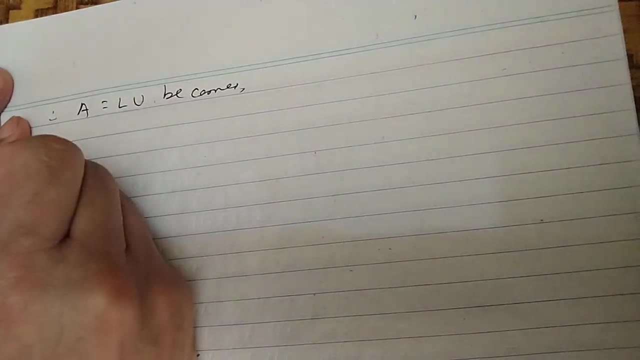 L44 is coming, this minus 11 by 2 will come, So therefore A equals to LU becomes In this way: write the value of A: 2, 1 1 minus 2: 4, 0. 2, 1, 3, 2. 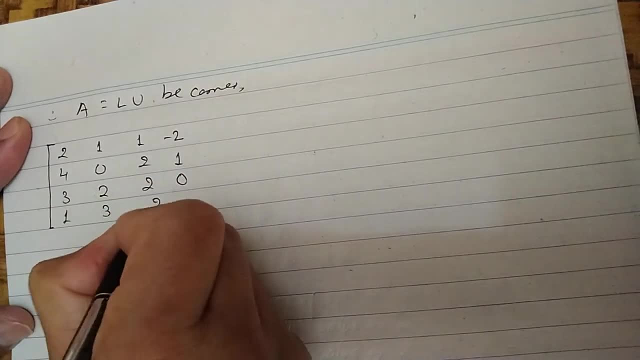 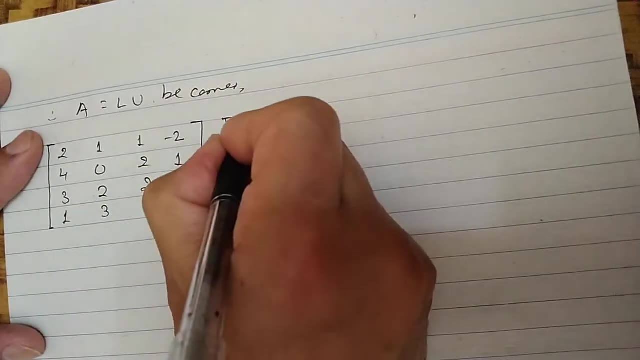 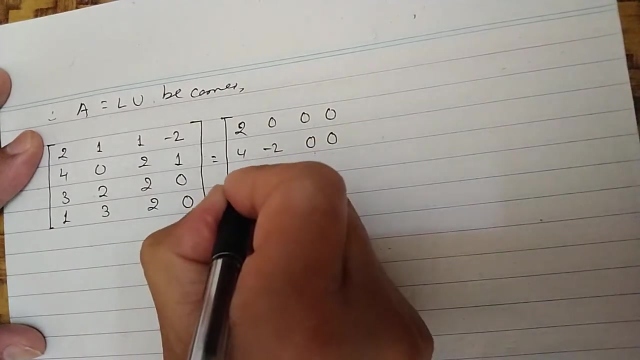 2 0 1, 3, 2 0. So write the value of L: 2 0 0 0, 4 minus 2 0 0, 3, 1 by 2, 1 by 2 0, 1, 5 by 2. 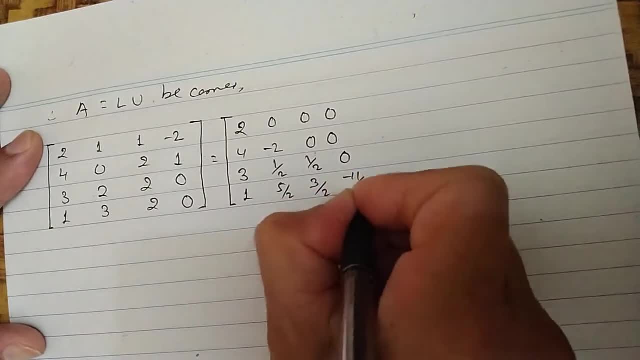 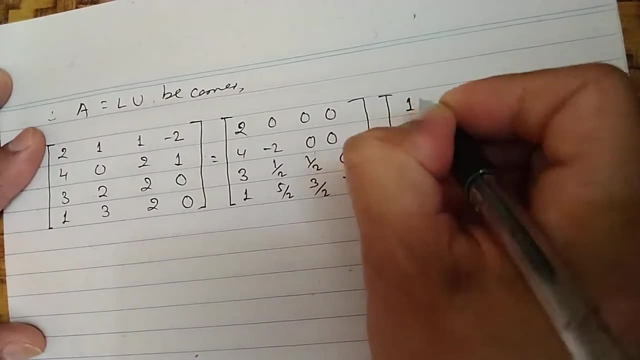 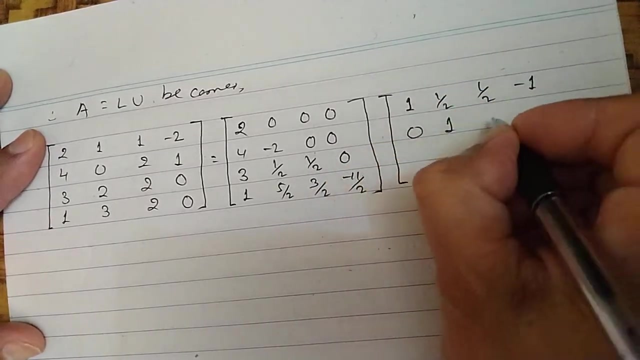 3 by 2 minus 11 by 2, 3 by 2. That is your L, And what is your U? 1, 1 by 2. 1 by 2 minus 1, 0, 1, Your 0, I rather. So- minus 5 by 2. 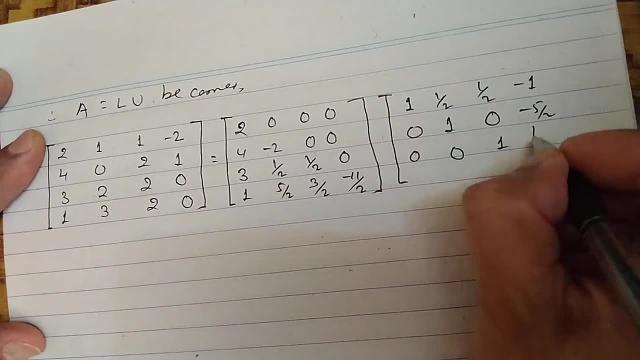 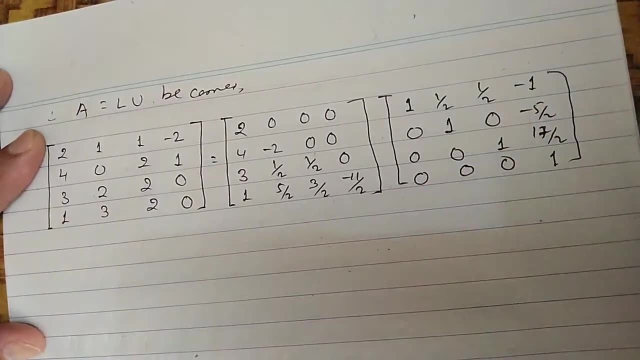 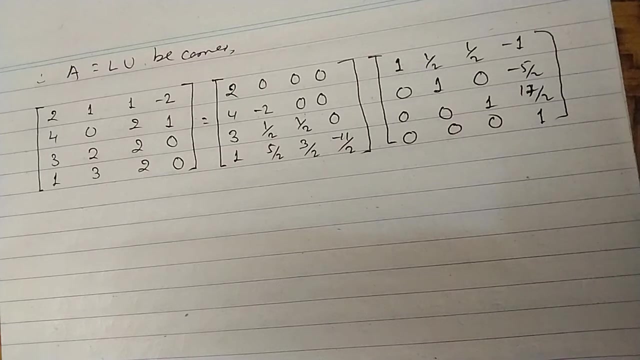 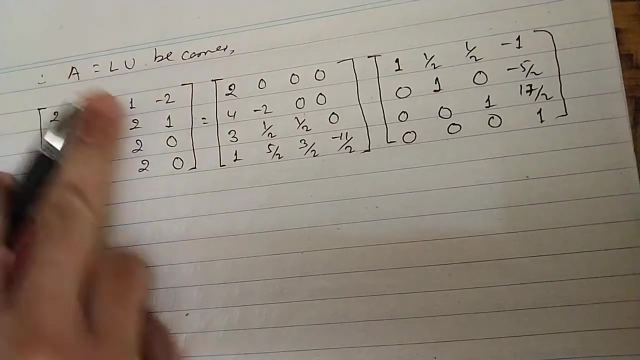 0 0 1 17 by 2 0 0 0 1 0 1 by 2 0 1 by 2 0 0 1, 1 by 2 0 1 by 2. 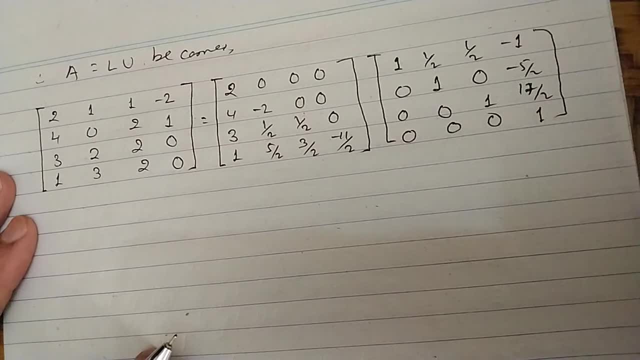 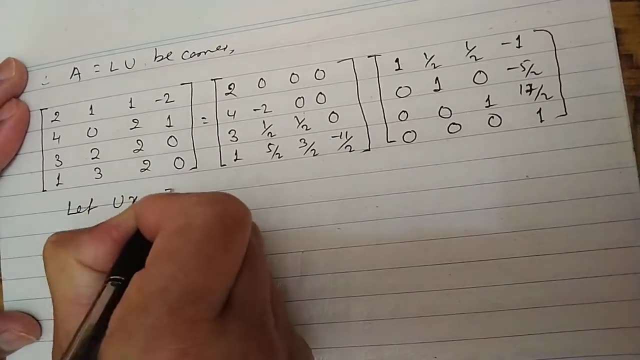 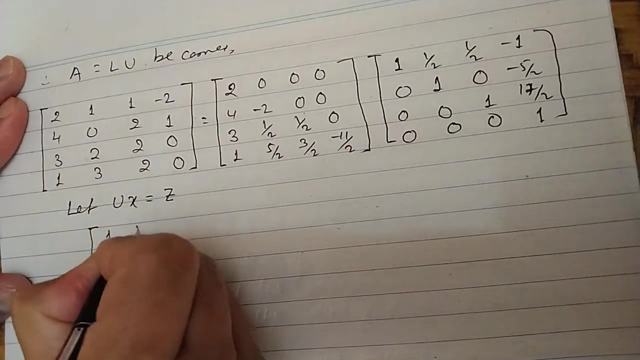 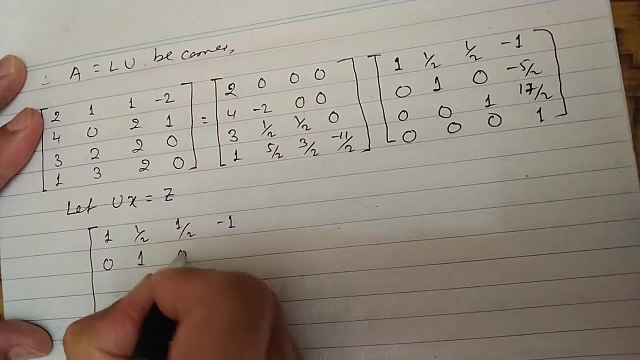 0, 1 by 2. Let us suppose ux equals to z, where z is unknown vector, so we will write u as it is. So u is 1, 1 by 2, 1 by 2, minus 1, so 0, 1, 0, minus 5 by 2, 0, 0, 1, 17 by 2, 0, 0, 0, 1,. this is your u. what is your x? x1, x2,. 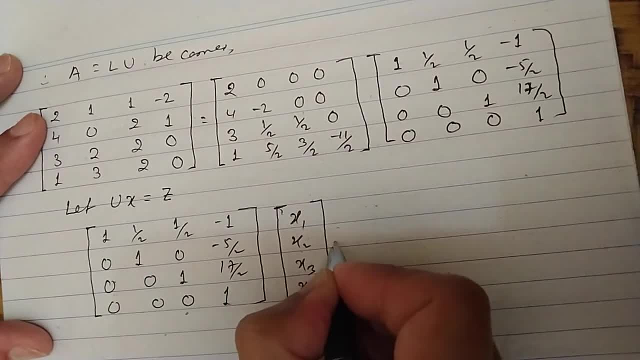 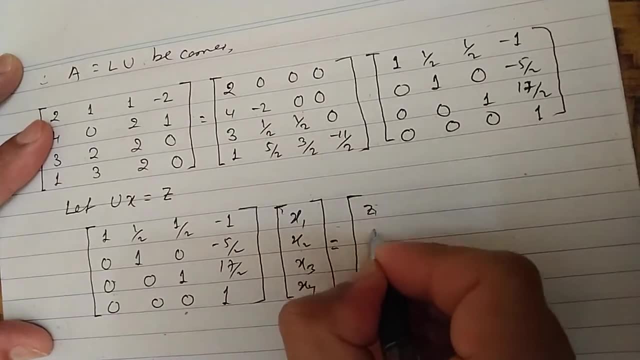 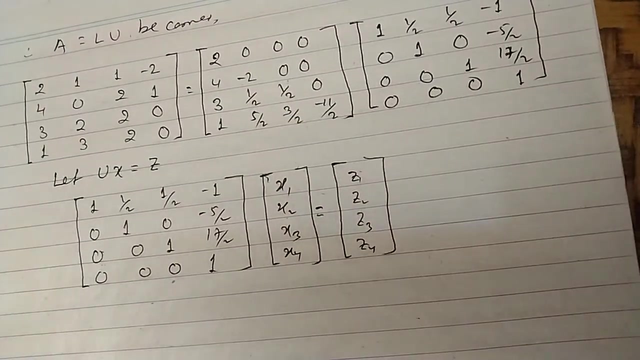 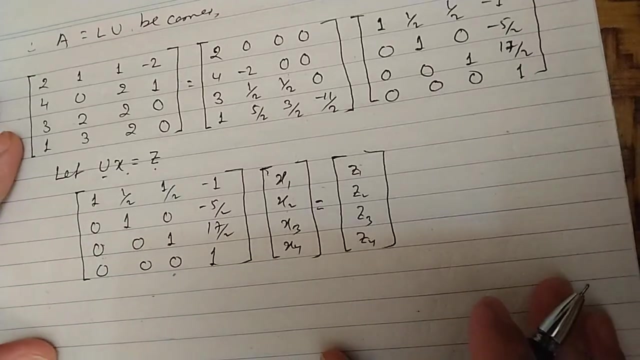 x3, x4, and what is z? z1, z2, z3, z4, so if you suppose ux equals to z, then the original system of equation. what will happen then? we have so: what is u, what is u, what is? 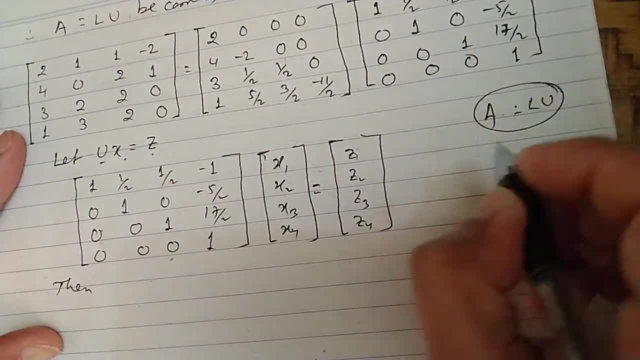 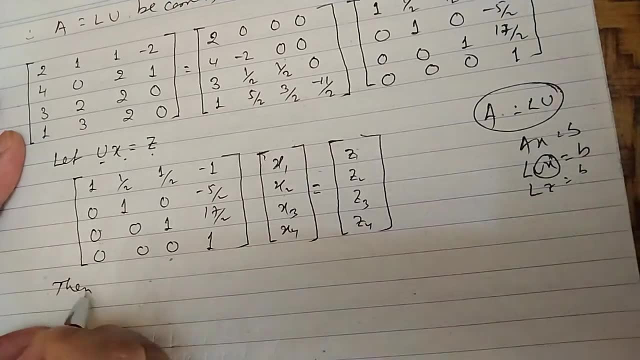 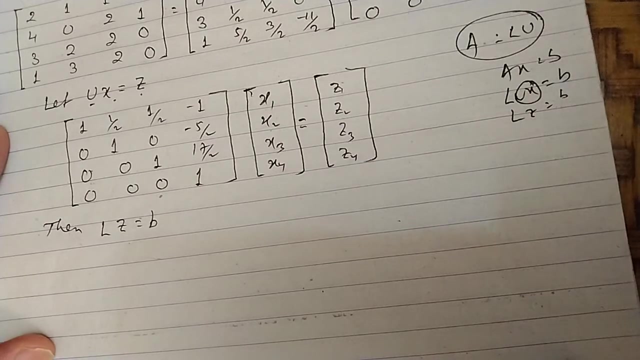 z, so a equals to l? u, you suppose so a x equals to b, so l? u x equals to b? l i suppose z equals to b. so what will happen? l into z equals to b, so l into z equals to. 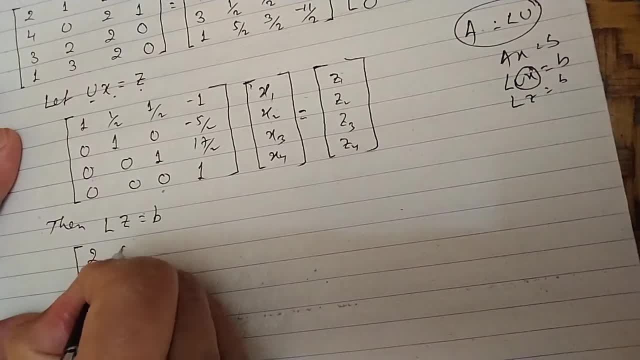 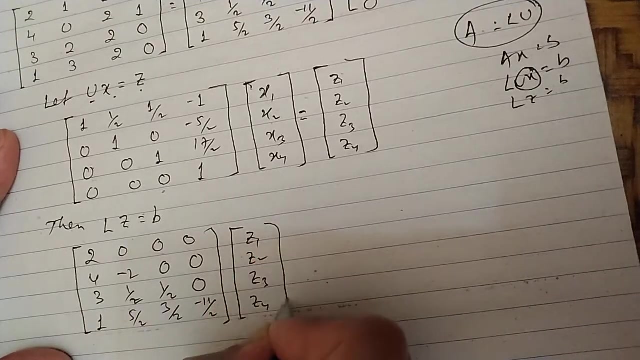 b. what will happen? you write l. we have 2, 0, 0, 0, 4, minus 2, 0, 0, so 3, 1 by 2, 1 by 2, 0, 1, 5 by 2, 3 by 2, minus 11 by 2,. z is unknown, z1,, z2,, z3,, z4, and b is 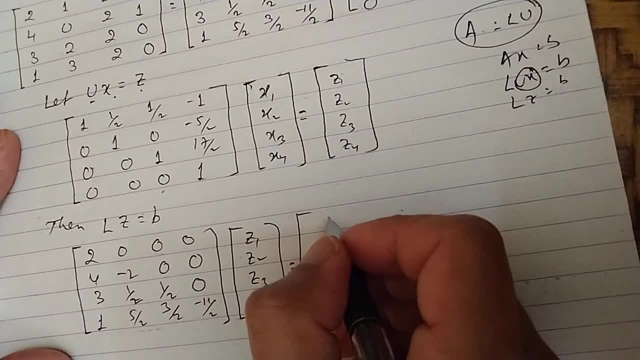 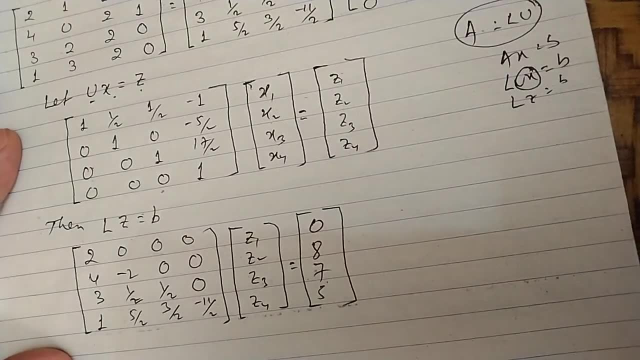 given in the equation. so what is b's value? 0,, 8,, 7,, 5,. so as per time, what is solved by z1, by the forward substitution, so z1 will be equals to 0,, while over down so 2. 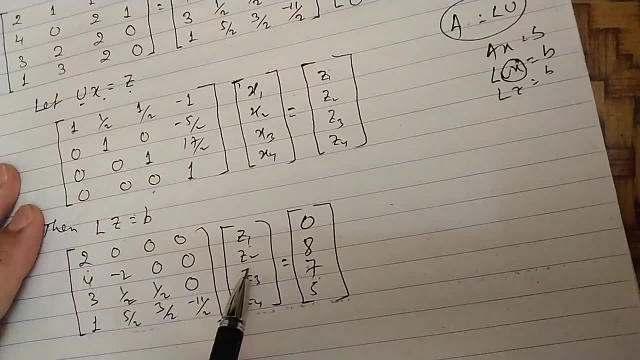 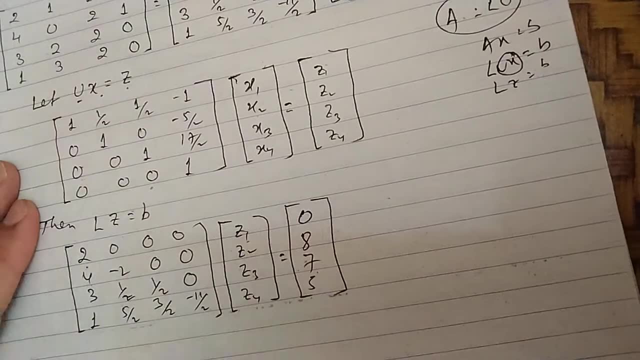 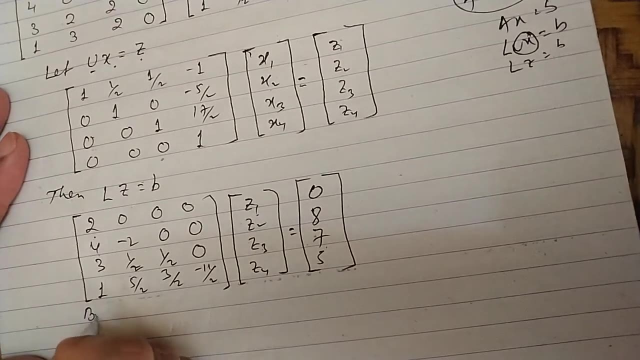 into z1 equals to 0,, 4 into z1, minus 2 into z2, equals to 8, put z1 equals to 0, minus 4, and so on, so you can get the value of z from this equations. okay, so by forward. 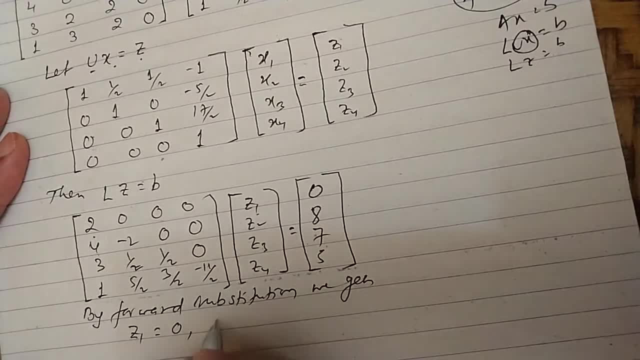 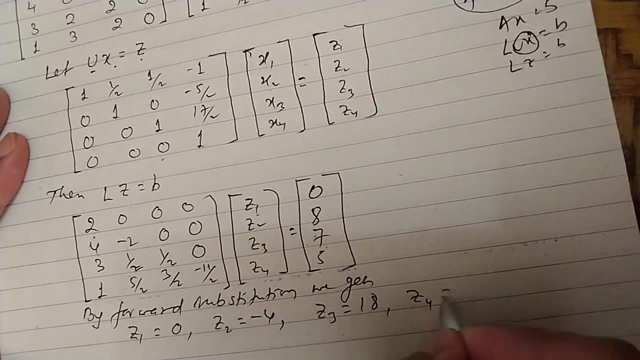 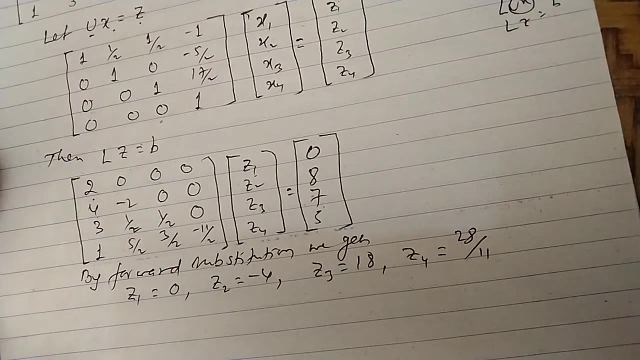 substitution, we get z1 equals to 0, z2 equals to minus 0.. minus 4, z3 equals to 18 and z4 equals to 28 by 11. okay, now it's easy. so put this value of z over here. you will get the value of x and x will be the answer. 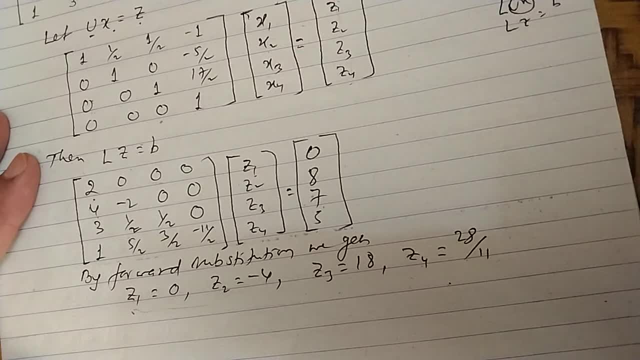 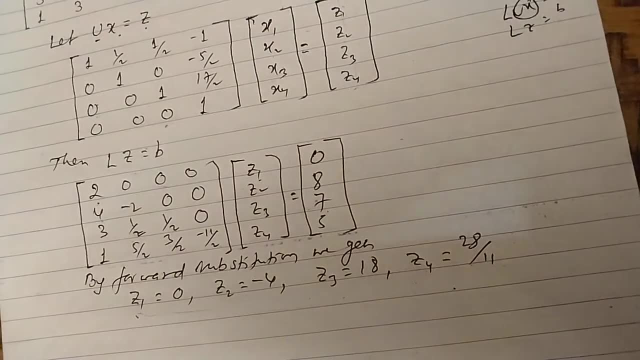 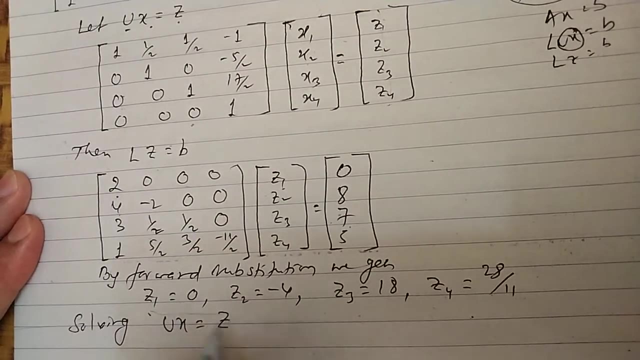 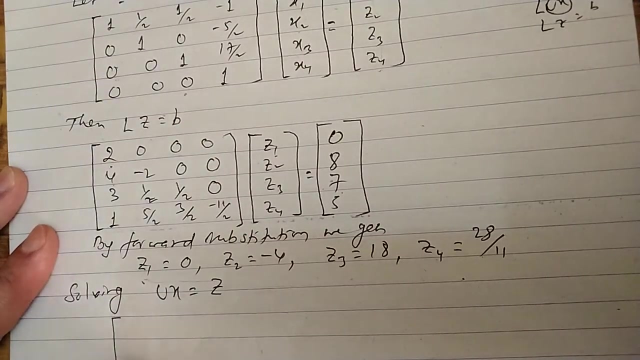 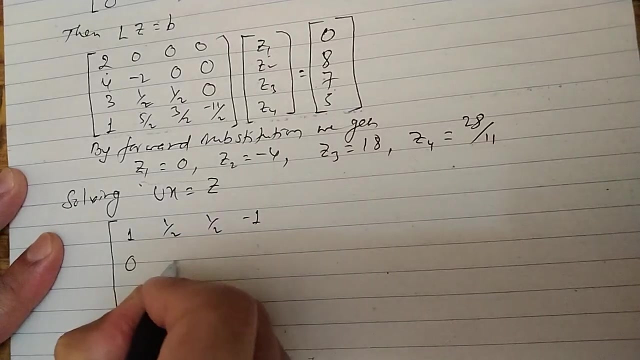 oh, this one x when i go, i'm wrong. so solving what ux equals to z. for z, you'll get the. so sorry, for x, you'll get the answer. so put u over there, the u you. it's a? u umbro 1, 1 by 2. 1 by 2 minus 1: 0. 1 0 minus 5 by 2, 0, 0, 1. 17 by 2, 0, 0, 0, 1. 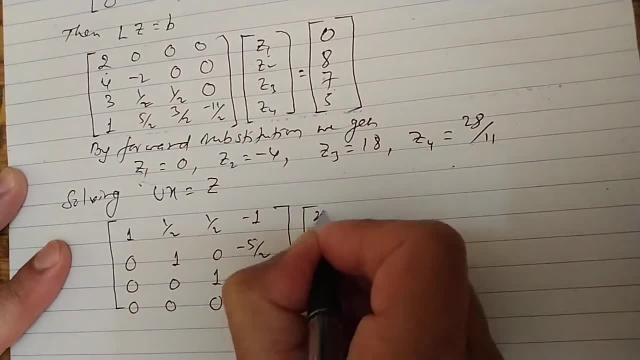 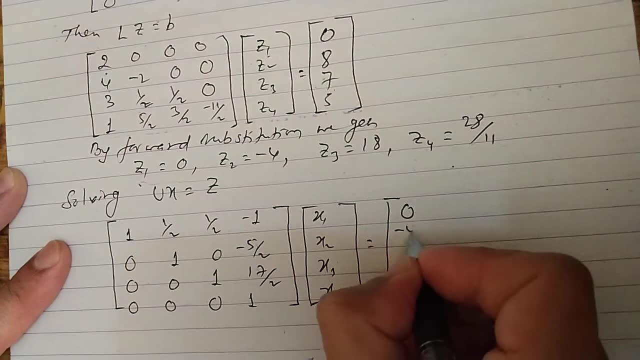 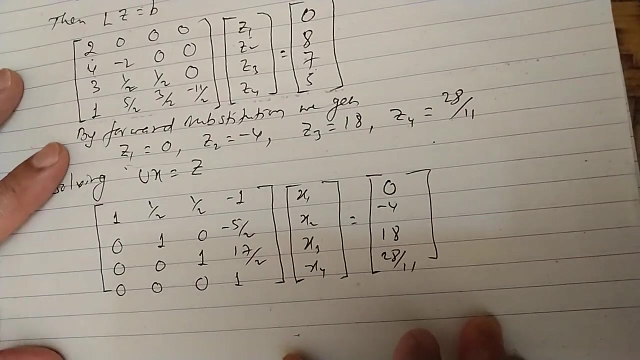 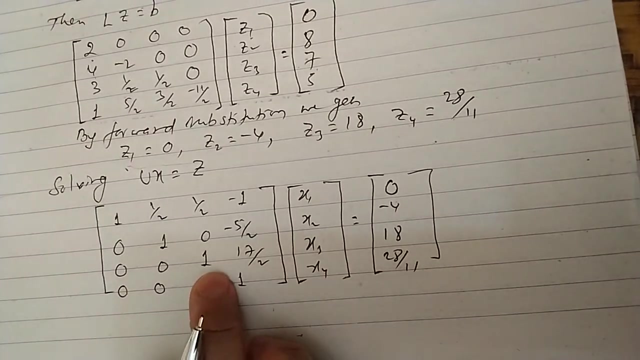 x is the unknown- x1, x2, x3 and x4. and we have just calculated z as what: 0 minus 4, 18, 21, 28 by 11. so by using the backward substitution x1, 28 by 11, so this x3 plus 17 by 2, x4 equals to 18, you'll get the value for x3. 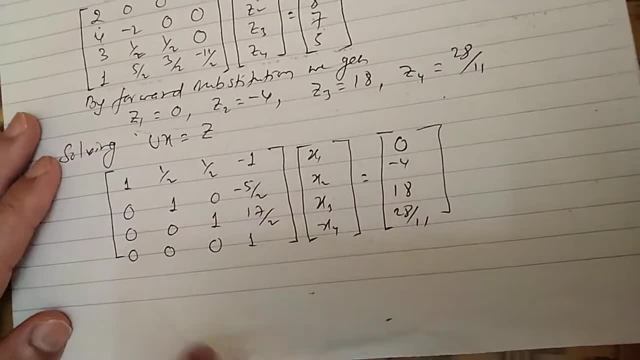 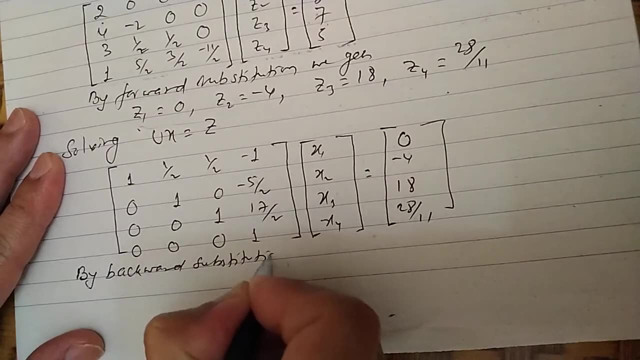 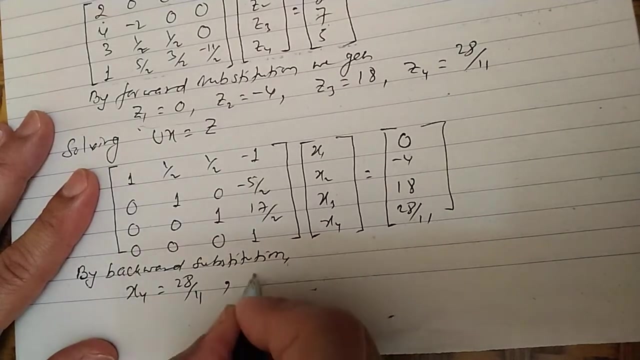 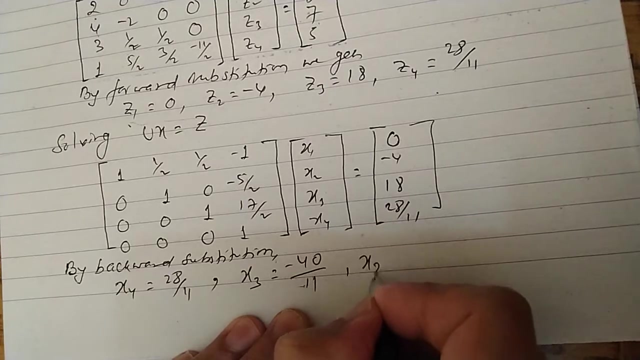 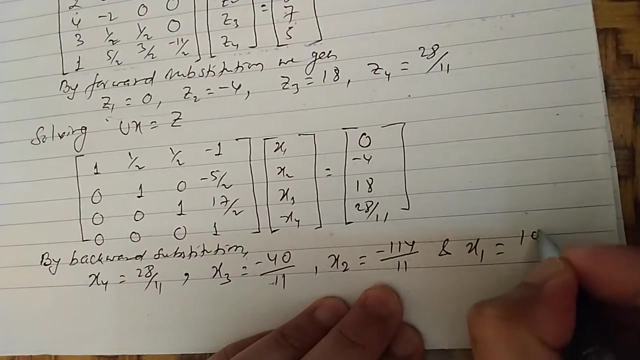 so by backward substitution you will get the value for x3. value of x4 equals to 28 by 11, value of x3 to be minus 40 by 11, value of x2 to be minus 114 by 11 and x1 105 by 11. so these are the solution if you substitute. 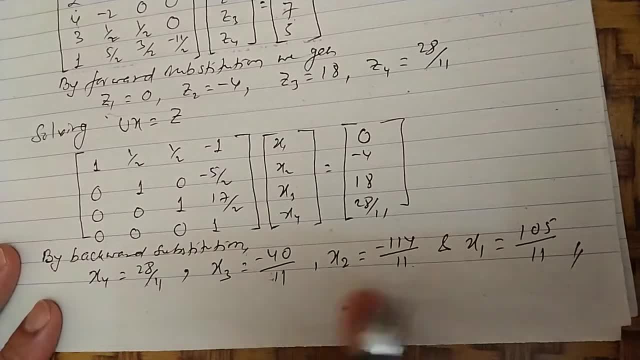 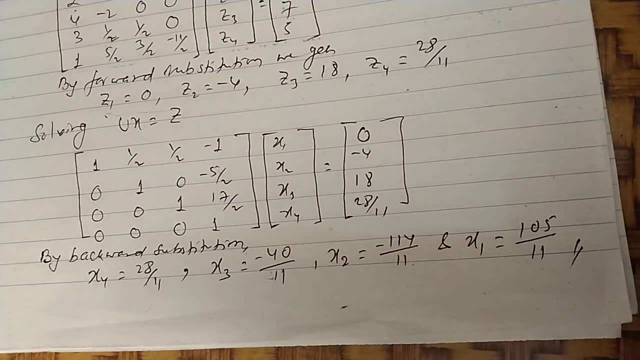 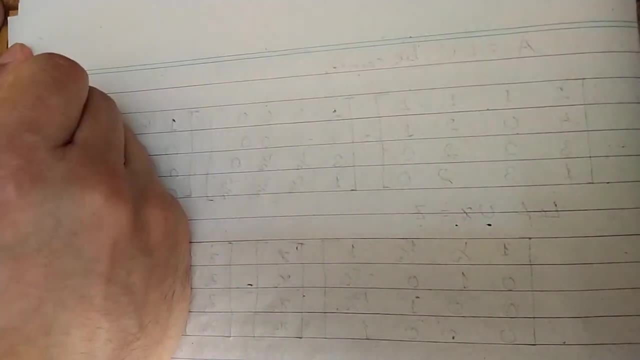 these values in above system of equations. so with the equation system of equation coefficient here can your values are substituted or not. right inside will say that just as well. but the right hand side will satisfy the left hand side, right hand side, right hand side, equal also. so that means you are getting the correct answer. so another topic: uh, that is quite uh, similar to uh. 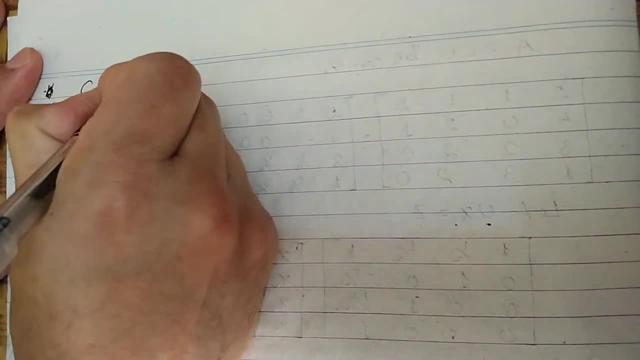 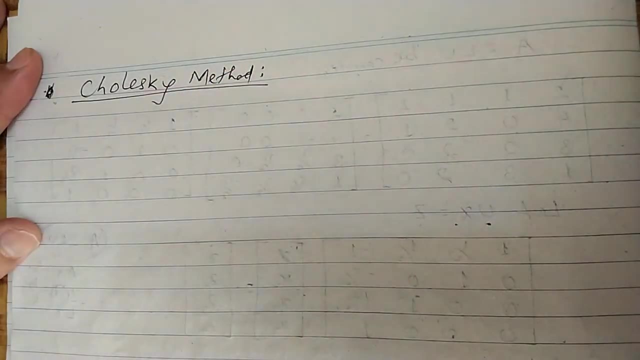 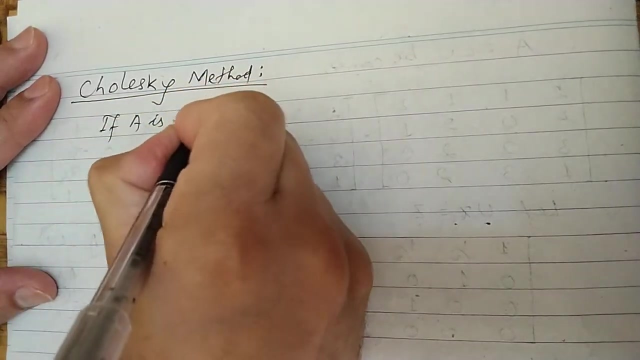 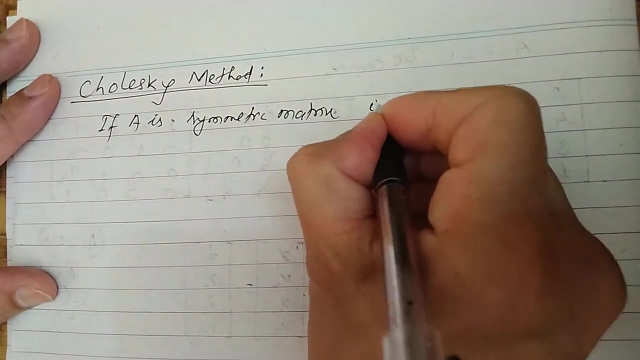 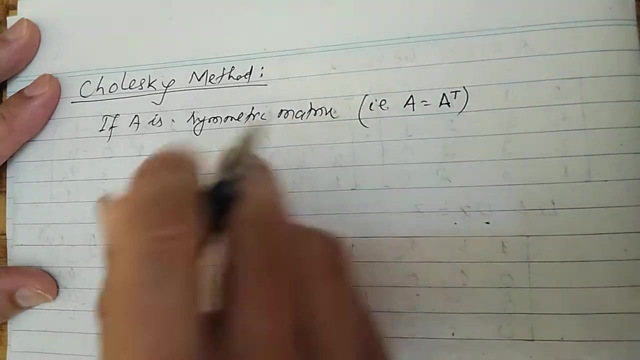 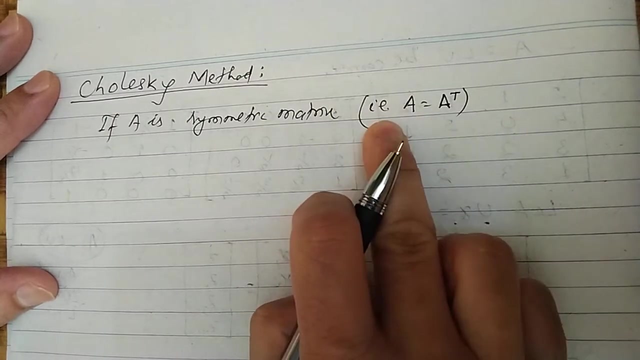 elute composition with known as cholesky c-h-o-l-e-s-k-y cholesky method. it's quite similar to elute composition method, but there is a condition used. oh, so if a is symmetric matrix, so symmetric matrix should be equal. so a should be equal to a transpose. so it's okay. 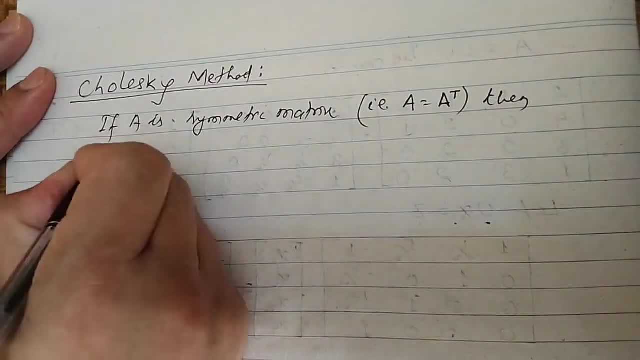 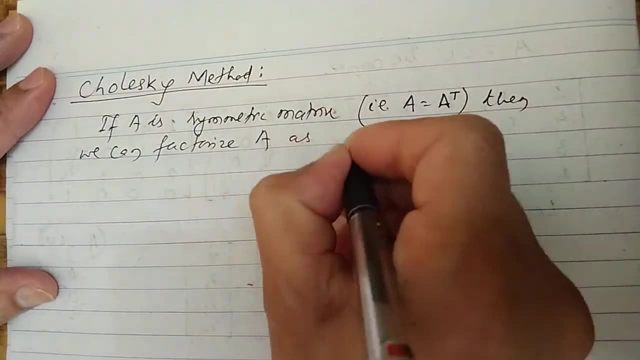 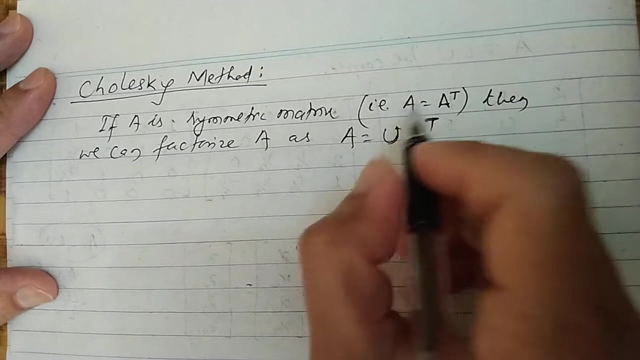 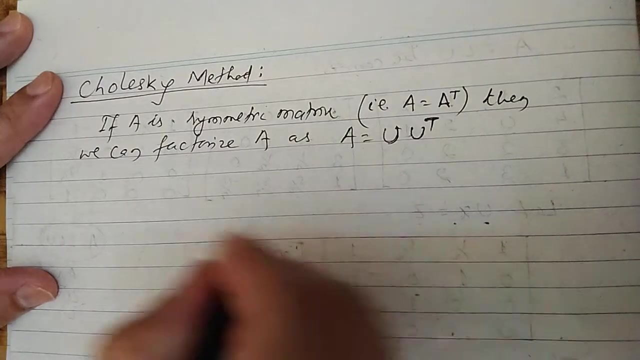 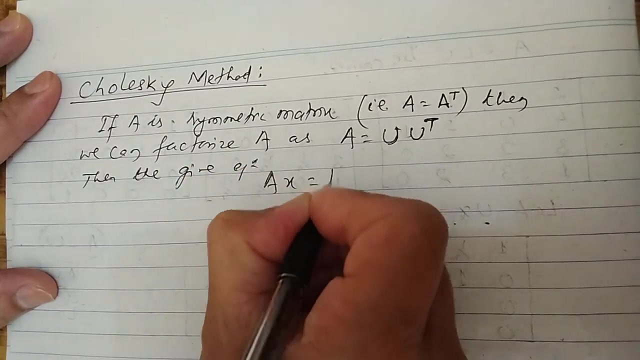 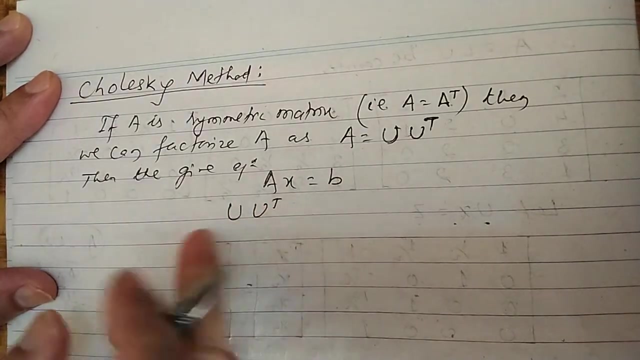 so then we can factorize a as a equals to u into u transpose. coefficient matrix: u transpose then the given equation: ax equals to b, u into u transpose. okay, i'm going to l? u my algorithm, so it's my: u into u transpose, equals to b. 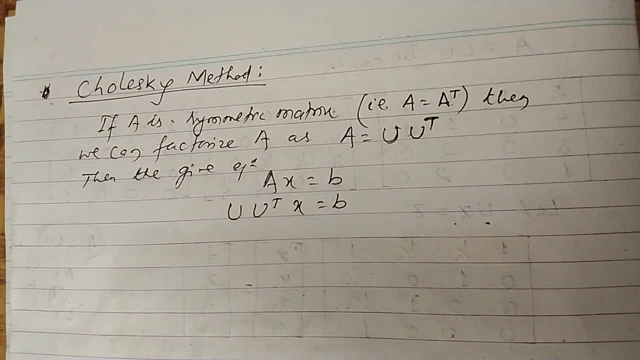 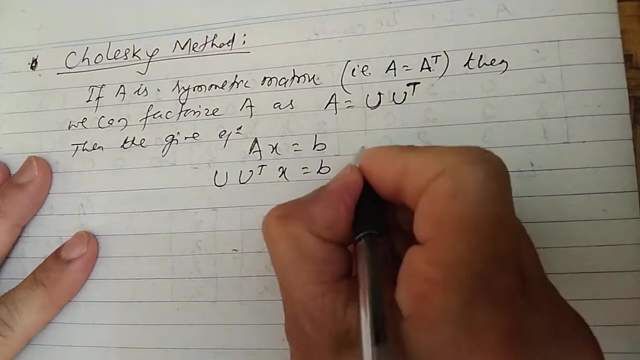 so u into u transpose equals to b, and this is a process like before, u into xz. so suppose you have u into xz, so you can do it like this: let u into x equals to z, or u transpose into x equals to z, anything you like. 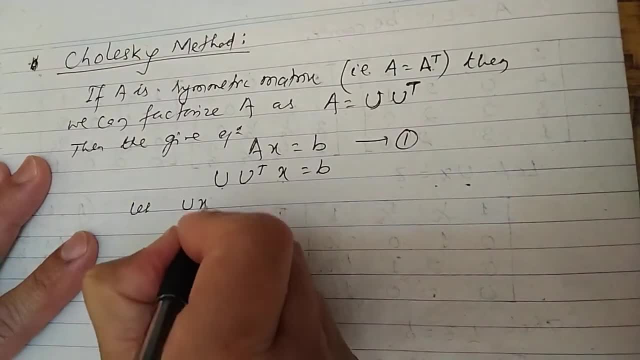 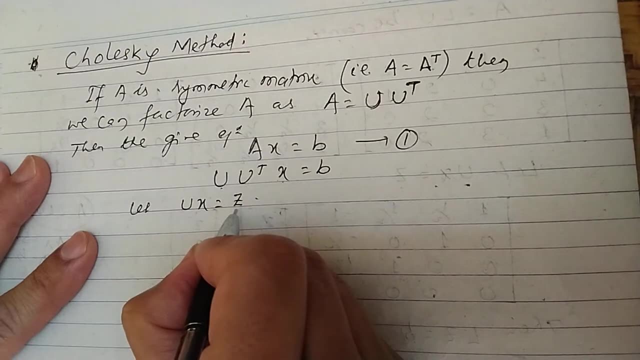 so let ux equals to z, i suppose. let ux equals to z. i suppose if i do ux equals to z, i will get ux equals to z and then do ux equals to z. in this case, If I suppose ux into z, what will be left here? u transpose: 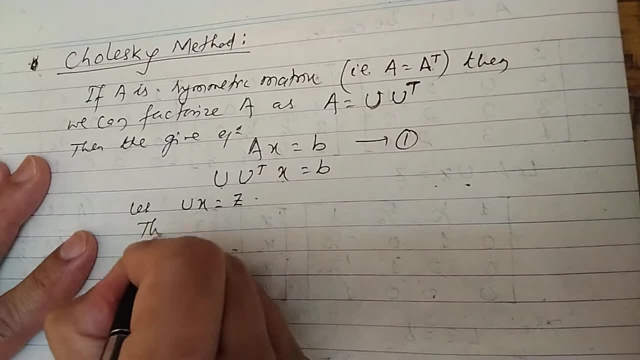 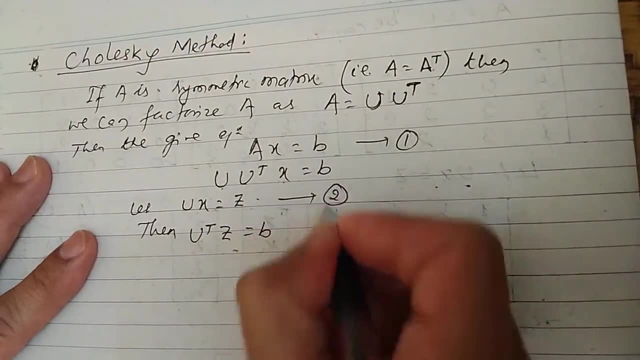 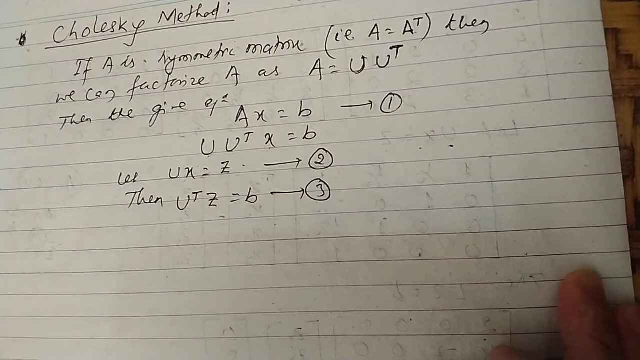 If I have z at the place of ux, u transpose into z equals to b. So let's make equation number 2 and equation number 3.. The process is the same. So here we will not take diagonal elements of 1.. We will take diagonal elements of 1.. 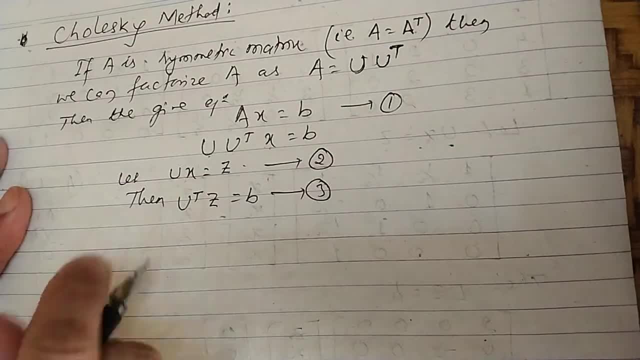 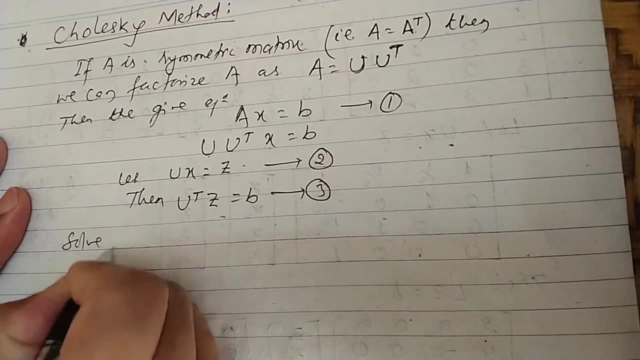 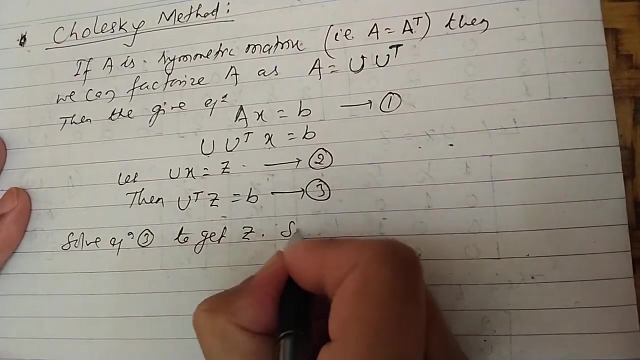 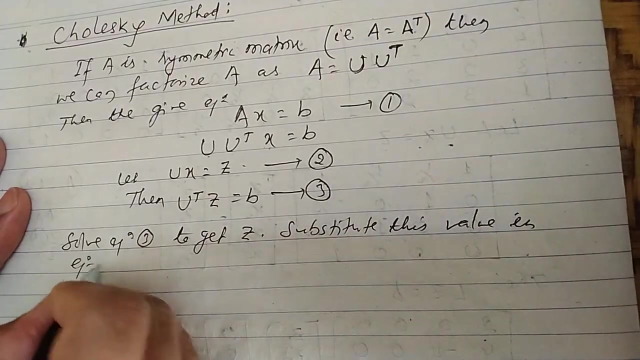 I will give you a problem, I will give you its hints and you try to solve it. So we have these equations with us, So we solve equation number 3.. So solve equation 3 to get the value of z. Substitute This value in equation 2 to get the value of x. 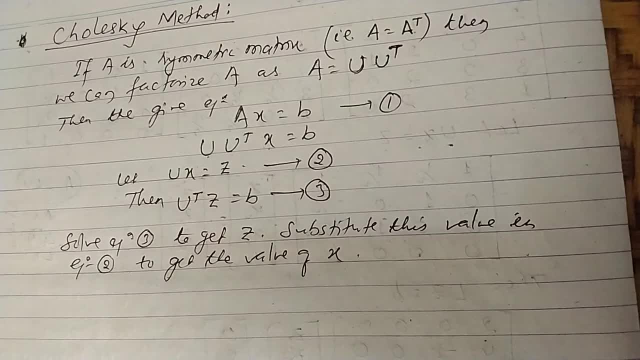 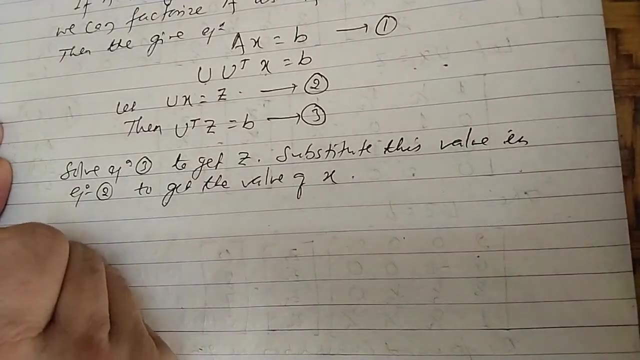 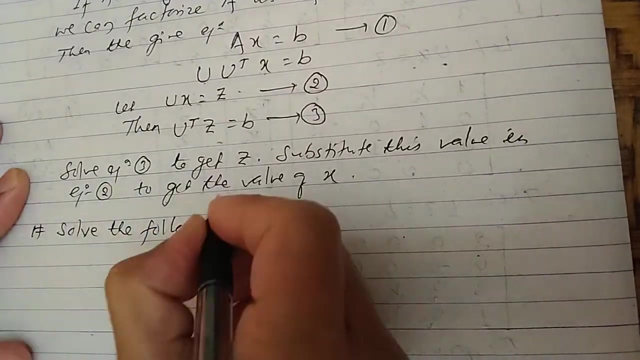 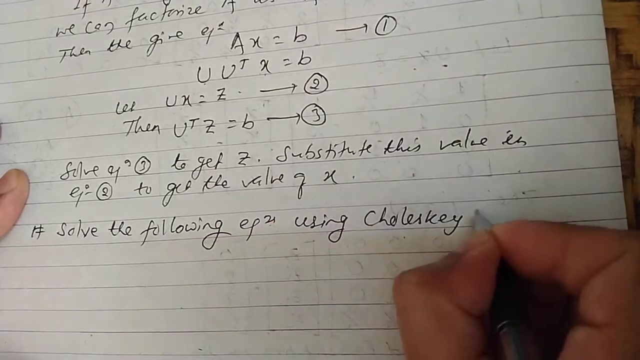 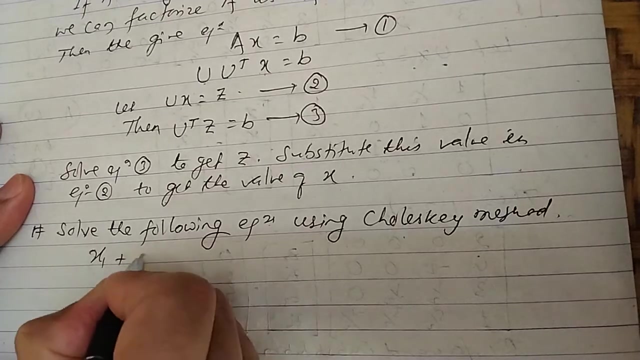 And x will be the solution. So let me write down a problem here. Solve. Solve the following equations using Cholesky method. So I will write down 3 into 3 matrix. follow equations: x1 plus 2x2 plus 3x3 equals to 5.. 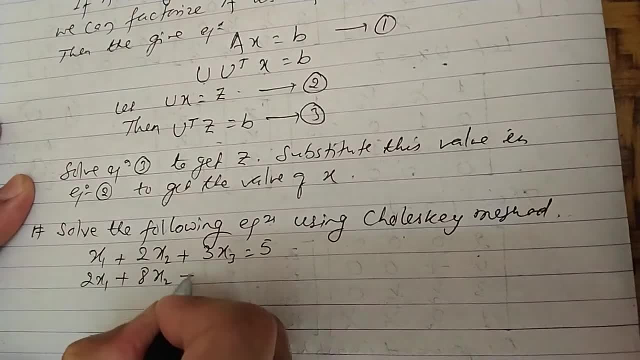 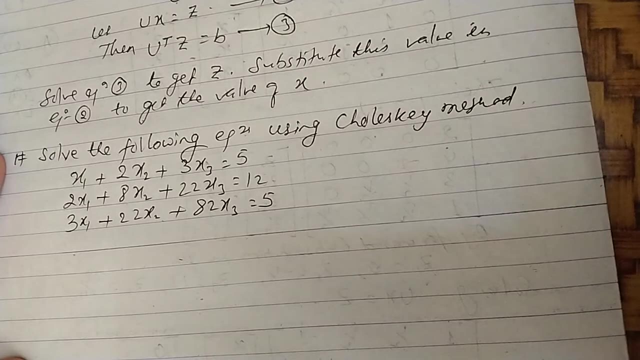 Orgo 2x1 plus 8x2 plus 22x3.. Orgo 3x1 plus 8x3 plus 22x3 equals to 12.. Orgo 3x1 plus 22x2 plus 82x3 equals to 5.. 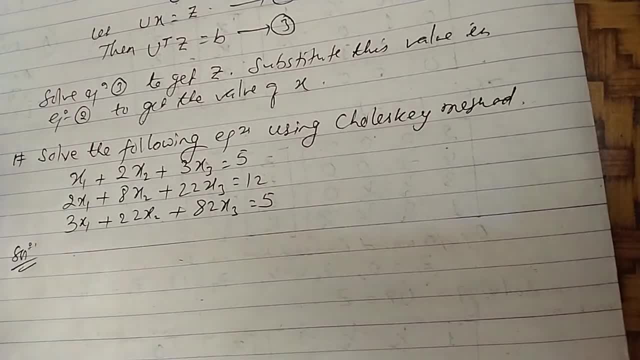 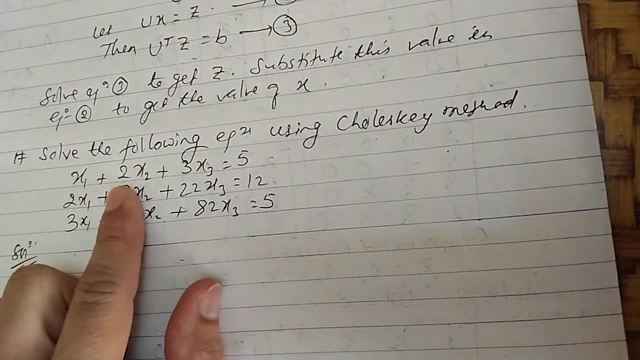 Orgo: 3x1 plus 22x2 plus 8x3 equals to 5.. I also will give you some hints. First, let's solve the question: is using Cholesky method or not? We don't. So you have to give that problem which can be solved by the Cholesky method, which cannot be done if you have already given it. 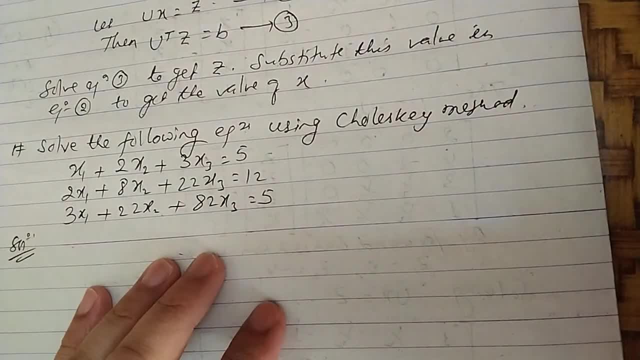 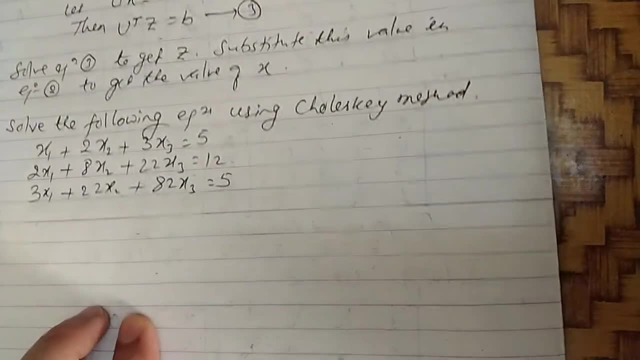 If there is no such thing, then what did you give in the straightforward question? Since the coefficient matrix and its transpose, this condition is not true. It cannot be solved by using the Cholesky method. Please be very clear on this. Look at the coefficient matrix. 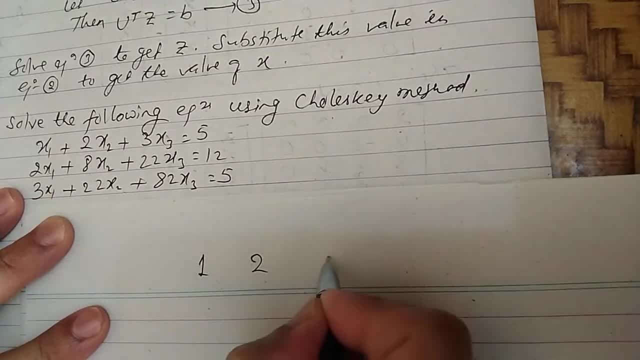 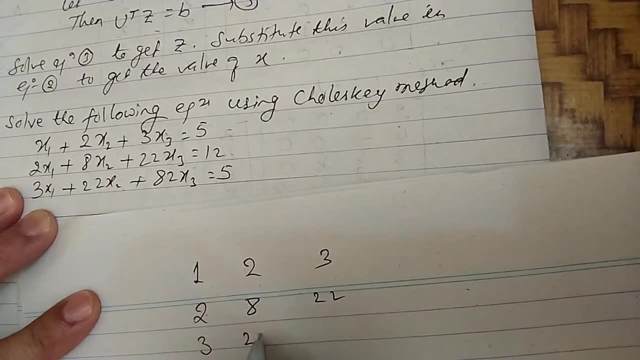 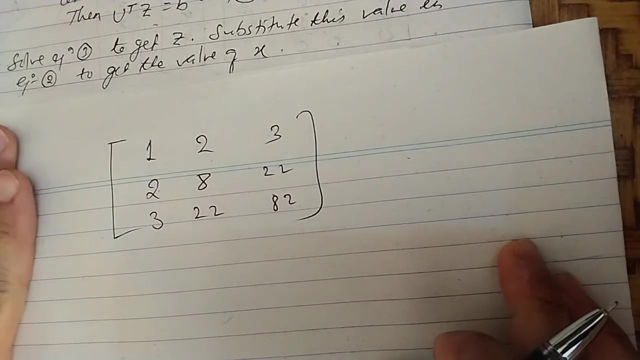 I don't have to do this, I just want to verify you. Sometimes it is not solved. Why can't it be solved? If this condition is not there, then it cannot be solved. This is A. I will write the equation later. 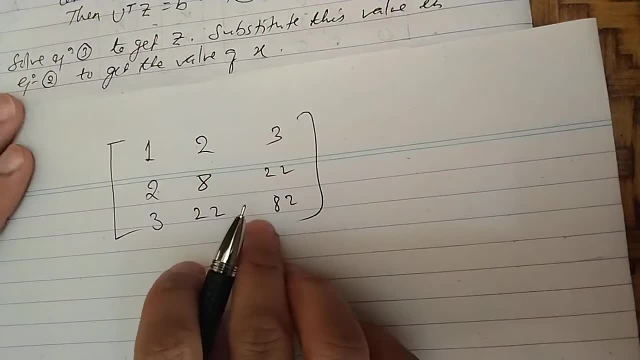 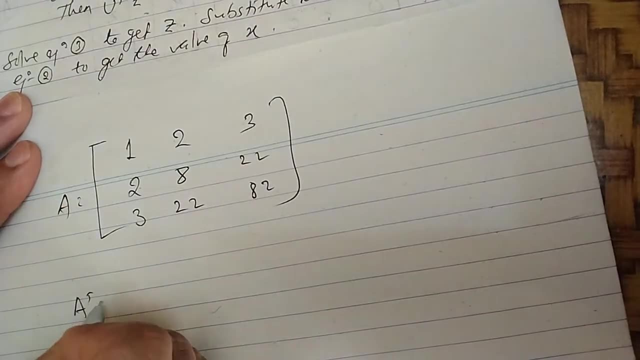 This is A Alright. So what is A transpose? then I will write A transpose. This is A Its. A transpose is also the same. I will write 1,, 2, 3 vertically like this: 1, 2, 3.. 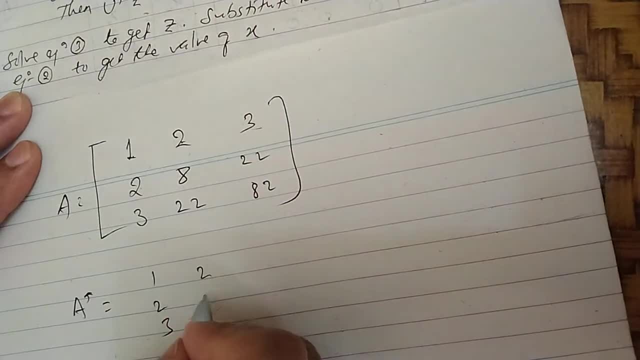 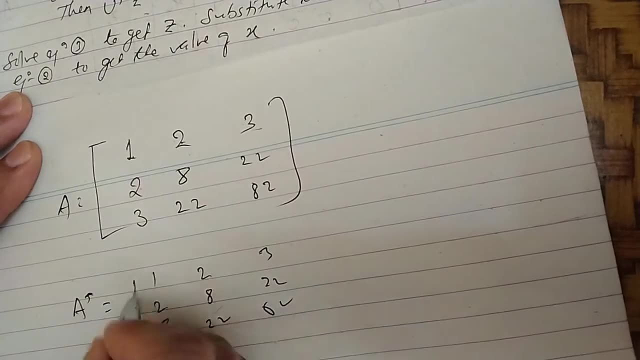 1, 2, 3.. Right, So this one is 2A22.. This one, So write this one in the column. What would it be? 322, 822.. You get the same Equal. So A equals to A transpose. 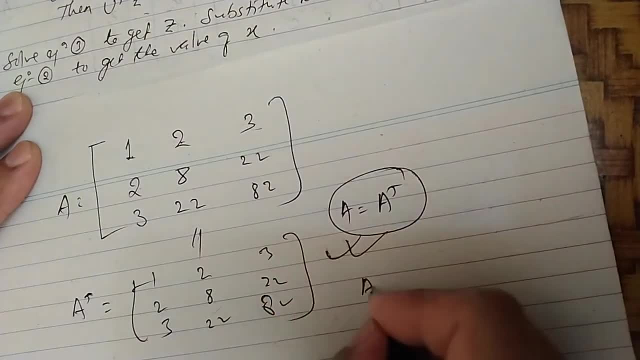 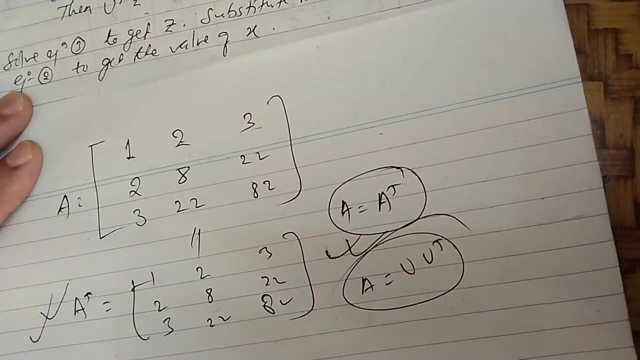 If this condition is there, then you can factorize A equals to U into U transpose, And then you can solve by using the Cholesky method. This problem can be solved by using the Cholesky method. If this condition is not there, then the coefficient is set out. 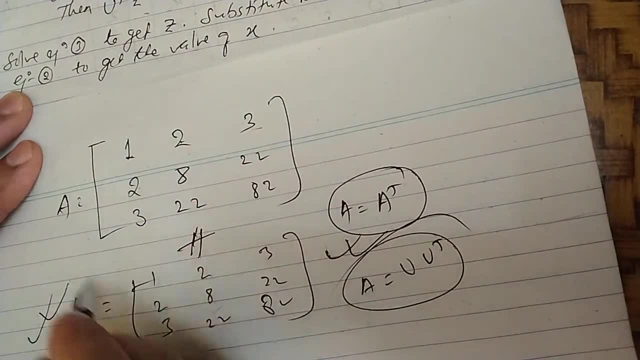 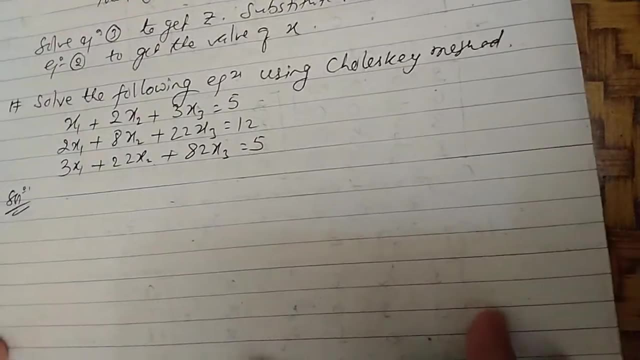 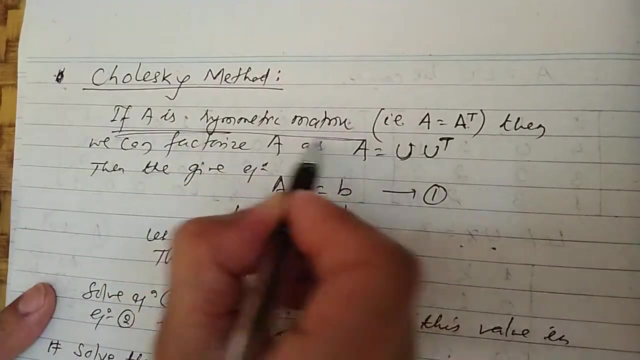 So since this condition is not true, it cannot be solved by using the Cholesky method. Write down clearly and move on to the next question. So this is a very important condition if A is a symmetric matrix. So I think you can do it now. 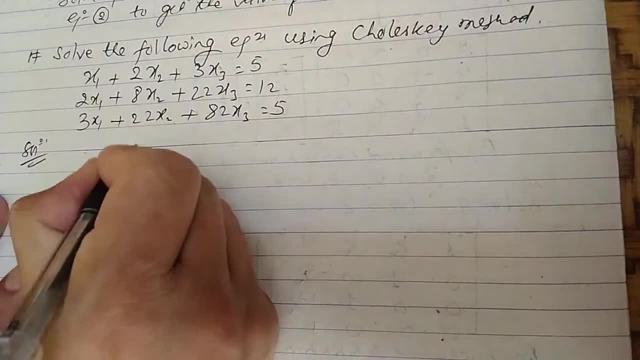 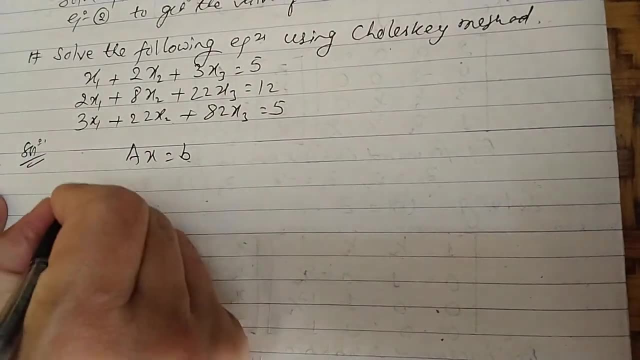 I will show you. So I have not written all these equations repeatedly, because if you write in this form, it will be easy for you. Now we can understand what is A, what is X and what is B, So AX equals to B. 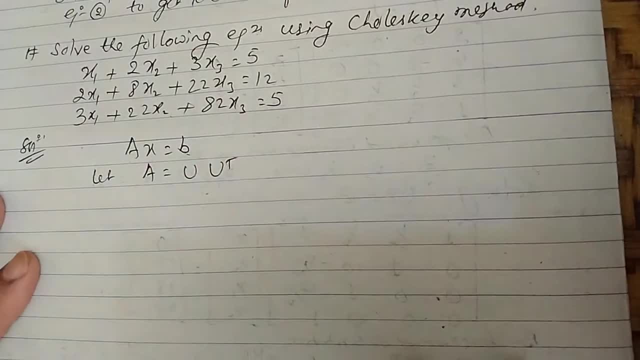 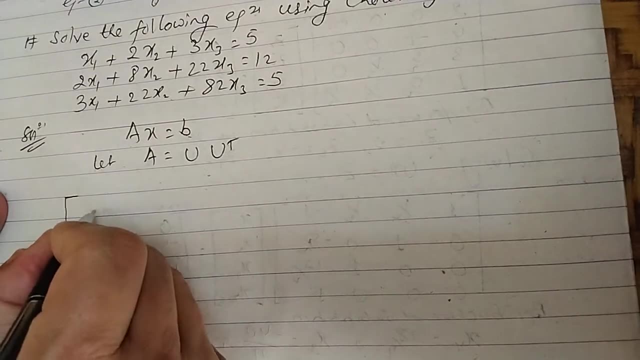 So let us factorize A equals to what U into U transpose. alright, Now write U and U transpose, and the rest will be complete. So what is 1, 2, 3? And what is 2, 8, 22?? 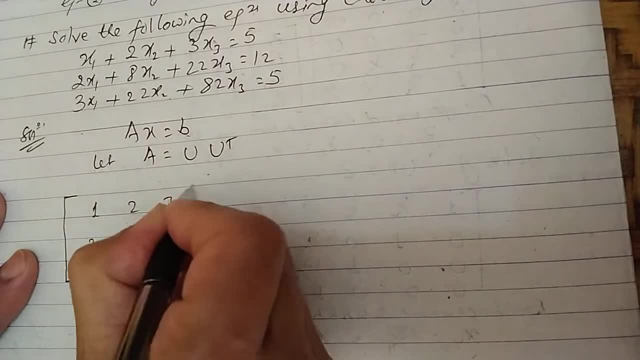 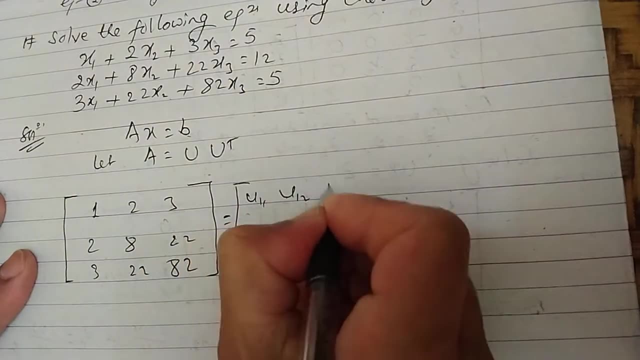 And what is 3,, 22,, 82?? Alright, So we will not take the diagonal element 1.. It is only a Taylorian decomposition, So U11., U12., U13.. 0.. U22.. 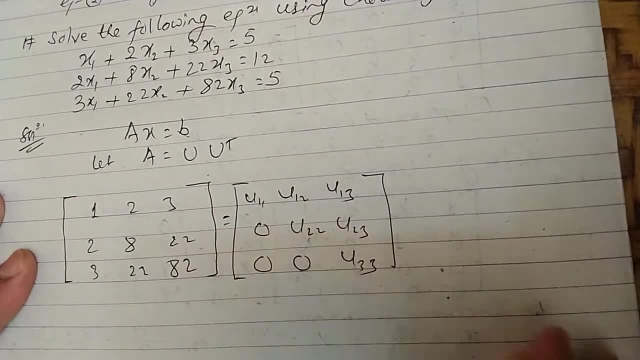 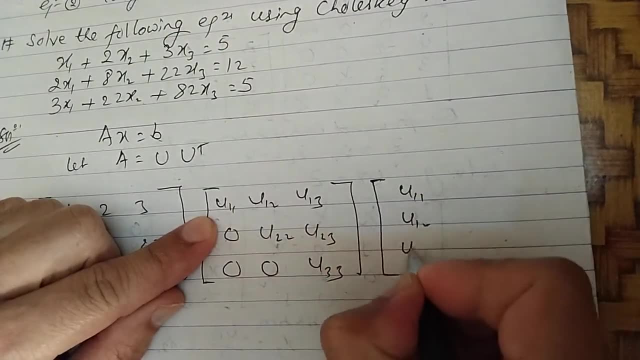 U23.. 00.. U33.. Alright, So this is the upper triangular matrix. Now what is the transpose of this? U11.. U12.. U13.. Write the row in the column. So another one: 0.. 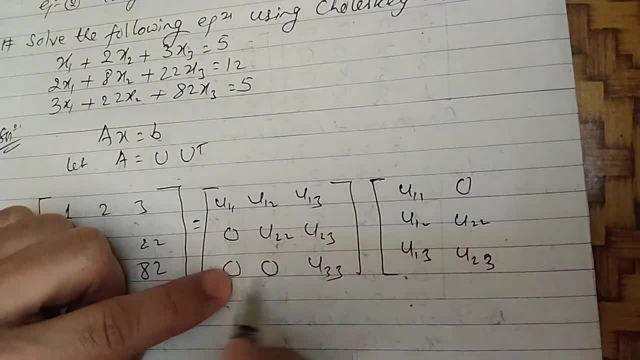 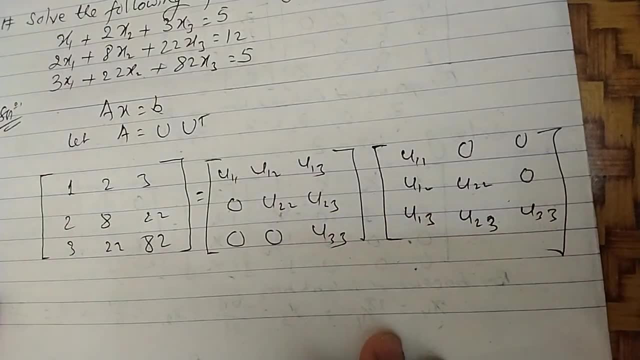 U22.. U23.. Alright, Another one, So 0. 0.. U33. 24. 0.. Where do you want it to be Words as well? You want it to be 4 in 4.. 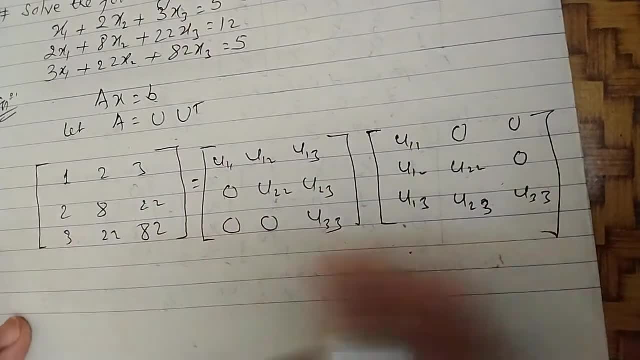 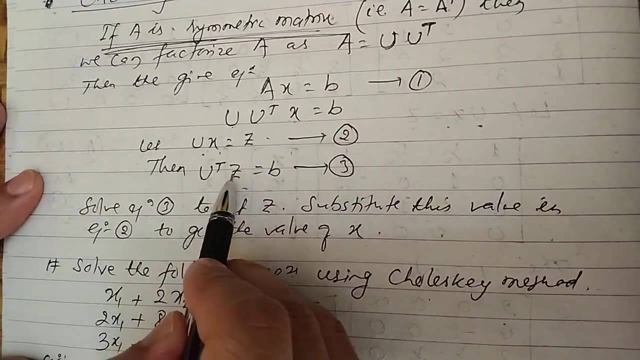 Not here. It should be here, right, Okay, Okay, Now, you are looking for this. Now, if U comes after, oh, Now, what is dunno? 1, 2., 2.. 1., 2y, 1.. 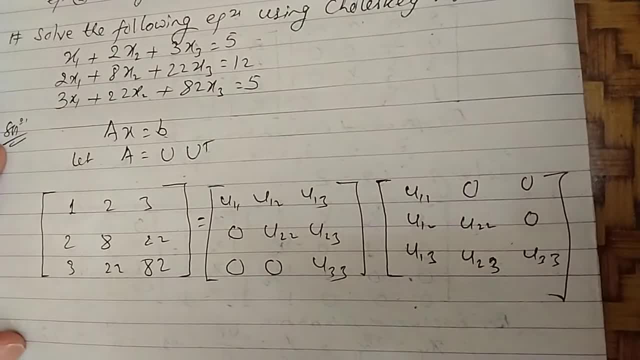 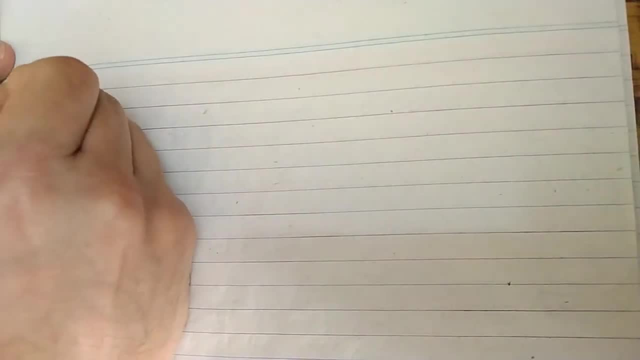 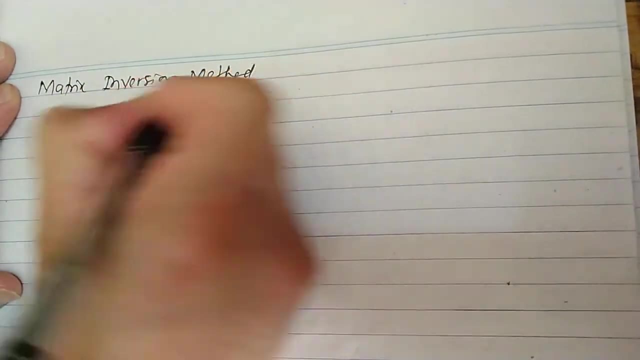 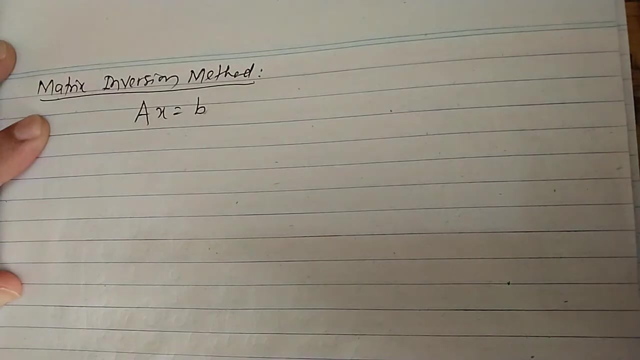 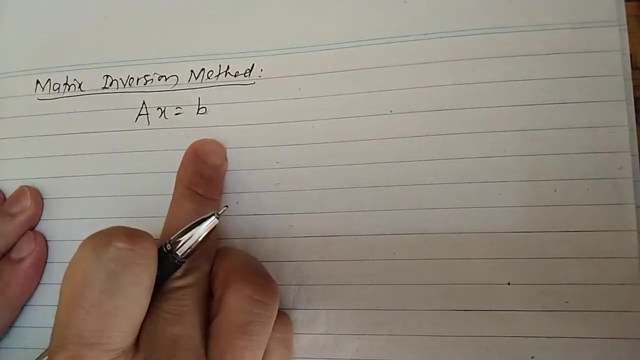 the solutions in the next day of the class. so let us study matrix inversion method. matrix inversion method: all right, it's very simple. so system of equation is given as what ax equals to b. all right, so if you multiply both side by a inverse, or if you try to solve for x, 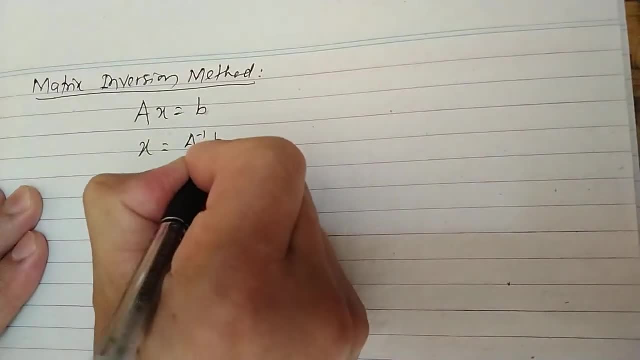 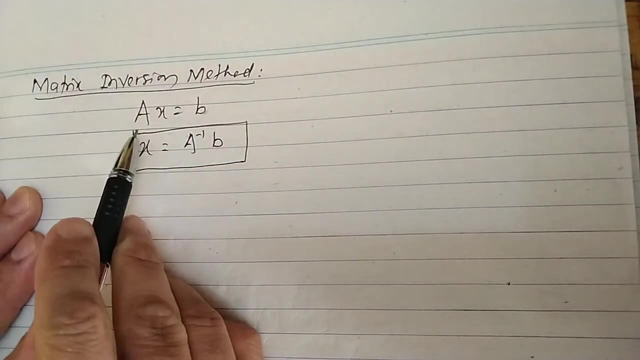 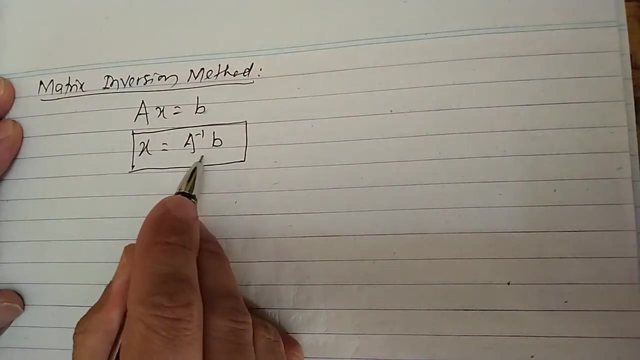 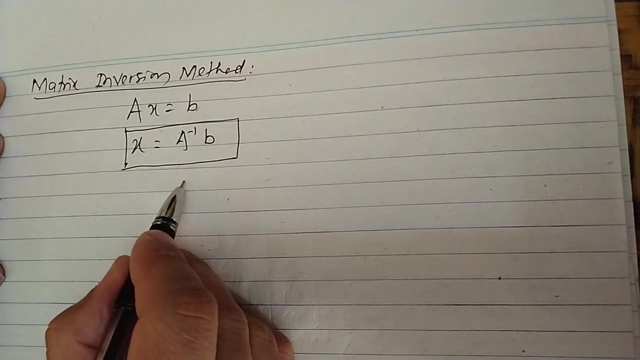 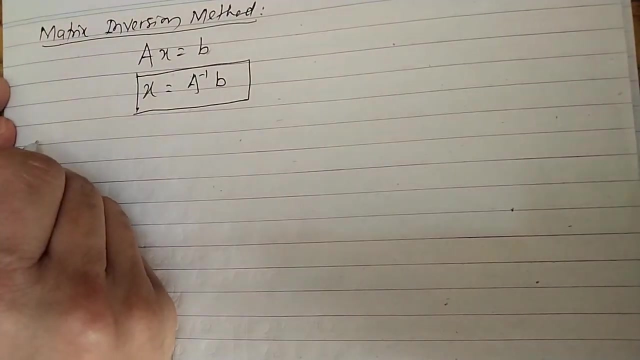 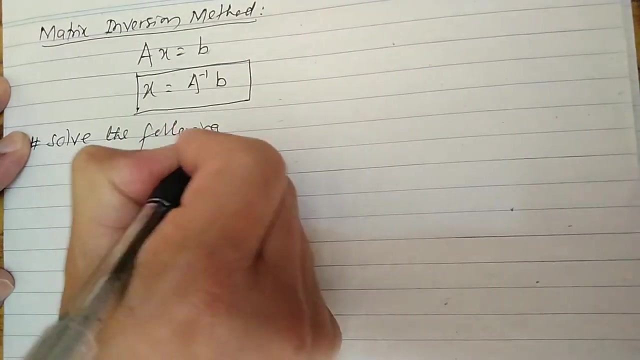 so x equals to a. inverse into b, you will get the value for the solution x. so inverse will be using gauss-jordan method here, and you can use the cofactor method, as you have studied in mathematics previously. okay, so let us try to solve a problem, solve the following system: 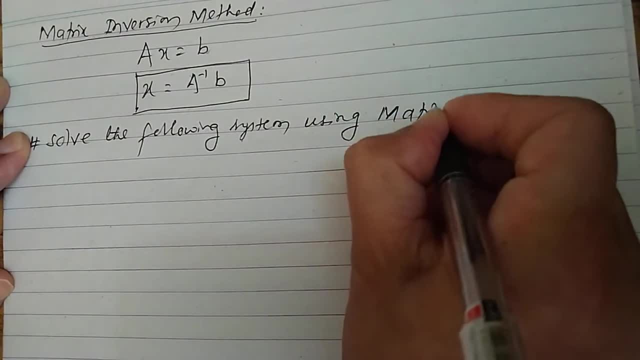 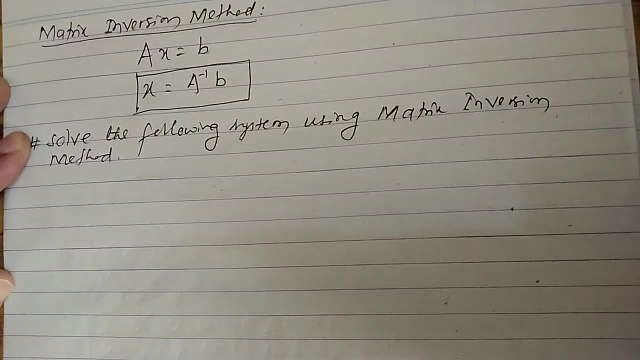 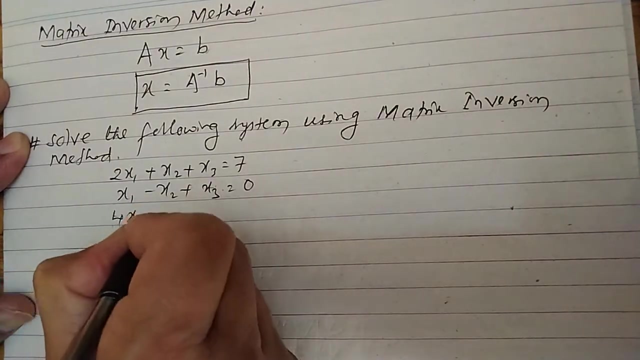 using matrix inversion method. so you have given an equation: 2x1 plus x2 plus x3 equals to 7, x1 minus x2 plus x3 equals to zero, and 4x1 plus 2x2 minus 3x3 equals to: 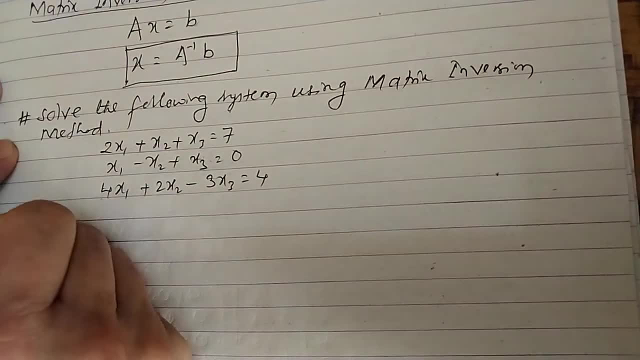 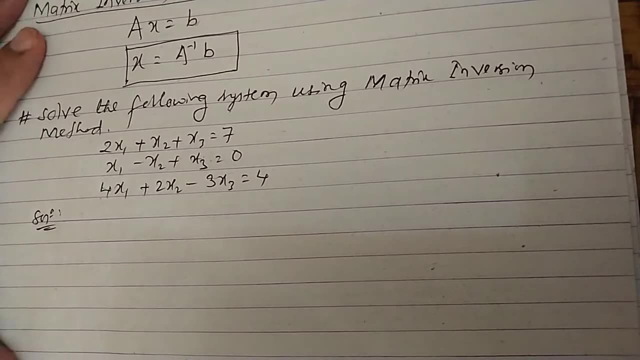 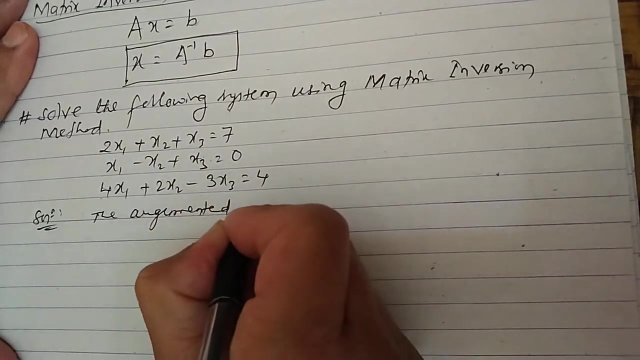 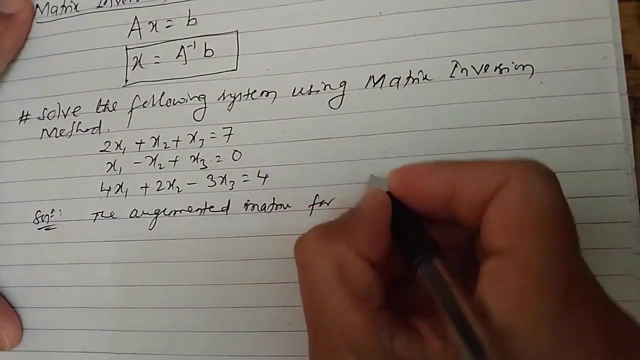 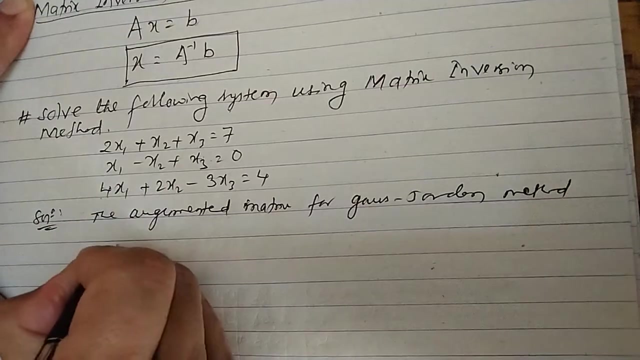 four. all right, I can solve the resolution, so i'll be using- they've got certain method to get the inverse metrics, so let us write down the argumented matrix, the augmented, the augmented matrix for gauss-jordan method. so What is the coefficient of this? 2, 1, the coefficient is this matrix 1, another 1, minus 1, 1, another 4, 2, minus 3.. 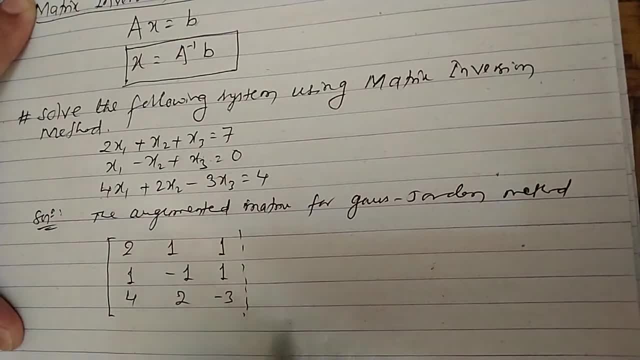 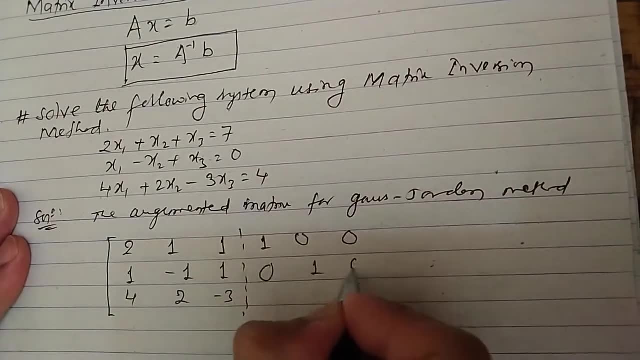 Alright. so what did we do in Gauss Jordan? We have studied previously. we have changed it to unit diagonal matrix 1, 0, 0, 0, 1, 0, 0, 0, 0, 1, so keep that unit diagonal matrix. the order is the order. 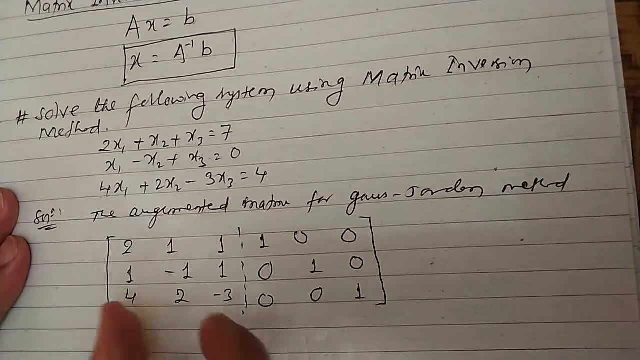 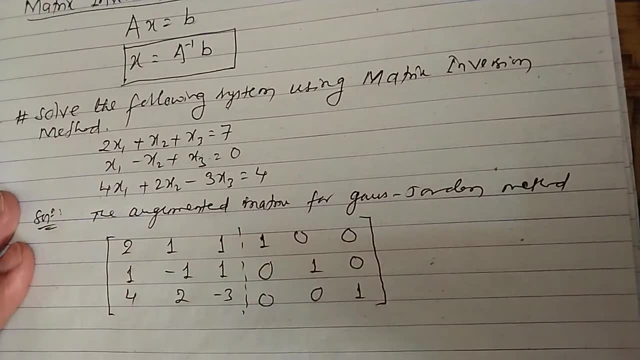 So A into unit diagonal matrix of the same order A and unit diagonal matrix of the same order. Now, after doing the row operation in this we will use Gauss Jordan. we change this matrix into this type. We will change this to unit diagonal matrix and do the same row operation here also. 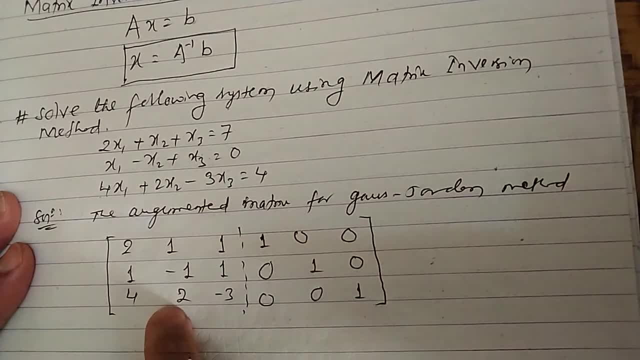 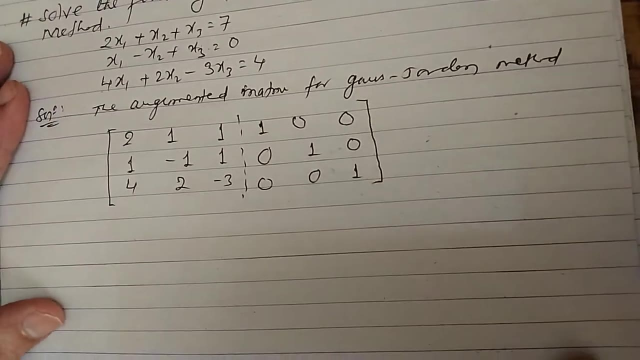 So when we change this to this, when we change this to unit diagonal matrix, the matrix here will finally be inverse. So this is known as the Gauss Jordan method for matrix inversion. You can use the cofactor method you like. Alright, so we have studied that. we are going. 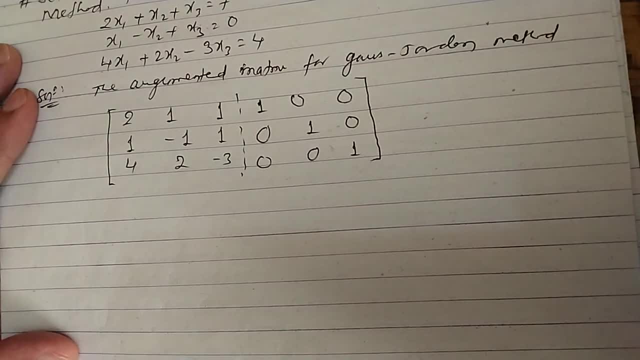 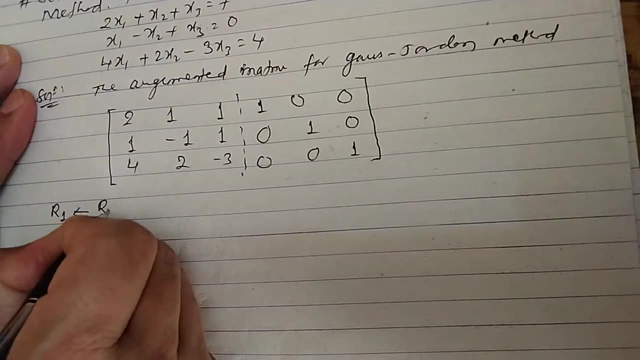 So now we have to do this from here also. So we have to make this unit diagonal matrix. so here is 2, we have to normalize it. So what we will do in R1, what operation we will do, We will do R1 by 2.. 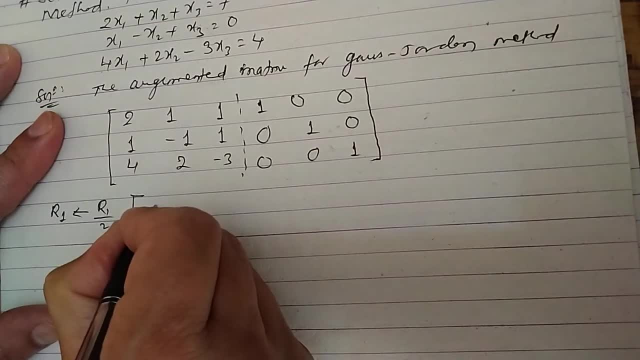 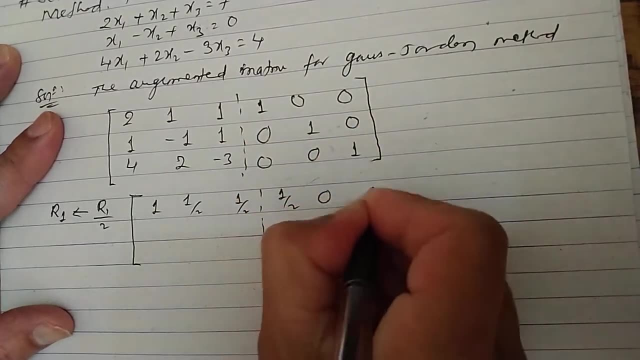 Why? Because we have to normalize it: 1, 1 by 2,, 1 by 2, we have to do the row operation here also. So how much is this? 1 by 2, 0, 0.. 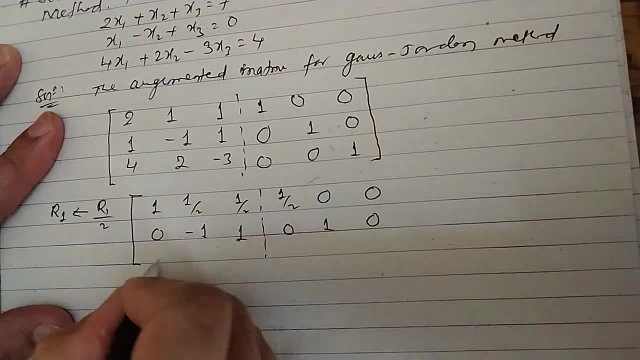 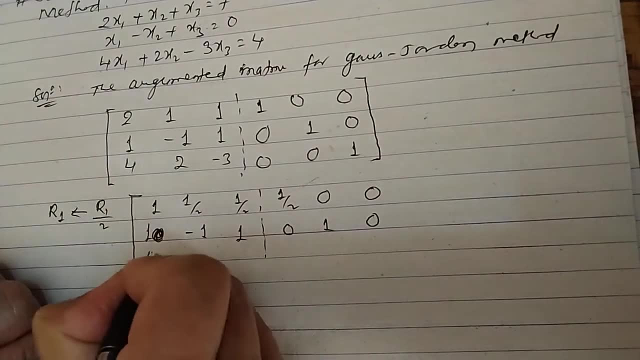 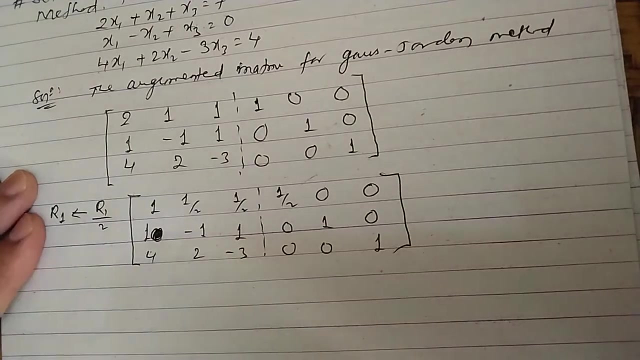 0, minus 1, 1, 0, 1, 0.. So sorry, this is 1.. So 4, 2, minus 3, 0, 0, 1.. Alright, 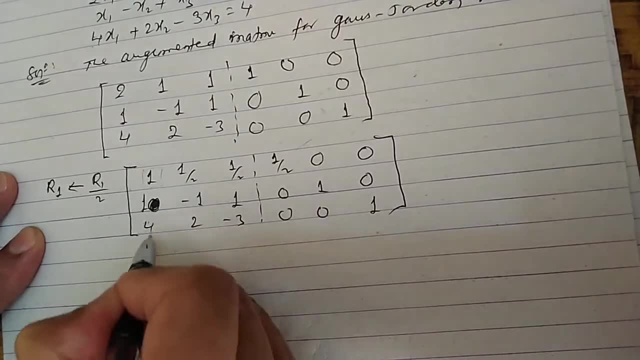 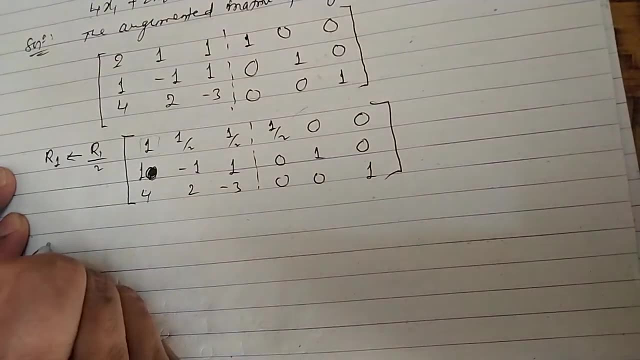 So, by using this row or this column A11, make this to 0.. As in Gauss elimination or Gauss Jordan, right. So we will do the operation in this. Which one will we do In R2.. What will we do? We will do R2 minus R1 and put it in R2.. 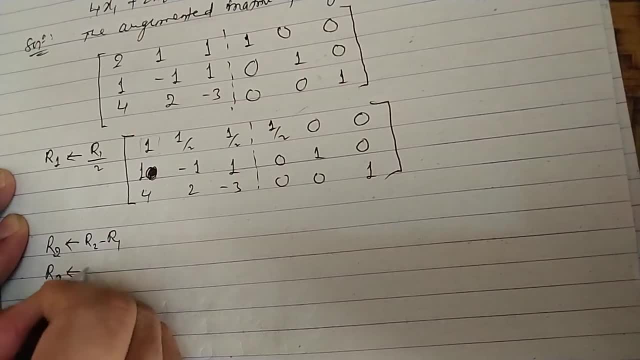 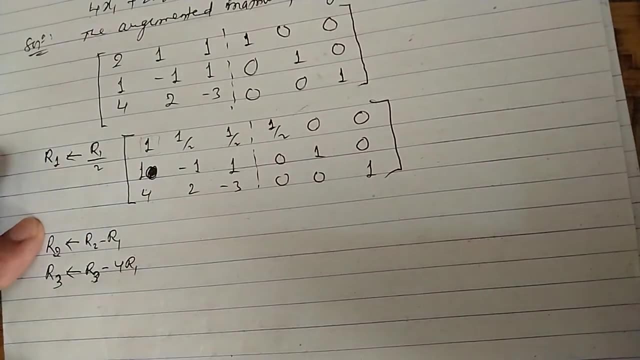 Oh, what will we do in the other? We will do the operation in R3.. What will we do? R3 minus 4 times R1.. Whatever is here, it is here also right. So 4 upon 1 will be 4, R1. 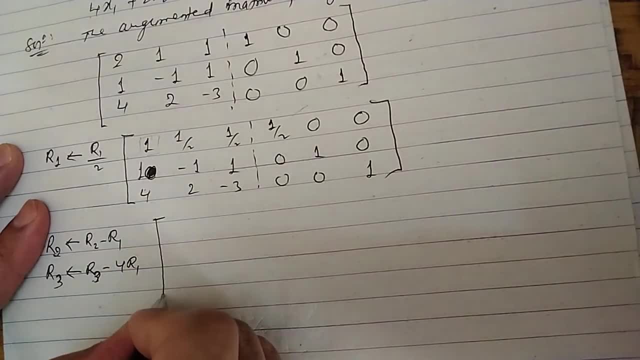 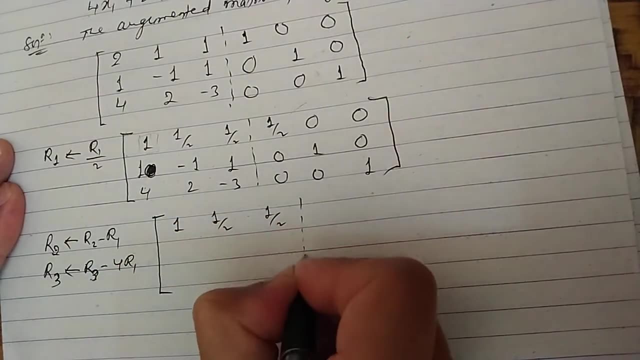 There is a positive sign here, so we have to do minus. So let's do these operations throughout. What will happen? 1. 1 by 2.. 1 by 2, unchanged, So 1 by 2, 0, 0.. 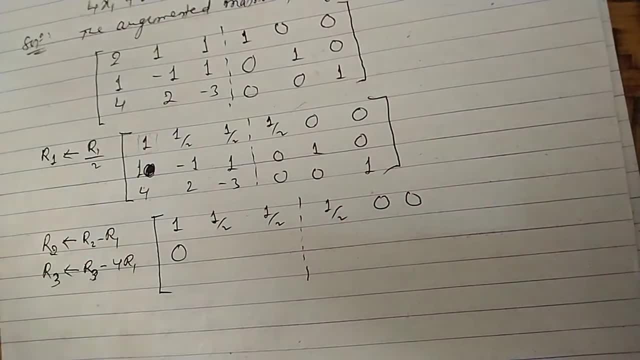 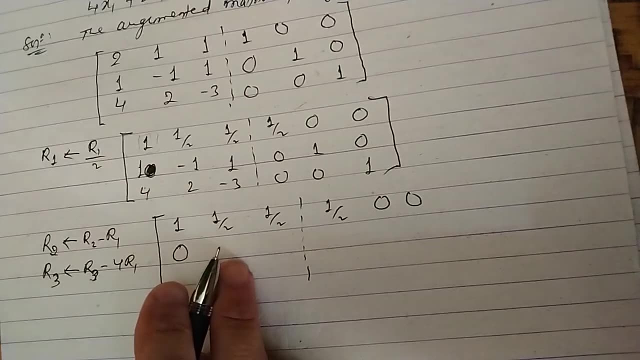 So we are making it 0.. So that will be 0. So what will happen in this? It will be 0, right? So after 0, what will happen? This will be minus 3 by 2.. 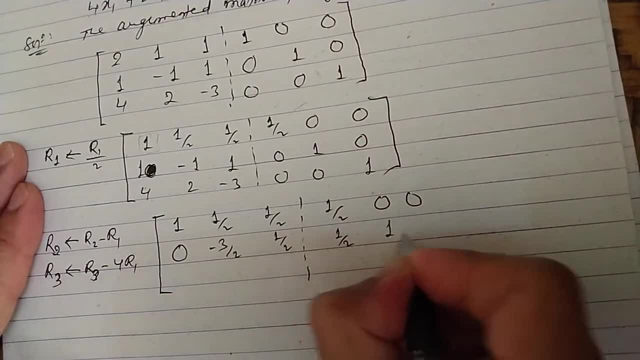 This will be 1 by 2.. 1 by 2.. This will be 1.. This will be 0.. We are doing 0.. This will be 0.. This will come 0 because in this it is half. 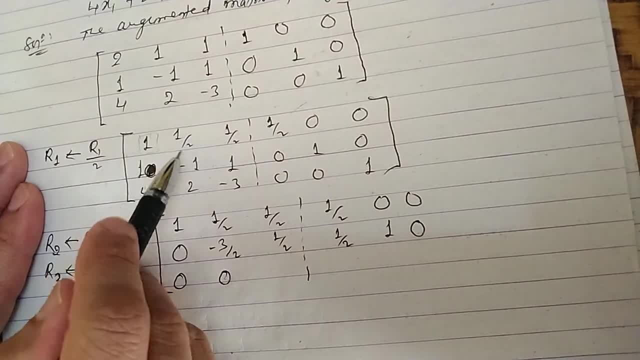 If we multiply half by 2, how much will it be? 1 will be. So here, when we multiply by 4, how much will be? 2 will be, And 2 minus 2 is 0.. 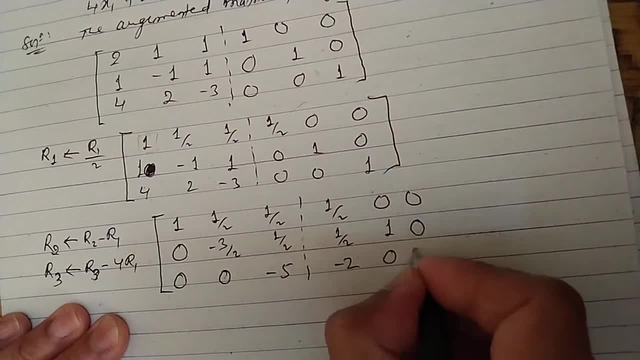 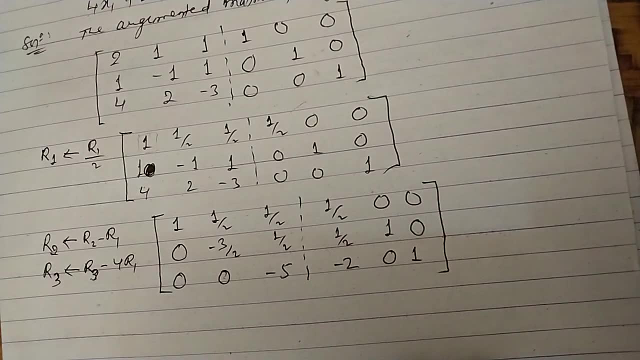 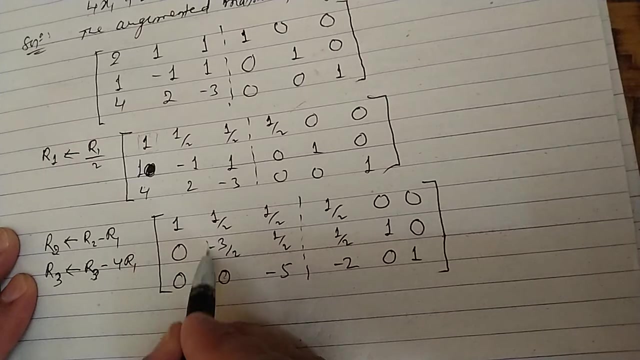 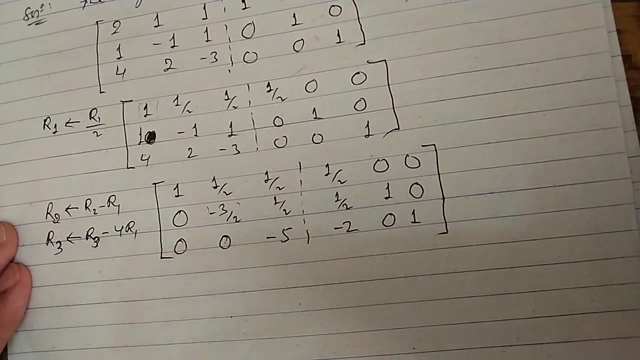 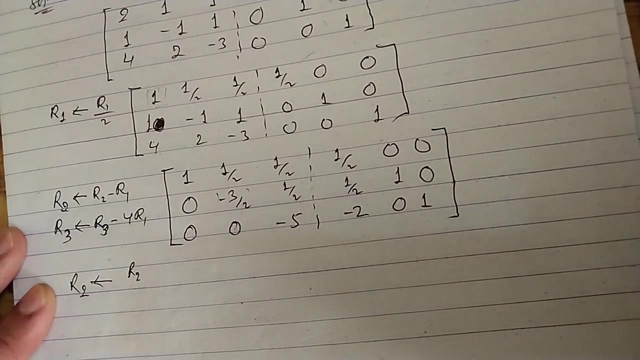 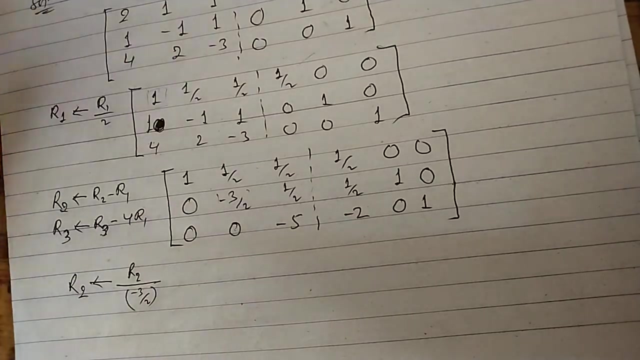 This is 0.. This is minus 5, this is minus 2.. This is 0 and this is 1.. So now, what do we have to do? we have to normalize this. So minus 3 by 2, what do we have to normalize? Minus 3 by 2, we have to divide it. So what do we have to do in row 2? So R2 divided by minus 3 by 2, or R2 into minus 3 by 2, as you like. So minus 3 by 2, we have to divide it. That means minus 2 by 3, we have to multiply it. So if we do this, 1, 1 by 2, 1 by 2.. 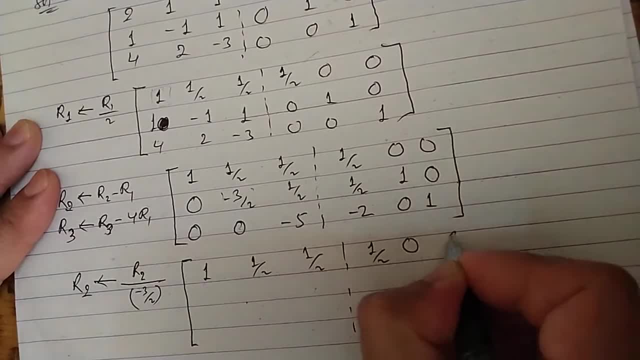 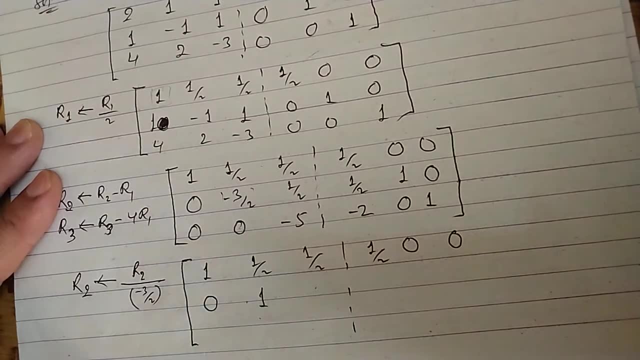 So 1 by 2, 0, 0, 0.. So what will this be Minus 1 will be. And if we divide this by minus 3 by 2, what will this be? 1 minus 1 by 3 will be. So what will this be? 1 by 3 will be. 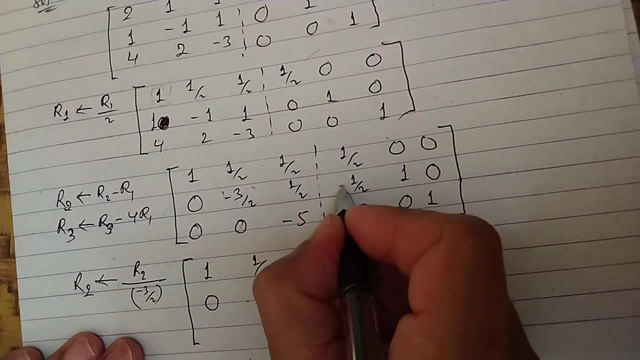 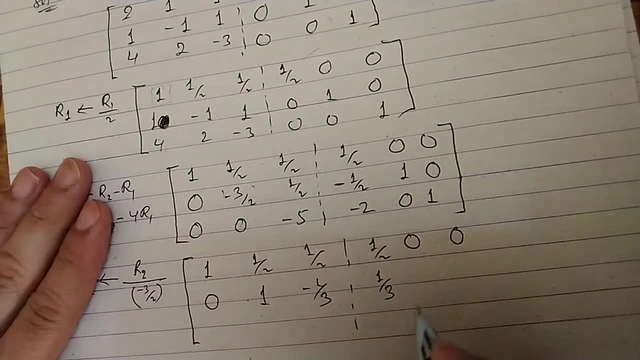 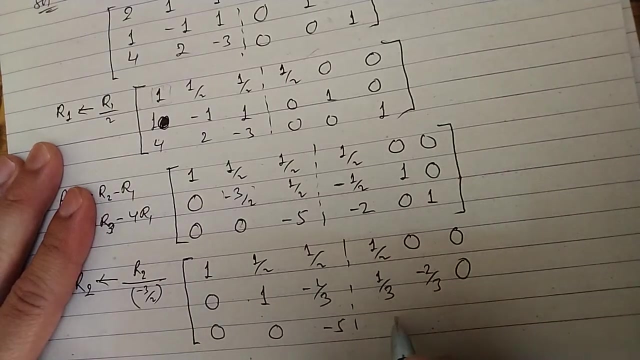 Here: minus 1 by 2 is there. Sorry Here, look at this. Here: minus 1 by 2 is there, Right? So 1 by 3 is there And minus 2 by 3 is there, And 0 is there And 0, 0, minus 5.. So minus 2, 0, 1 is there. 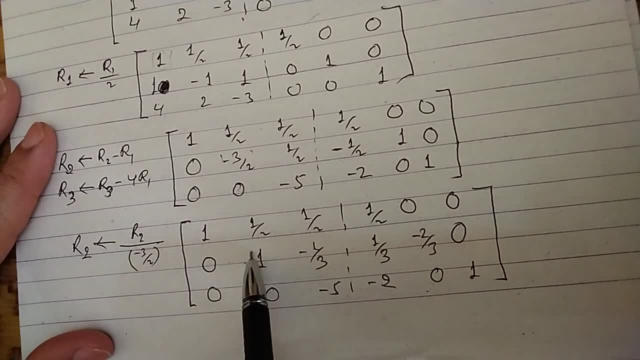 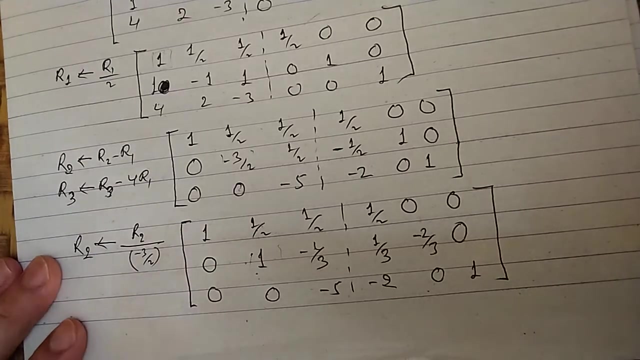 Okay, So now, using this right, you use this. What do you do? You change, Make these two 0.. 1 use here And you get 0.. So what other operations you do? Right, So normalize this. 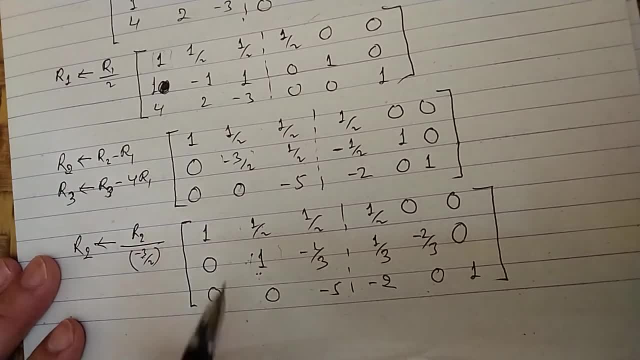 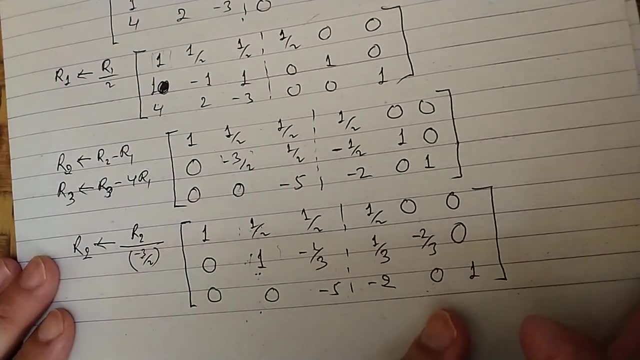 Normalize this And we do, And you get 0.. So you do operations in row 1.. This is already 0.. So it will do operations in R3.. Right, So you have to do this. So what have you done in R1?? 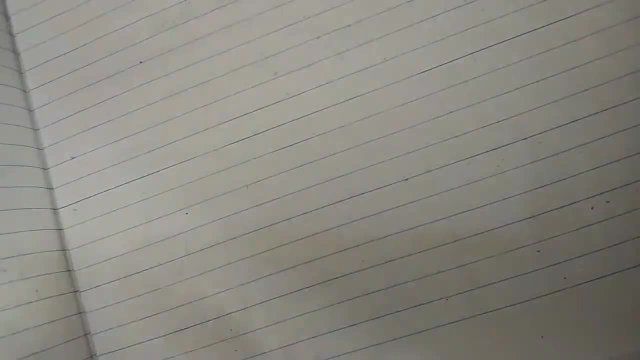 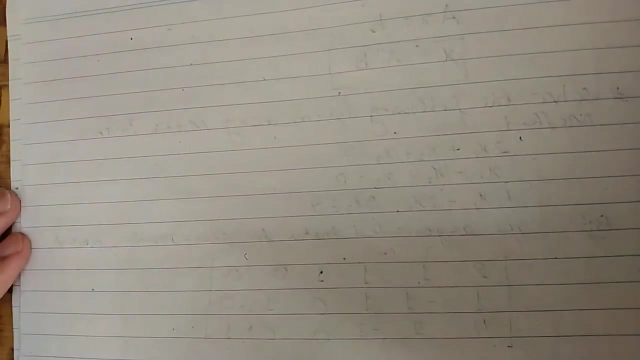 so r1 minus half r2. right, then you do the row operations.